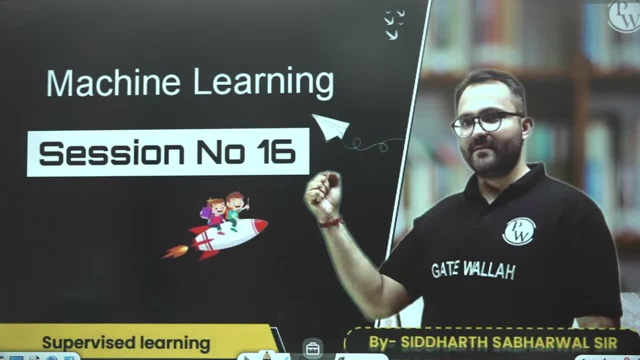 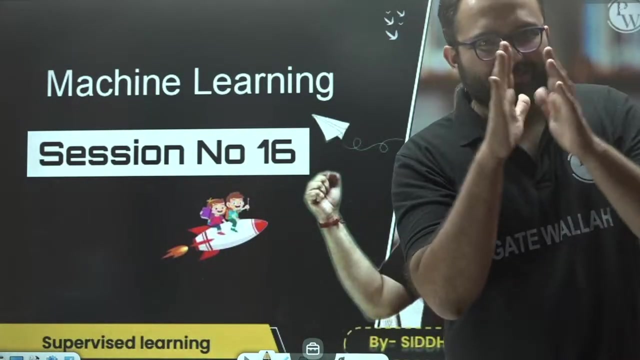 Thank you, Thank you, Thank you, Hello Namaskar friends, Good evening. everyone. Welcome to our channel And tell us quickly who are the kids who have come and we will move forward with full power, full energy. Today we will discuss decision trees. 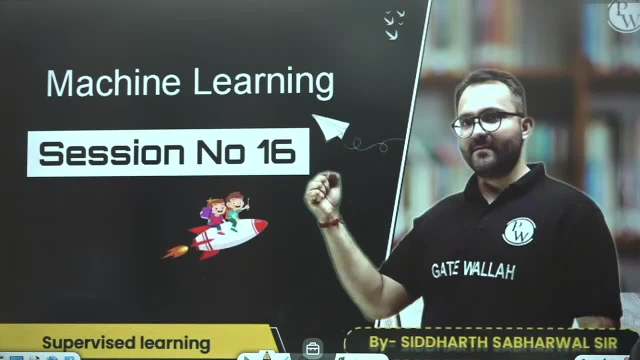 But first of all, the first thing we read yesterday. friends, let's revise it and move forward. Let me start my chart. So whose kids are clear about yesterday's story? Tell us in the comment box. quickly Mark your presence. 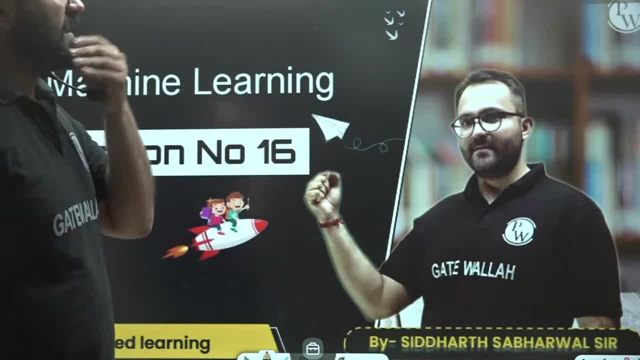 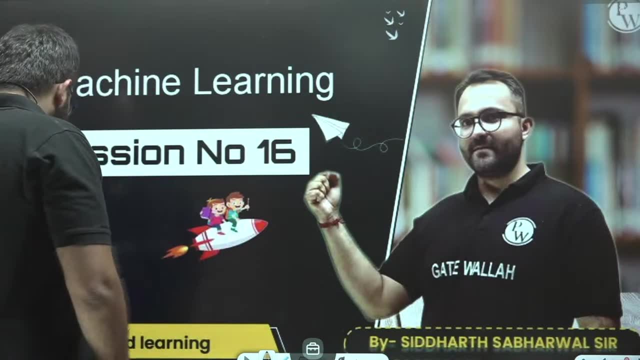 And we will move forward with full energy, full power. Let's start, friends. Put your presence quickly. Mark your presence in the comment box. So, friends, in yesterday's class we had almost finished the KNNs. There are only questions left. 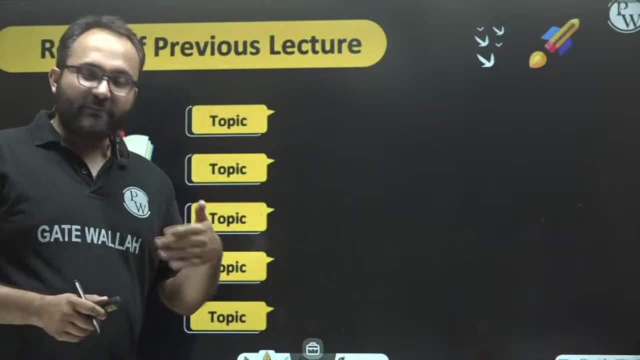 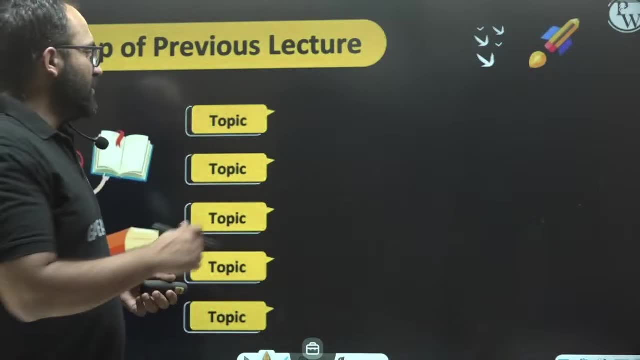 So I will ask you to do the questions today. Whatever we had read yesterday, we will revise it in the KNNs quickly And we are going to do some questions Like: let's see the cross-validation once And let's move forward. 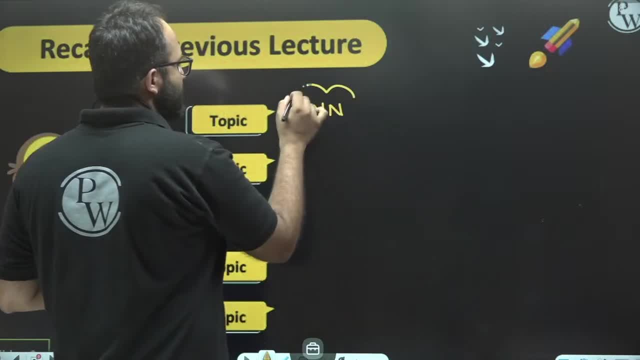 So in yesterday's class friends, we had read KNNs. Then we saw that to find K best, we have to do this, So we have to do this, So we have to do this, So we have to do this. 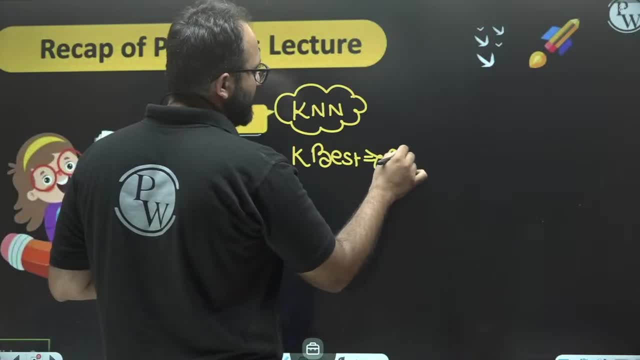 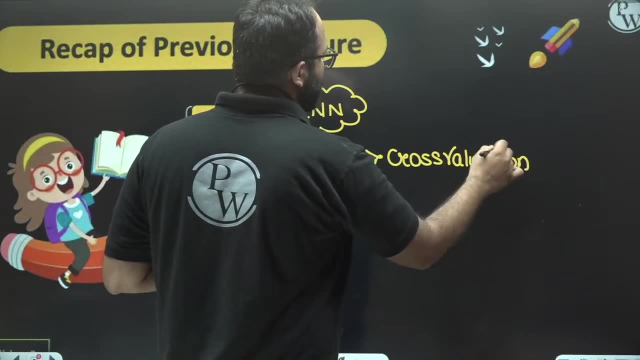 K is a hyperparameter, So to find the best value, there is a method That is called cross-validation. Okay, After that, we had seen two methods of cross-validation. One was K-fold cross-validation, And I told you that there is no relation between this and this. 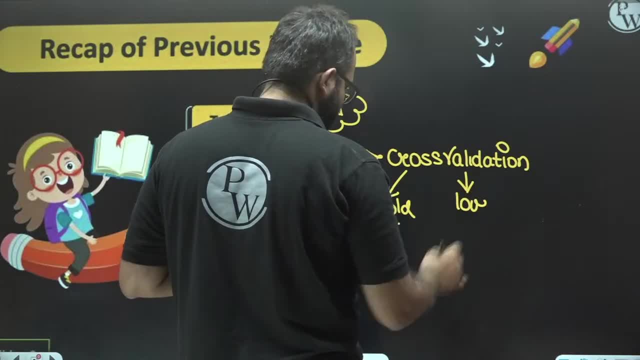 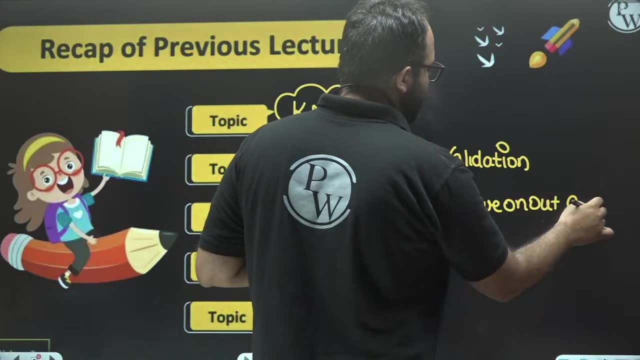 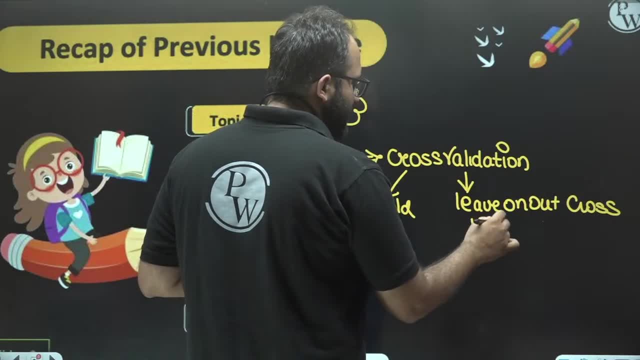 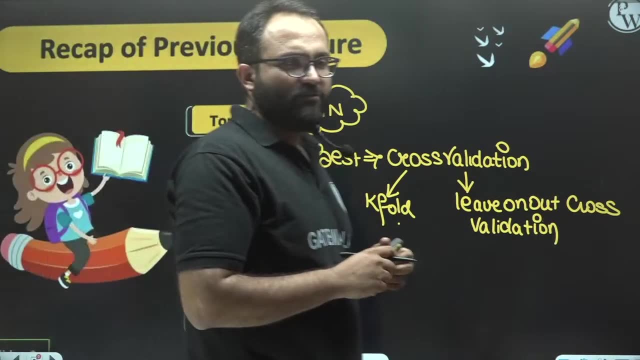 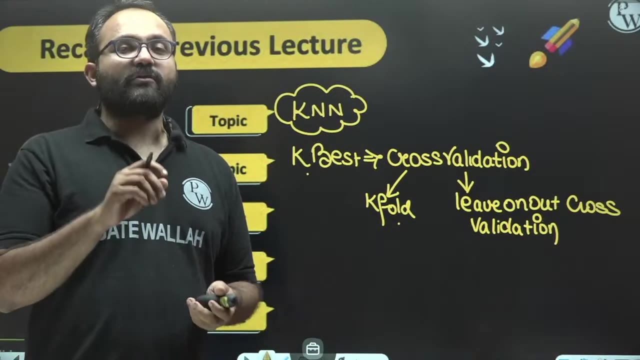 we are going to see this too. both of them will revise quickly after that, friends. we have seen one more concept that generally the value of y, which we were predicting, we were directly averaging it, but yesterday we have seen 2-3 questions where we have put a weight vector. 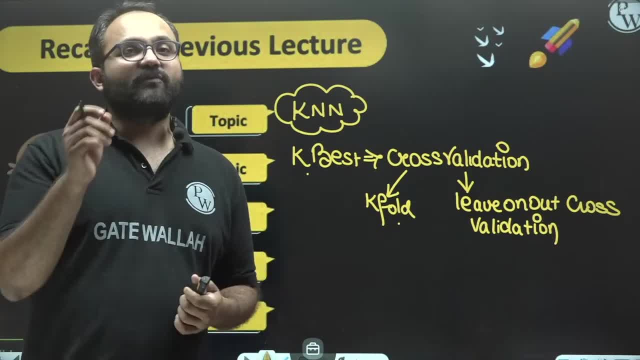 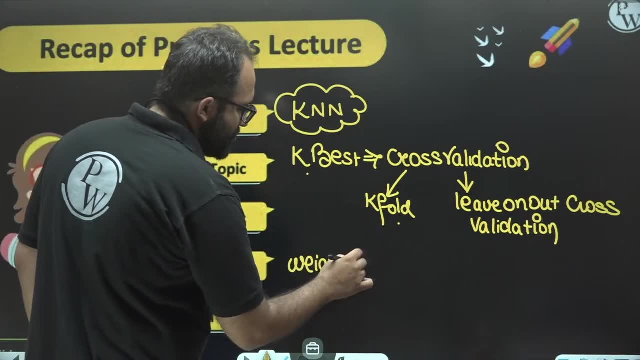 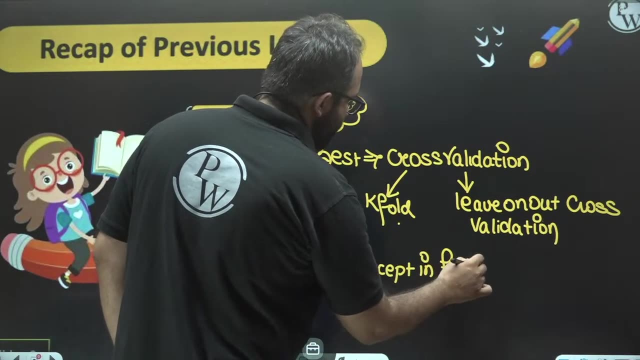 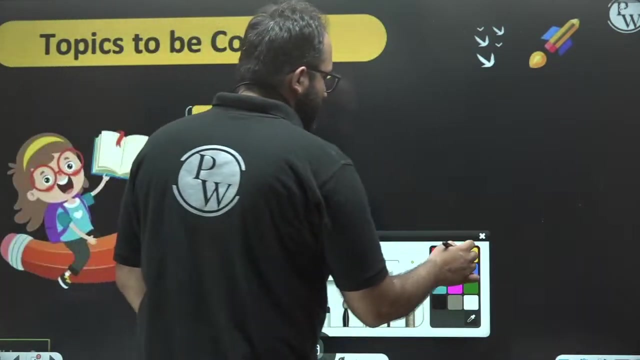 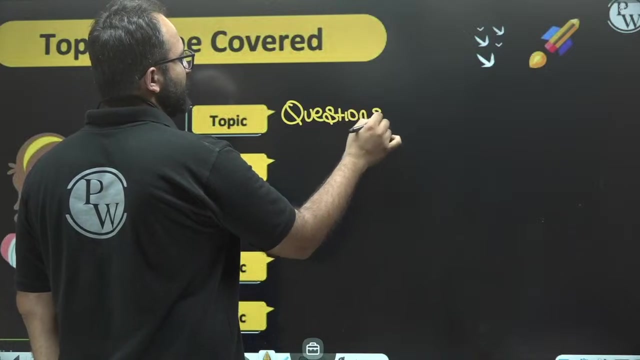 or a weight also, that was actually inverse of the distance. so we have seen a weight concept. ok, now if we see here what we are going to do in today's class, first we are going to do some questions. in last class we left some questions. and second thing, we will start today. 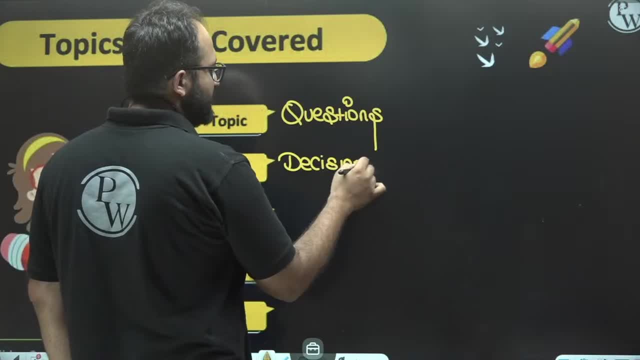 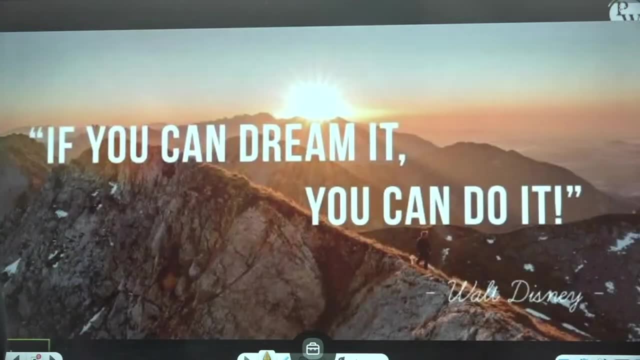 decision tree. ok, this is also a non parametric, unstable algorithm. we will try to understand it. so we start with a very beautiful quote: the fitful power that is: if you can dream it, you can do it. if you can think about someone, then you can achieve it easily. 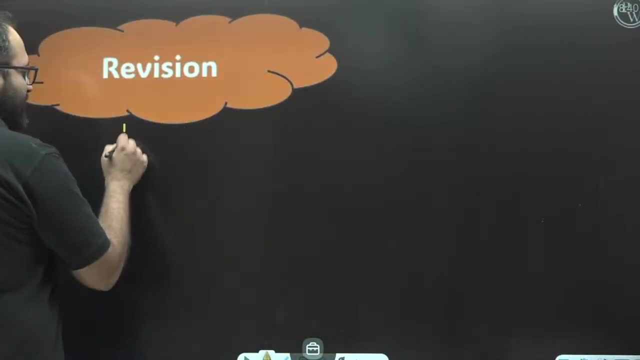 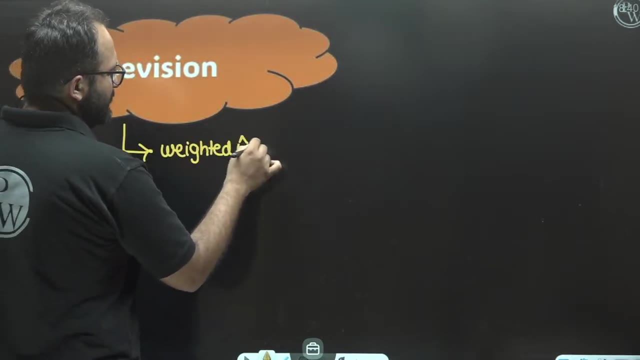 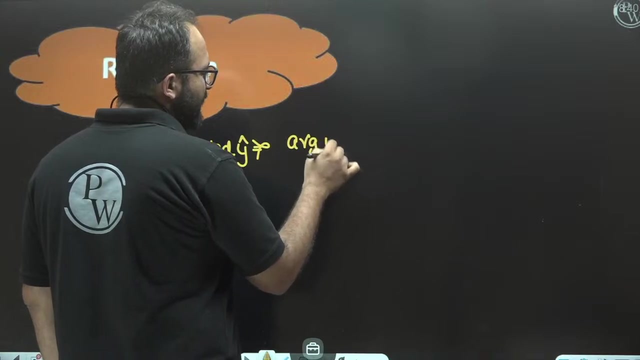 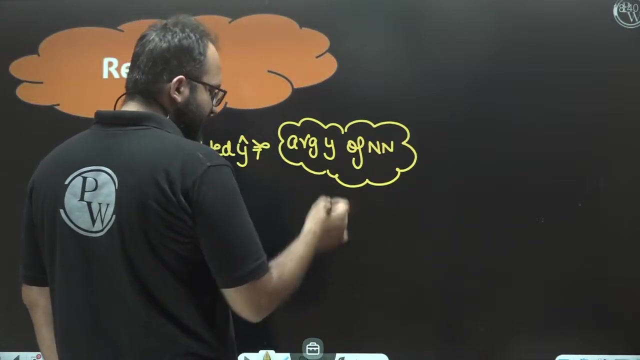 so let's revise quickly, friends. first of all we will see weighted y hat. so weighted y hat is very simple. in this we have seen first, generally, we were taking the average of y, which was our nearest neighbor, y of the nearest neighbors, or k nearest neighbors. that would be better. 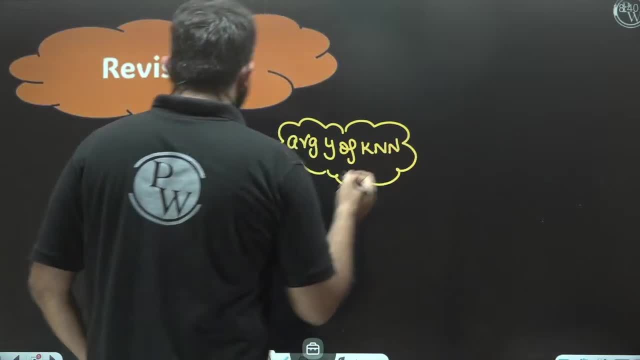 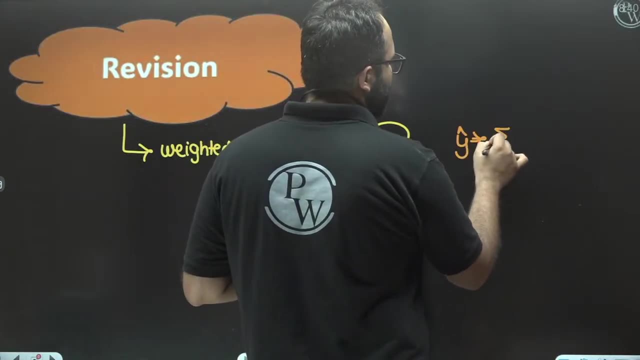 of the k nearest neighbors. ok, and here what we will do, friends, but in the weighted case we have to calculate the weight of all, for all the nearest neighbors. we have to calculate the weight of all. now, how will we calculate the weight? the question we saw yesterday. 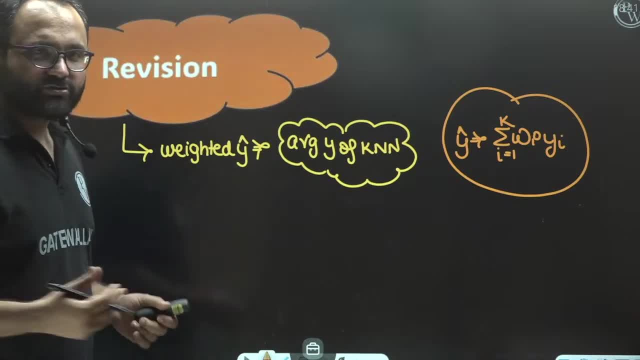 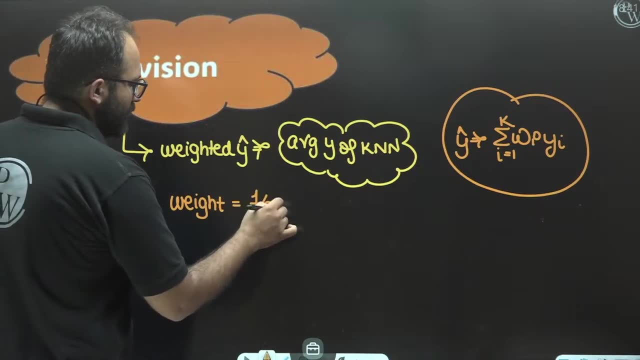 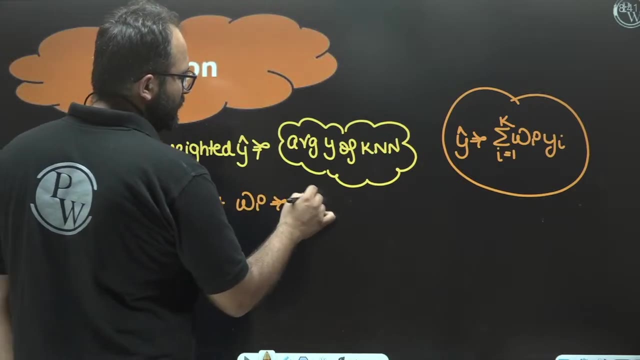 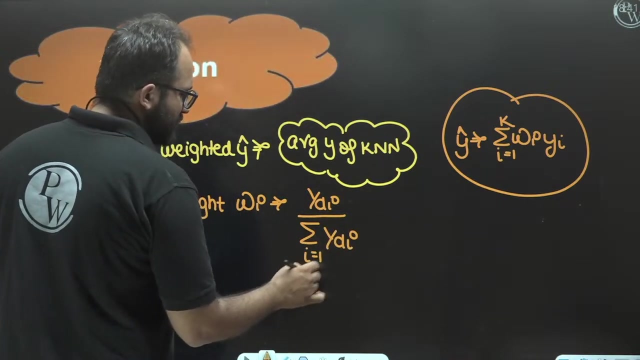 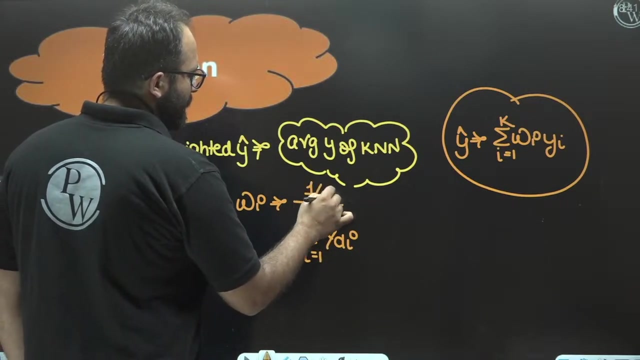 we saw that the weight was inversely proportional to the distance. so weight of ith point is equal to the distance of ith point. divided by sum of distance of the points i is equal to 1 to k. right, this is how we were doing, ok, so i hope. 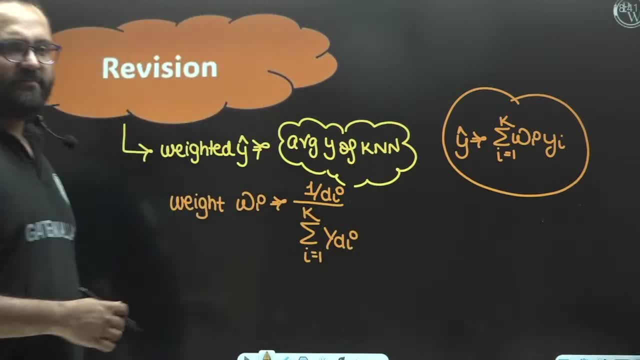 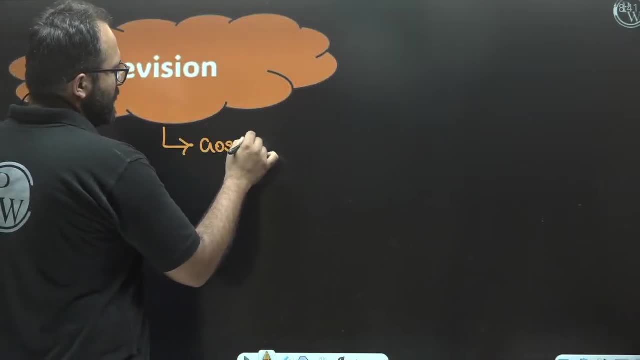 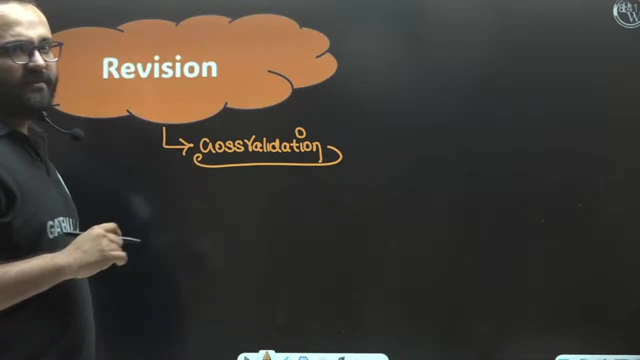 you are able to understand this, and we have seen this in yesterday's class. next, friends, we have seen a cross validation. why cross validation is done. i have told you that if we are giving training and then testing, then we will be able to find the k value. 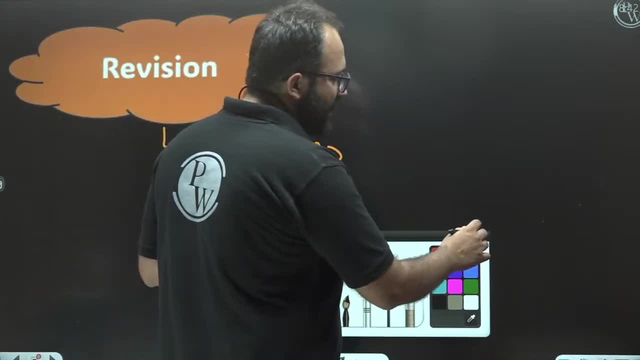 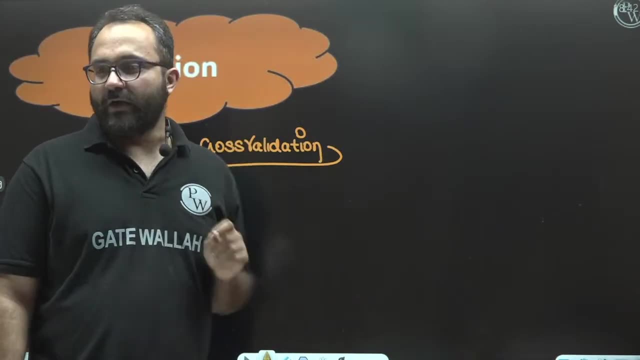 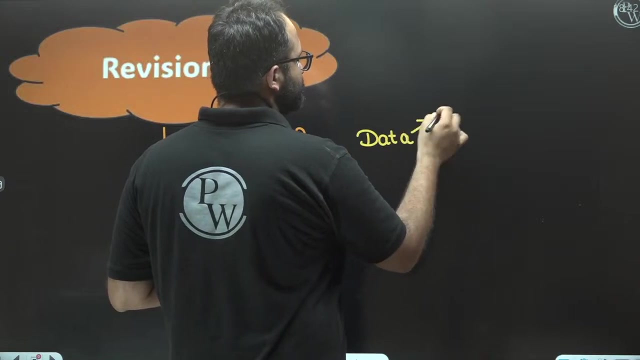 so there was a problem that whatever we find during testing, it will be best for 10 to 20% data. it will not be best for overall data. it will not be generalised. so what is better is cross validation. what we do in cross validation, whatever data we have. 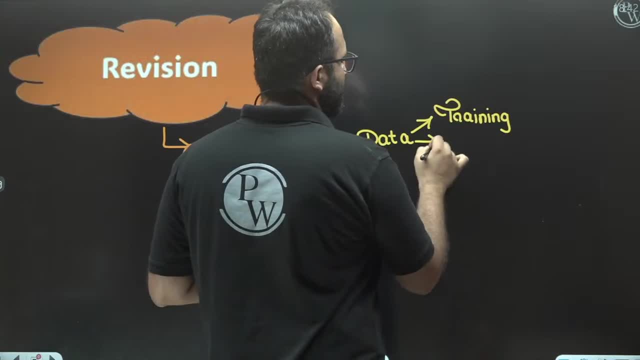 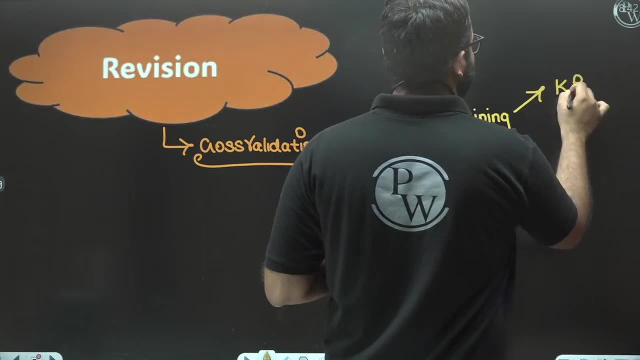 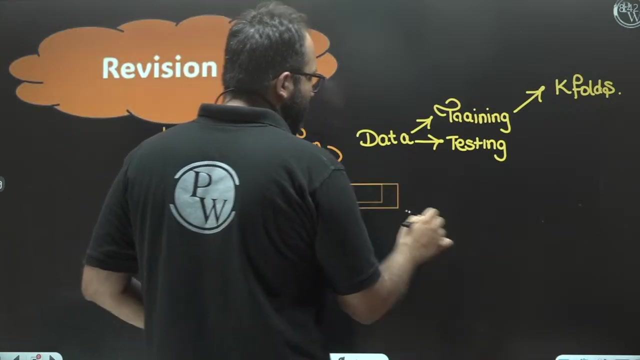 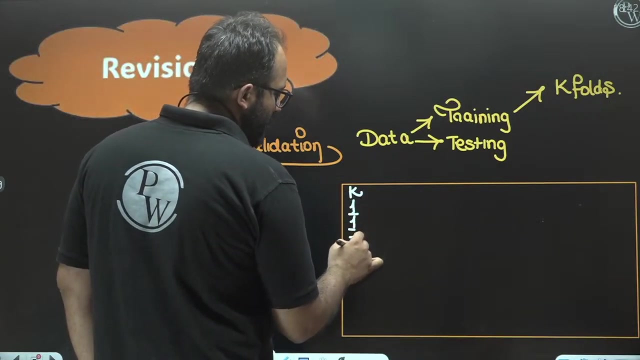 we break it in training and testing and after that we break training data in k folds. after that i had told you that in yesterday's class we made a table, created a table, that first you keep k value as 1 and in k folds training on one fold. 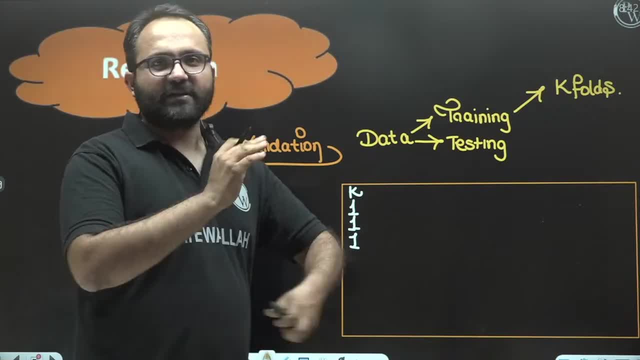 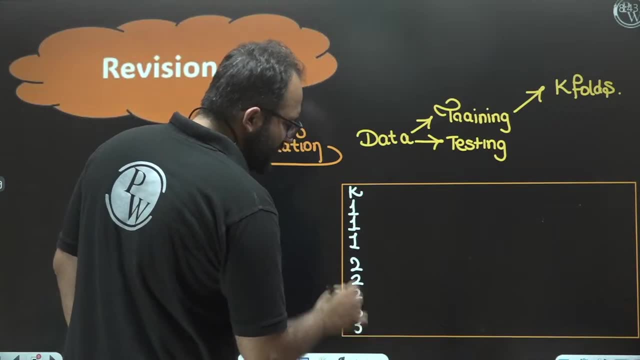 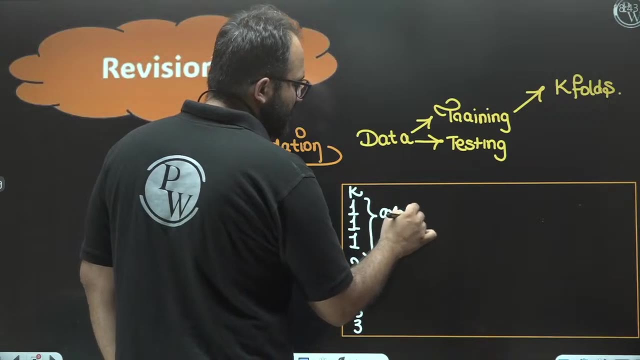 or validation on one fold and training on other fold. do this and repeat: similarly, do k equal to 2, similarly, do k equal to 3, and so on. so now find out the average accuracy for this, because we want to see what is best for training data. 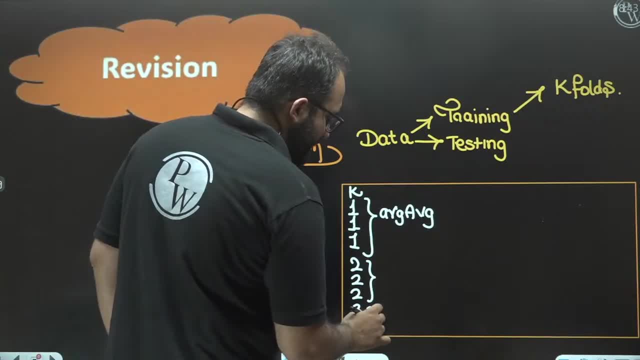 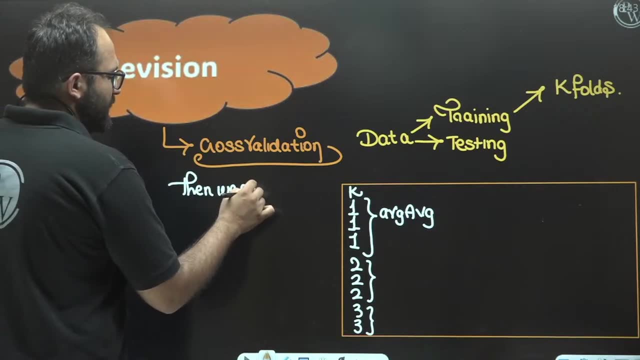 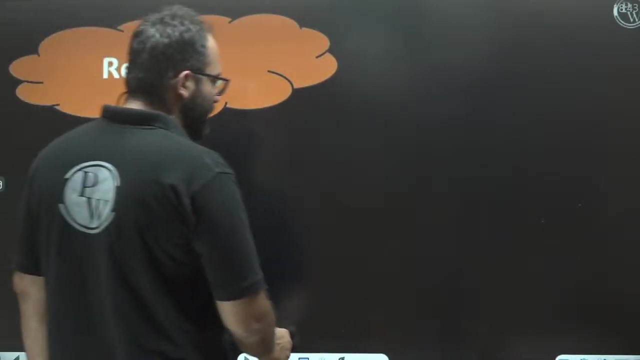 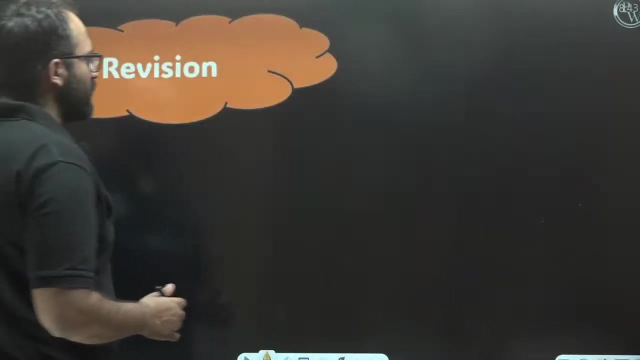 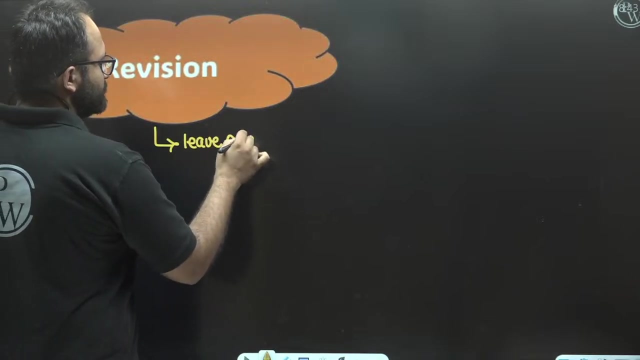 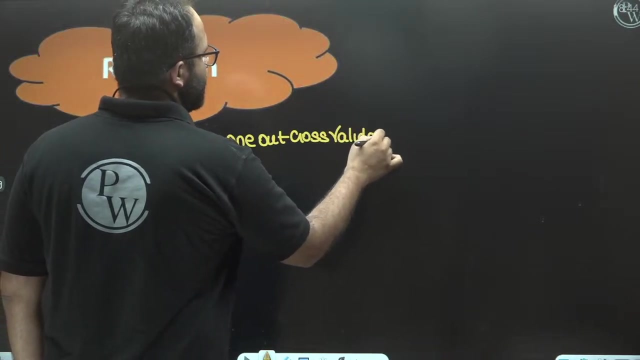 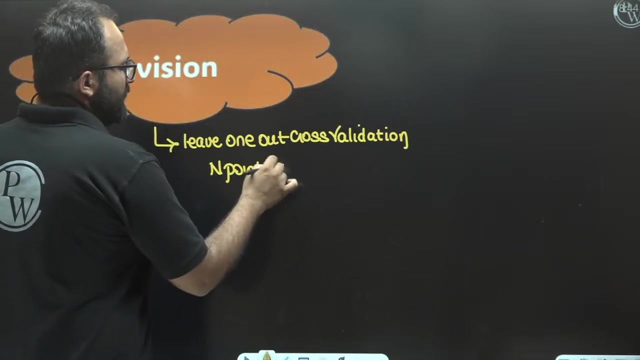 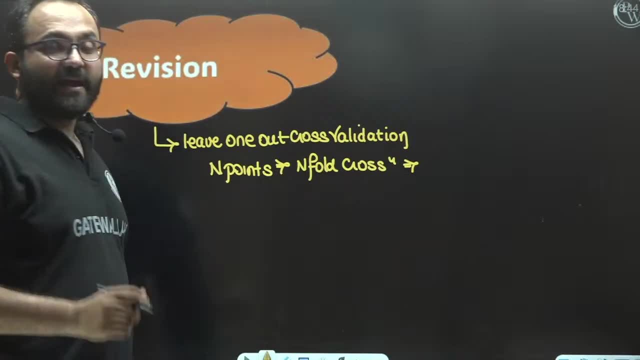 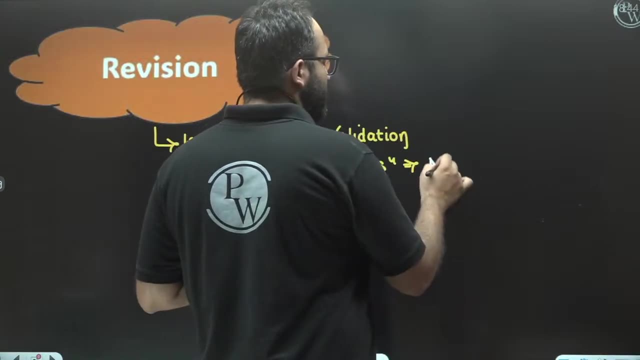 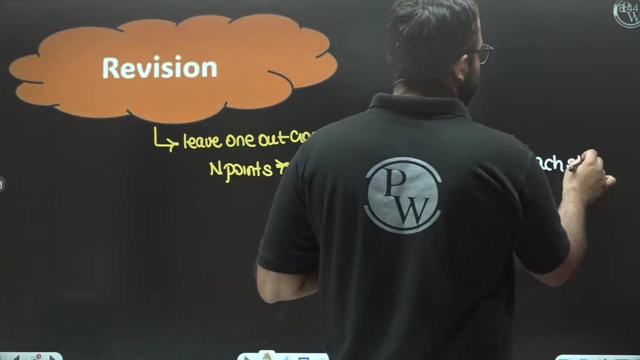 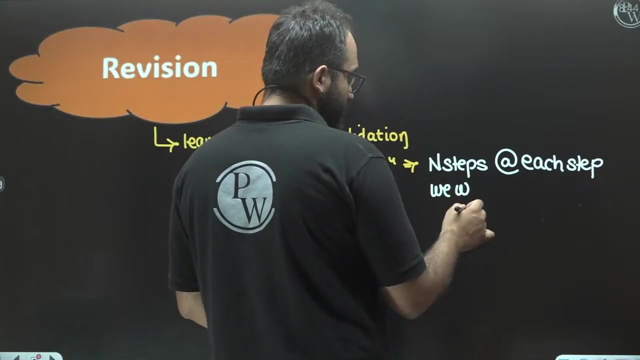 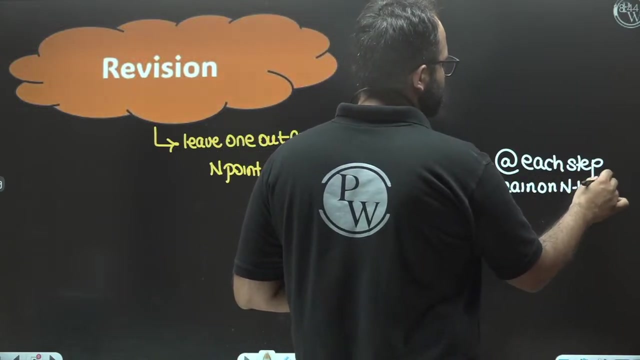 Where we will make n folds or n blocks, and each block will have only one data. So here we will have to do n steps, Or at each step. At each step we want, or we will train on n-1 data And validate or test on the one data point. 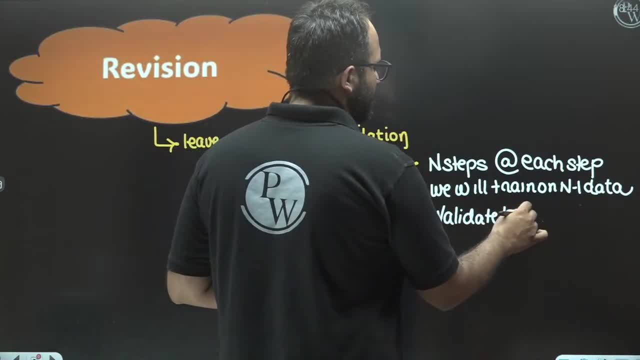 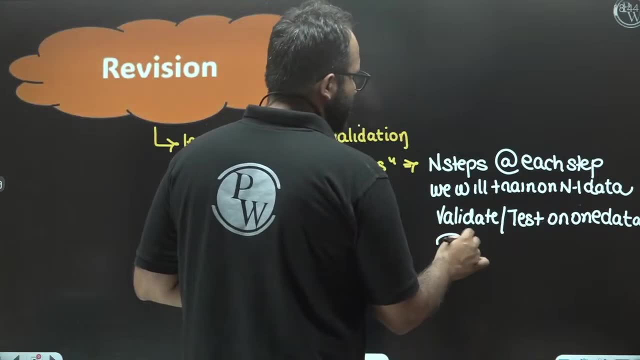 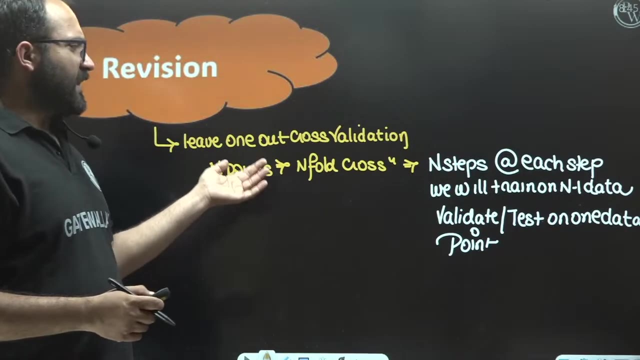 Take a validate or test on one data point. Take a validate or test on one data point. Take a validate or test on one data point. This is our whole story. It is same as k-fold cross validation, Where we were taking k-fold but now we will take n-fold. 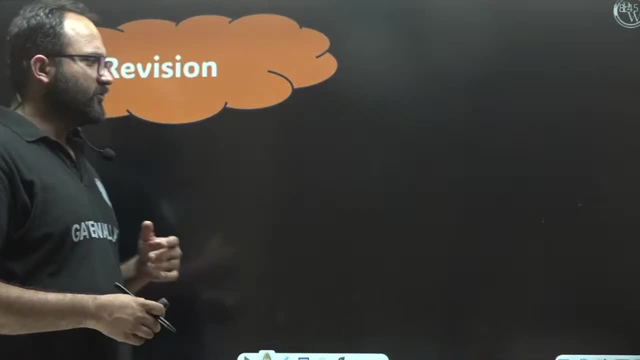 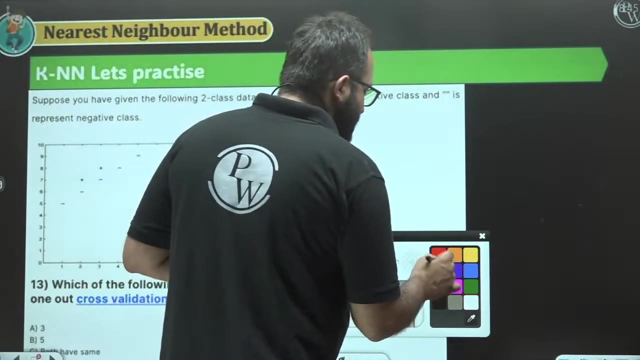 So this is how the story will be made. I hope you all understand this. So we have seen all the things in yesterday's class. Today we have a question. I hope this type of question can come in your paper. It is a very logical and good question. So we have given these points. 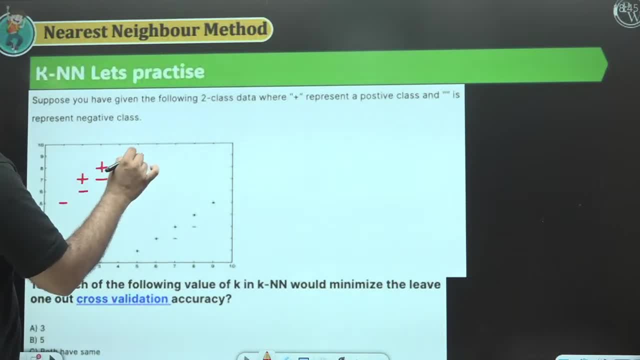 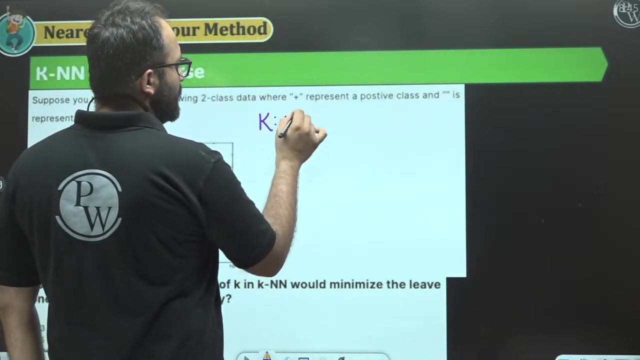 So we have given these points. Now here it is saying Which one of the following value of k in KNN would minimize the leave-one-out cross validation accuracy. So which value of k, Which one of the following value of k in KNN would minimize the leave-one-out cross validation accuracy? 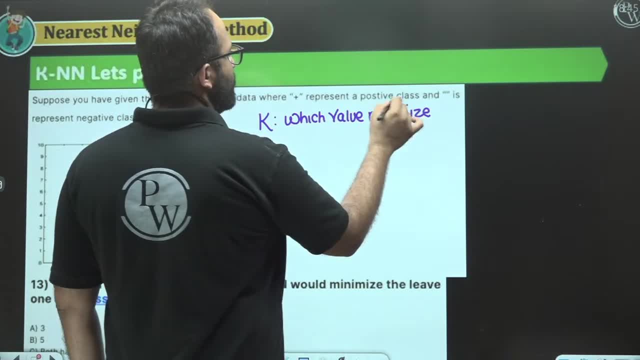 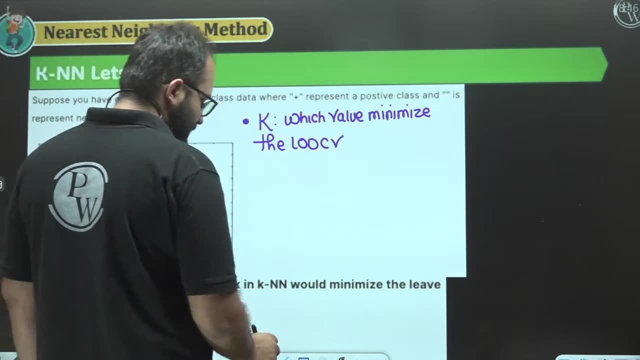 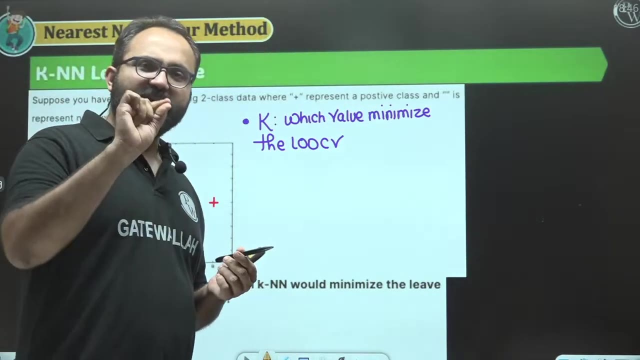 Which one of the following value of k in KNN would minimize the leave-one-out cross validation accuracy. So now what we will do in leave-one-out cross validation: We will do training on the overall data. We will leave only one point And then we will do testing or validation by keeping that point. 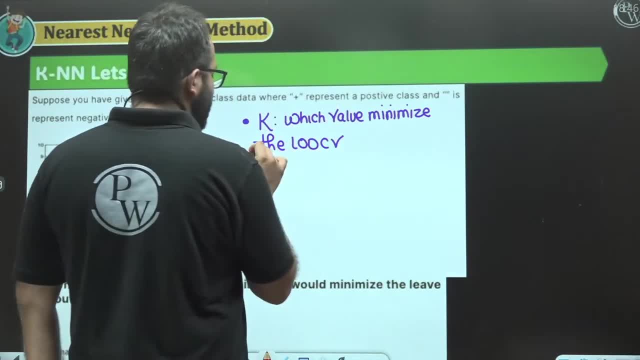 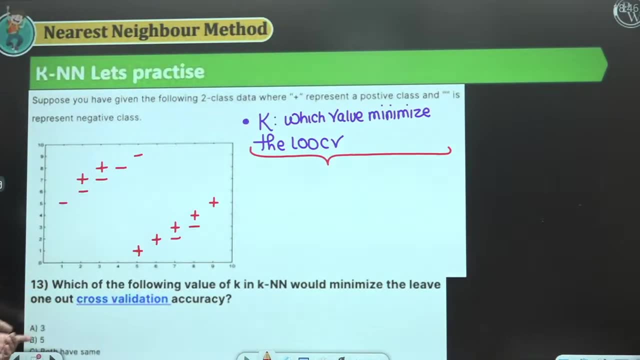 So let's quickly think about this, friends. Now here you can see. there are two options: k equal to 3, k equal to 5. Both have the same or none of these. So let's take k equal to 3 and k equal to 5. 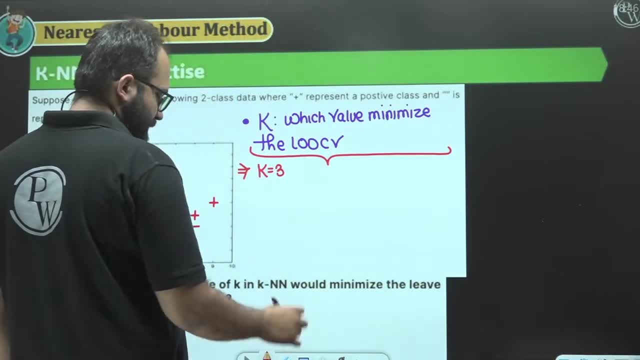 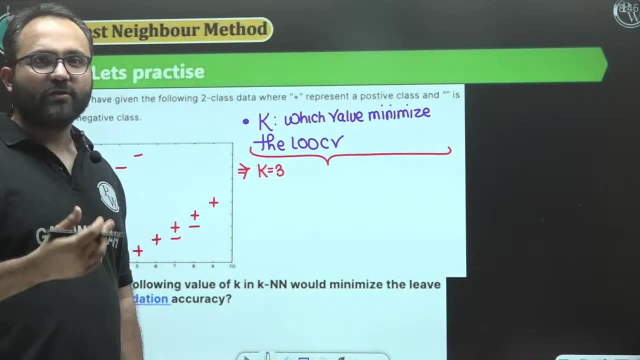 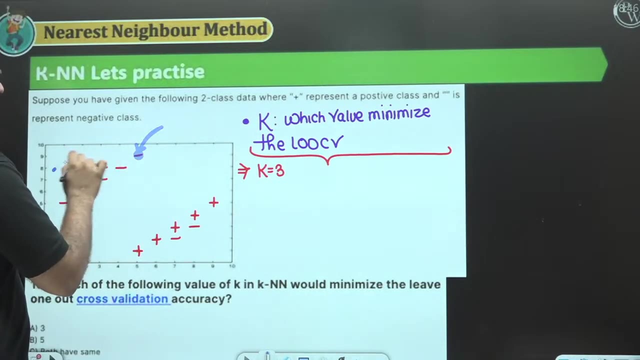 Or k equal to 5. So first let's take k equal to 3. So how will we do this, friends? I will explain you a little, As generally happens in leave-one-out cross validation, What will happen, friends? We will keep any one point for testing, And then we will make the rest of the training data. 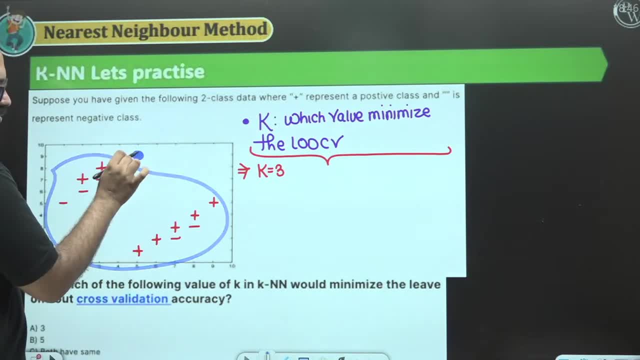 And then testing will be done on this point only, Which we left out. Then in the next step we will catch the other point As a testing point And on the remaining data Training will be done, And then we will see the testing of this point, That, how much accuracy it is coming. 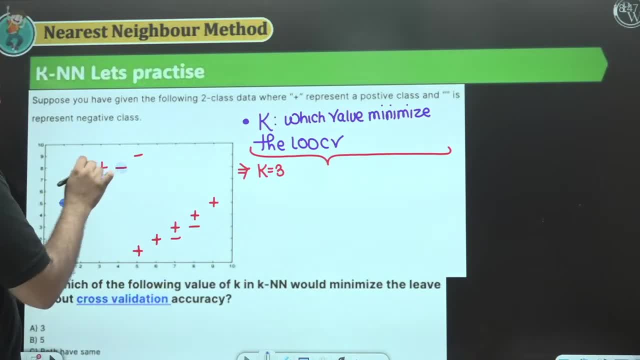 Like this: we will catch this point, Then we will catch this, Then we will catch this, Then we will catch this, And so on. We will catch each point one by one. It looks lengthy, but actually it is not so lengthy. it is easy steps. we will understand it very easily. 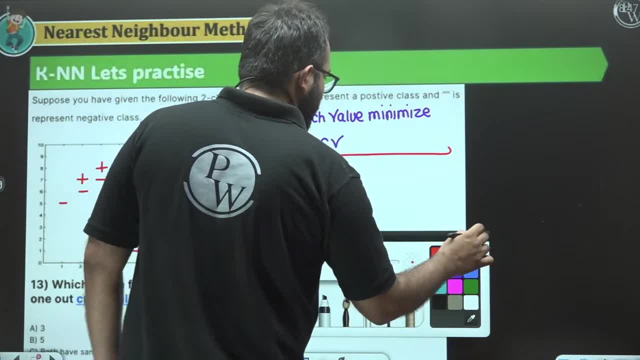 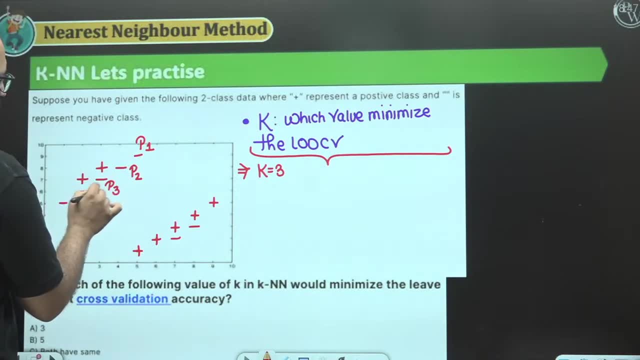 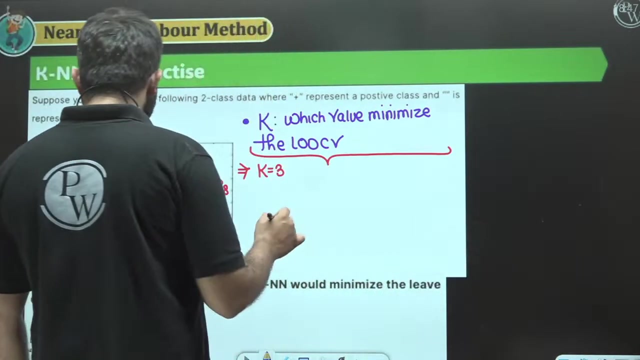 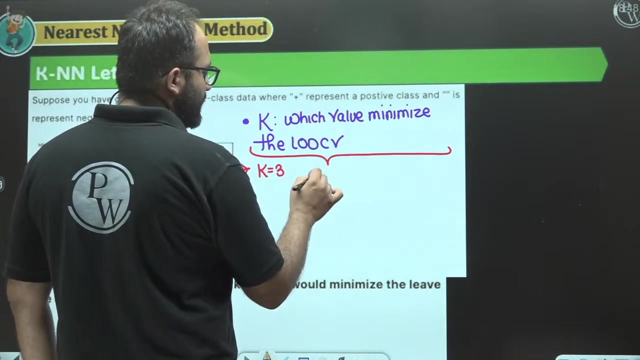 So let us assume points P1, P2, P3, P4, P5, P6, P7, P8, P9, P10, P11, P12, P13 and P14.. Now if I tell you, friends, I have kept P1 for validation, I have kept P1 for validation and the rest I have done training on the whole right. 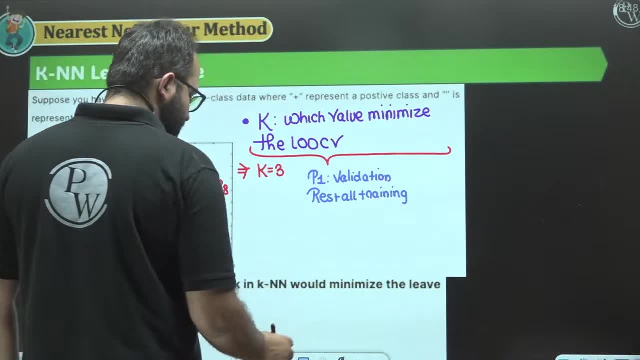 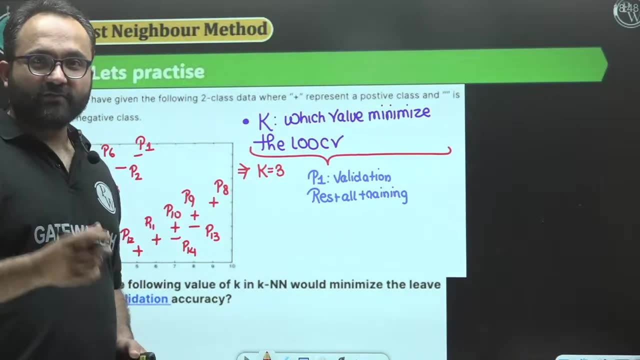 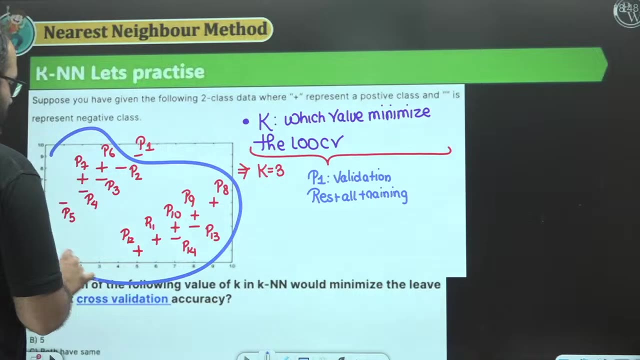 The rest we have done, training on the whole. now, think when we will keep K equal to 3 and bring P1 point, then what will come? what accuracy will come? Think about it. so you will say, friends, that, sir, we have kept this whole data, we have kept training data and now we are keeping P1. 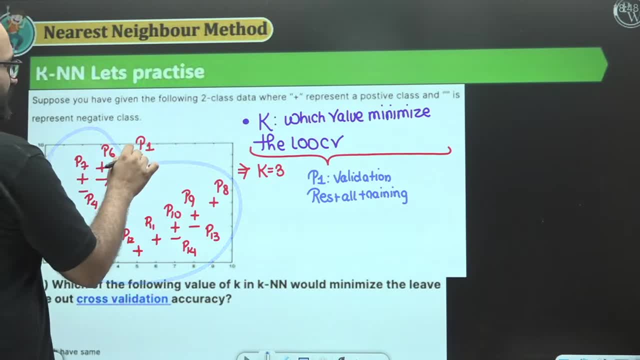 So as soon as you keep P1, then what will it do? now? it will find the nearest 3 points from P1, so the nearest 3 points are 1,, 2 and 3, we can see by doing this right. 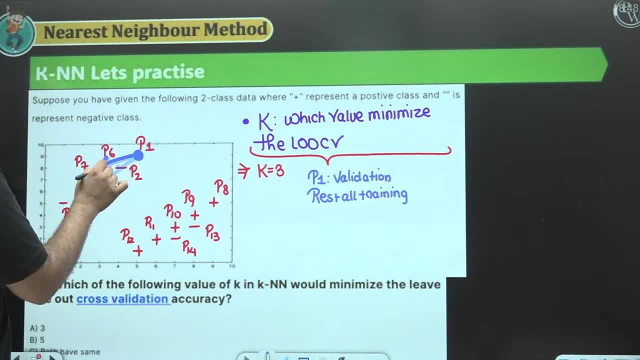 We can see by doing this. so if you see from here, then you will say, sir, 1,, 2 and 3.. So we can see here. So we can see that the accuracy of P1 is correct, because if we see 3 nearest neighbors, then in 3 nearest neighbors, in 3 nearest neighbors, we have in 3 nearest neighbors. here you can see. we have this point, this point and this point. 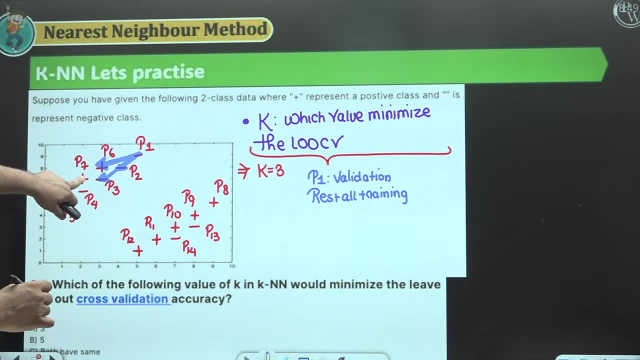 Right, Because this will be far away. this one will be far away, right, This will be far away. So, for this point, you will see that we are getting 2 points of class 0. And 1 point of class 0.. 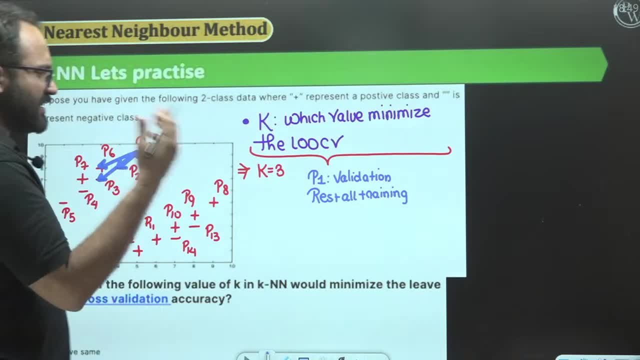 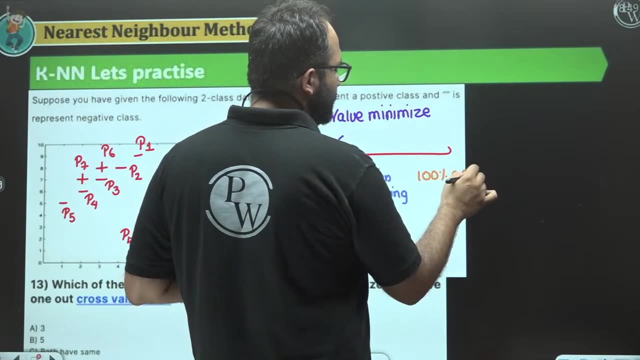 So for this point we are getting class 1.. So for P1, the estimated value will be absolutely correct for its true value. So here you will say that your 100% accuracy has come. You did not have any problem in this. 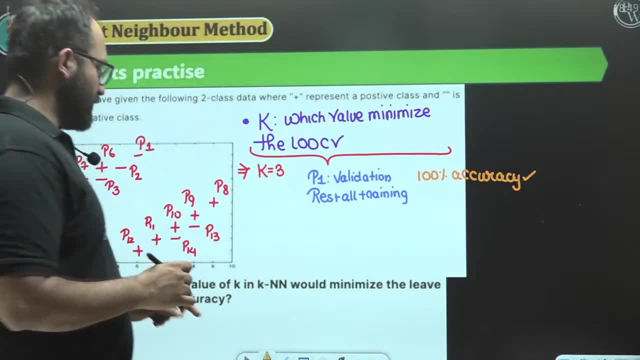 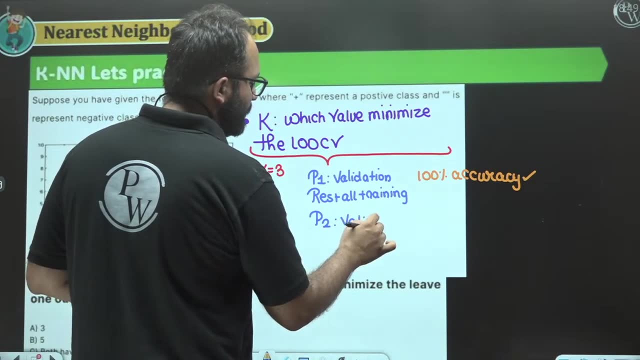 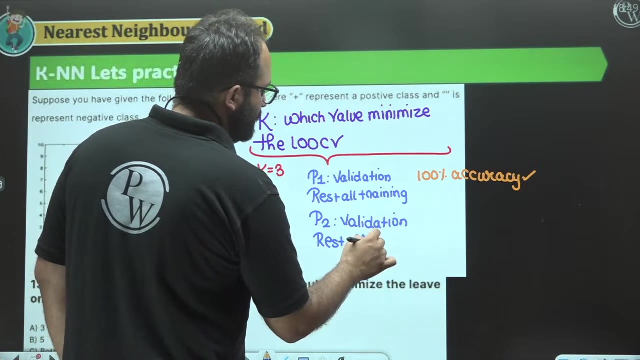 Who understood this thing Tell me quickly once. Ok, If we see the second point now, what are we doing, friends? We are keeping P2 for validation And on the rest of all, we are rest, all. Ok, We are keeping P2 for validation. 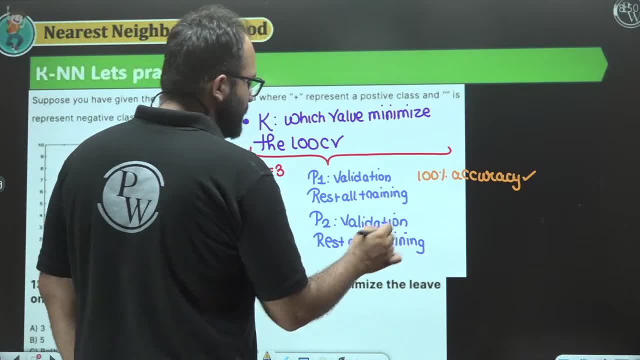 Now which data points we have. This the data which you can see here in this dialog box. Now you see that data points which are telling that the comments in this dialog box is not used in this relationship with users of that, then that means this is the Vehicle. 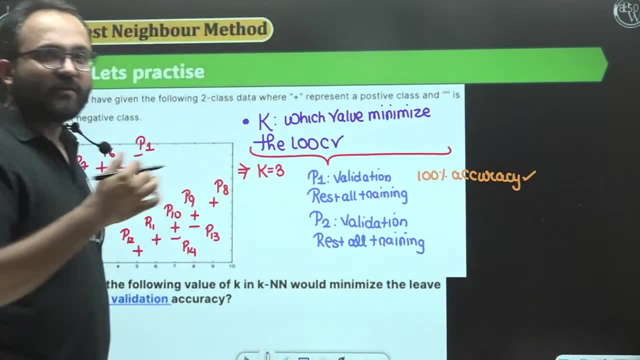 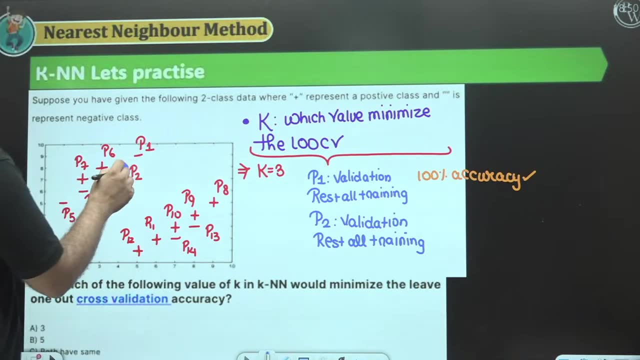 category. But if you think a little, you will be able to see that there are always other data points in them. Let see from this point: we set P2 as the мин times and Min times. we set P2 as min times. Yes. 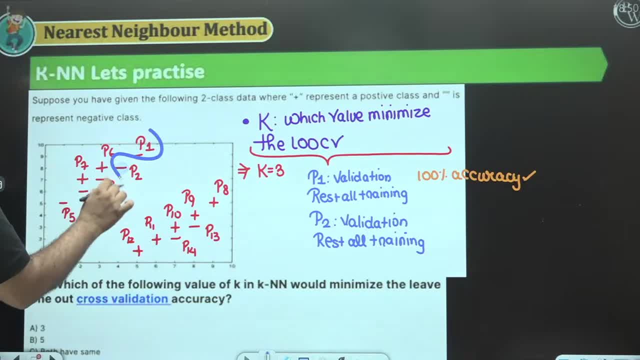 So we are taking from that answer that we can see the negation and we will solve this. what's the negation and what's the thing? Look right now from the symbol: gets it. I have a salute from P1 to P2.. 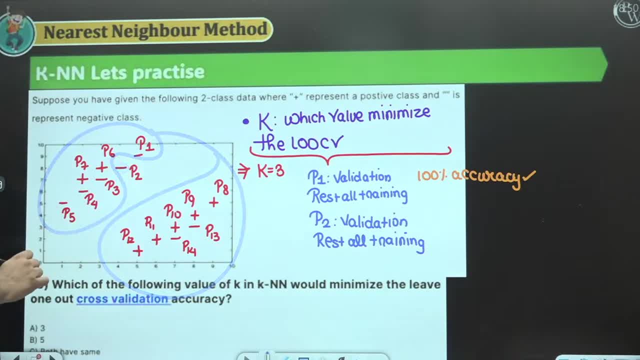 Just think about Now. you see that the data will himself Right. So for P2, you can see what is nearest. one is this, one is this and one is this. So obviously here also you can see that two classes are coming from 0 and one class is coming from 1.. 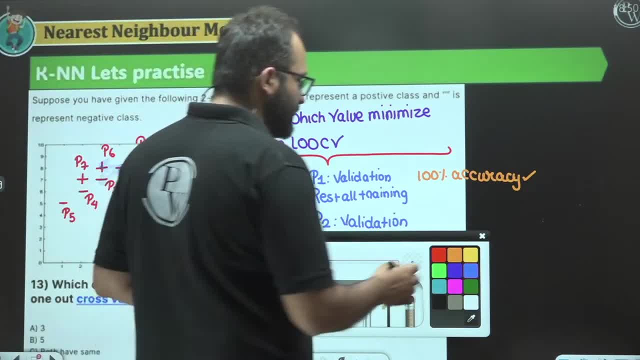 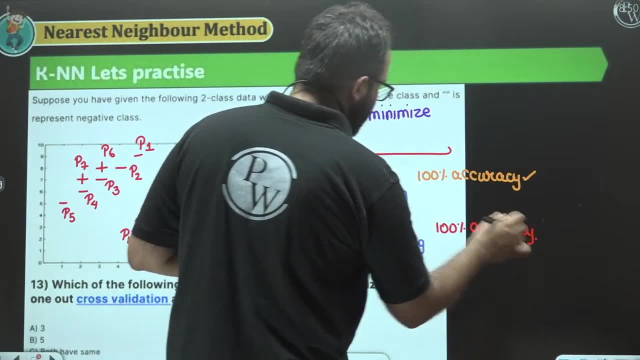 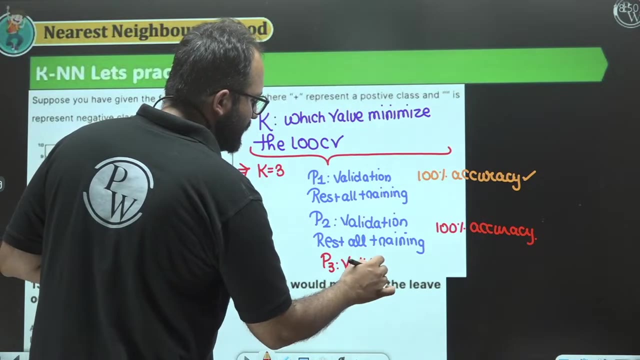 So according to majority, P2 is also coming accurately Means expected value is same as the true value. So 100% accuracy is also done in this case. Now, if we talk about P3, what do you think We are validating P3, we are doing validation on P3. 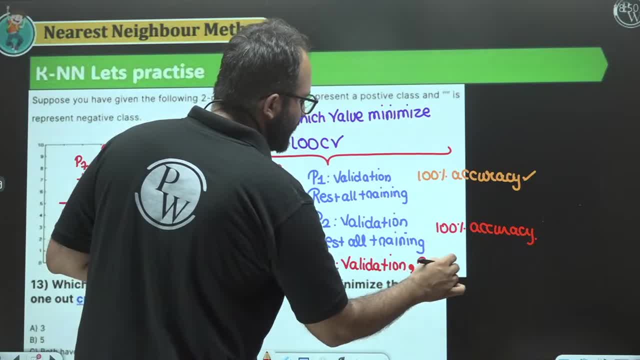 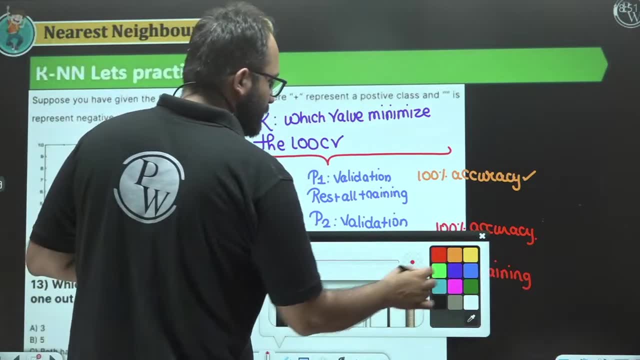 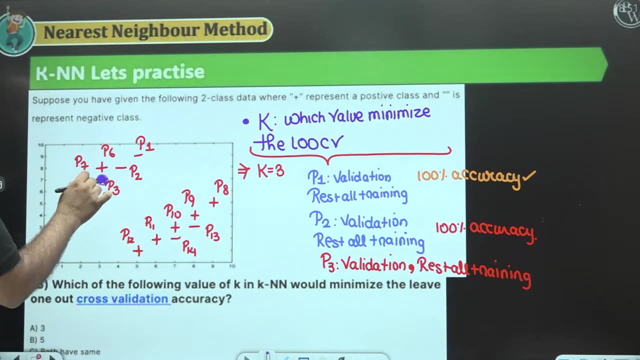 And rest all training. So now you see, friends, we are doing training on P3.. Means we have kept P3 as a test or validation point. So in the case of P3, you will see that this point is near, this point is near and this point is near. 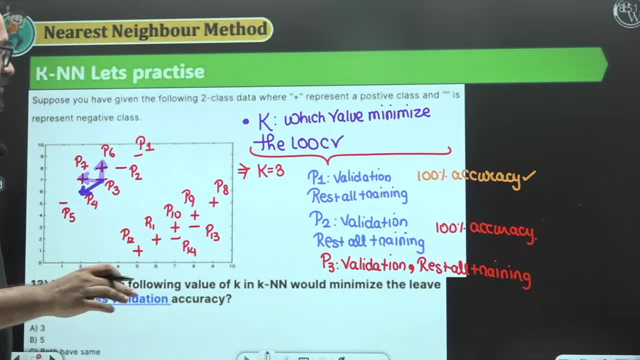 So in this you will see that error will come in P3. Why? Why? Because here in the plus point pass there are two plus and one minus. So obviously we can say: or P2 can be our nearest Means, these two will remain. and third is one. 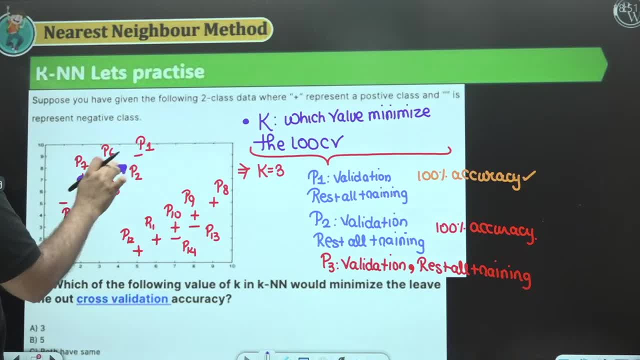 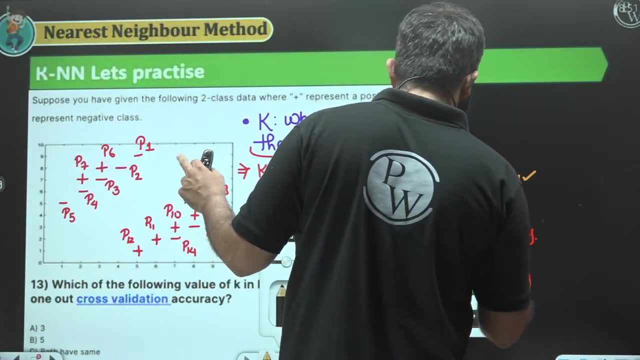 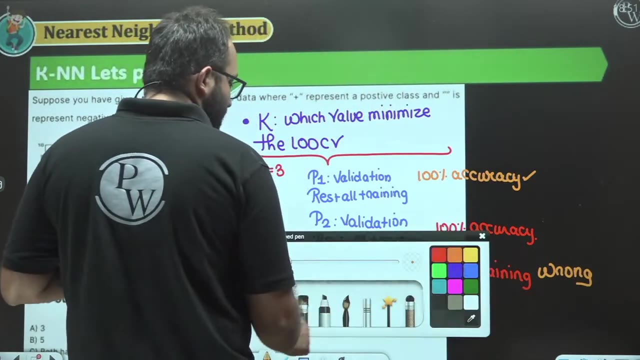 So here you will see that there are two plus nearest and one minus nearest, And thus here our accuracy is spoiled Because our 3nn will give it plus sign. So here the whole story will be wrong. In P3 the story will be wrong if we will validate P3. 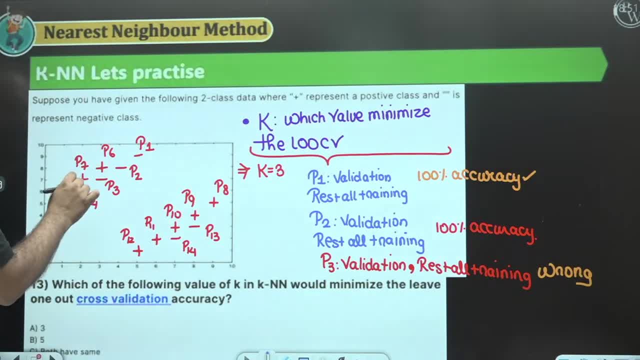 Similarly, now we will see P4.. So in the case of P4, you will see that here the accuracy will be made. In this way, you will see that this point is near. Then here the minus point is near, and here the minus point is near. 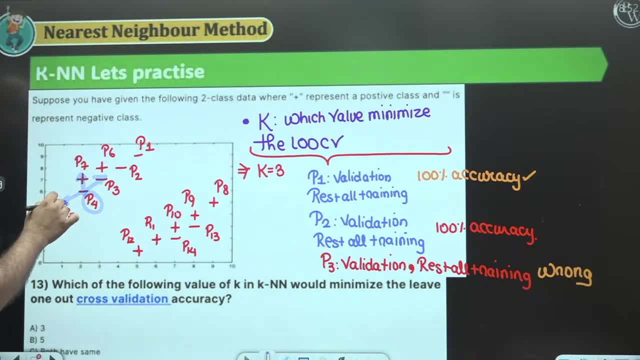 So everything will be right in P4. Similarly, in P5 also it will be right. This one is in the plus pass and the minus one is in the two pass, So in P4 and P5, if we do validation. So everyone understood that we will get accuracy in P4 and P5.. 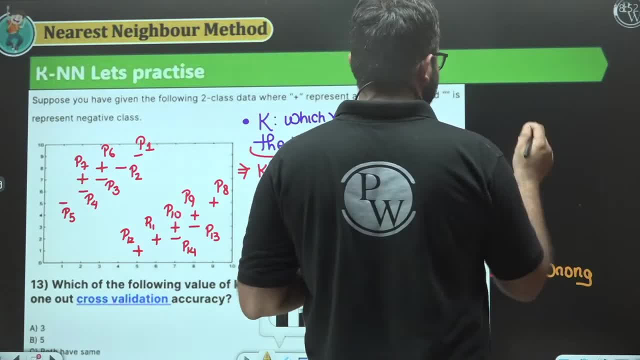 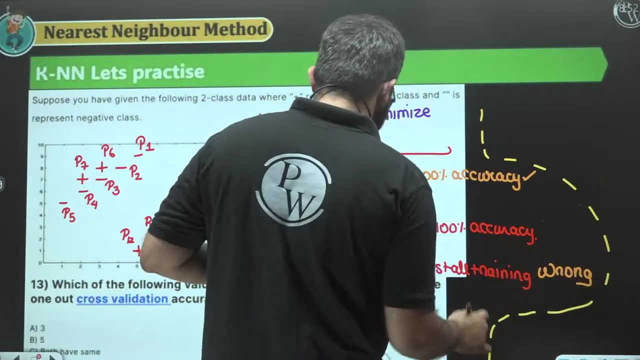 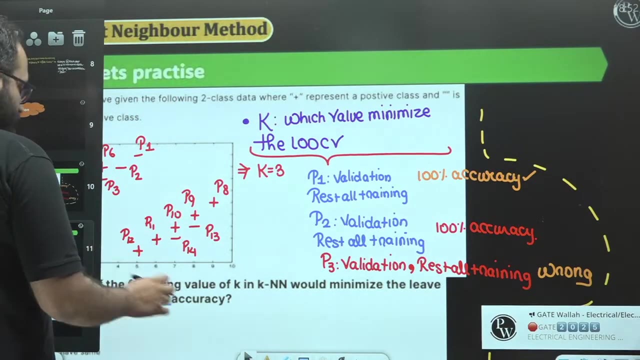 And now the question is: what about P6 and P7. If we keep P6 on validation, I will write this on the next page, Because that would be better. You will understand it very well. I will rub it. Sorry, I will not rub it like this. 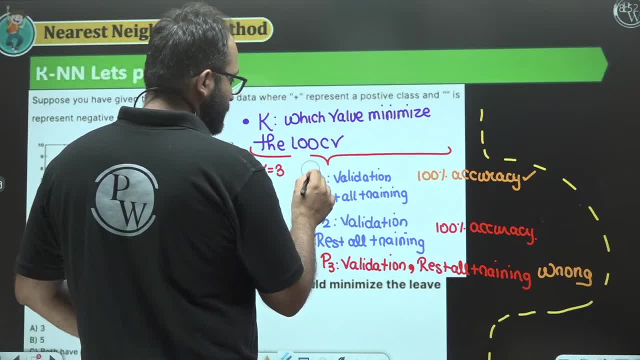 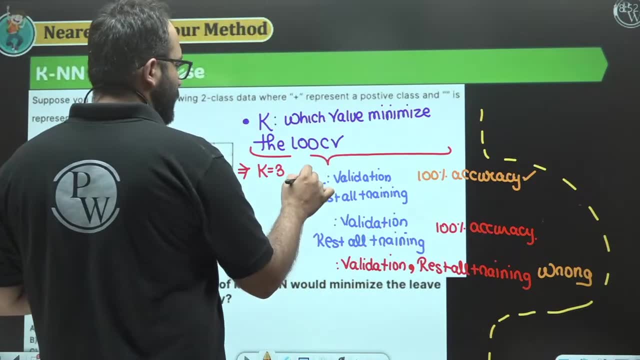 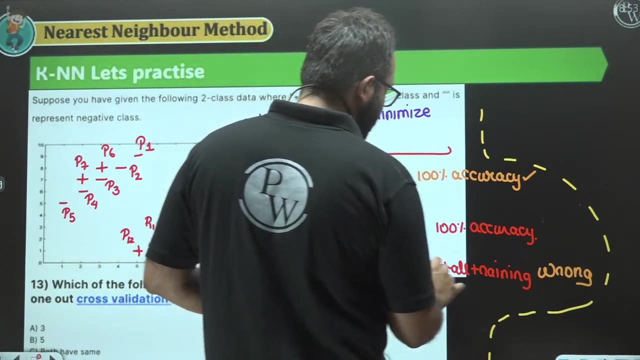 I will just rub point P, As I told you that if we are taking on P4 validation or P5 validation, Then we will see 100% accuracy in this. We will see 100% accuracy. There is no problem in this. 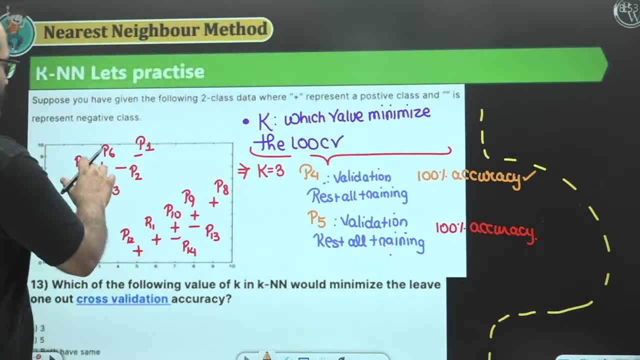 But now see here, Think and see. If we keep P6 on validation, Keep P6 on validation And this is the whole data training. We are validating P6 now, So when P6 will come for testing, Then what will be the nearest neighbor? 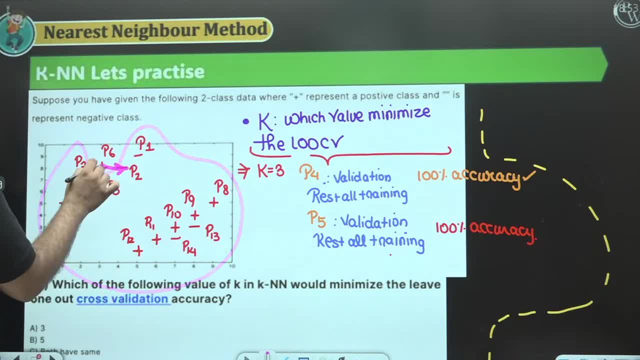 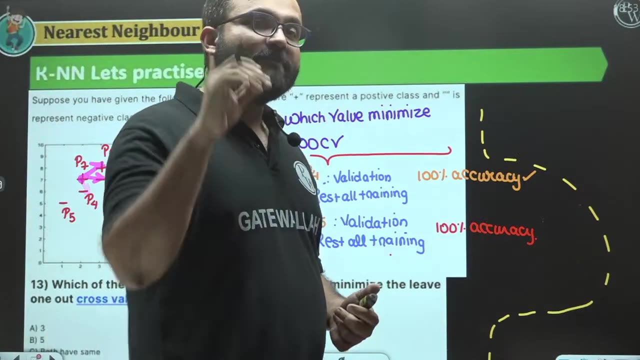 This one, One minus and one more minus. So obviously this minus will be predicted Exactly in the same case. If we keep P7 for validation, Then near P7 1 plus and 2 minus will come. So P6 and P7 will always be predicted minus. 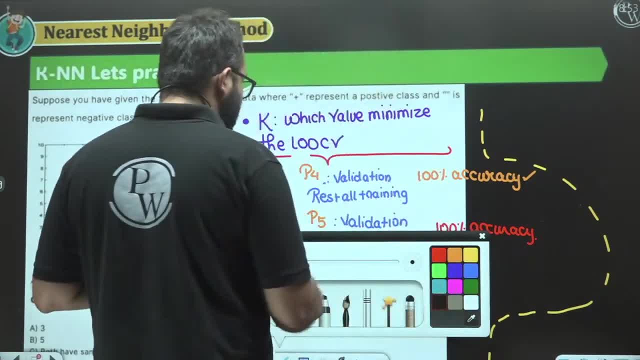 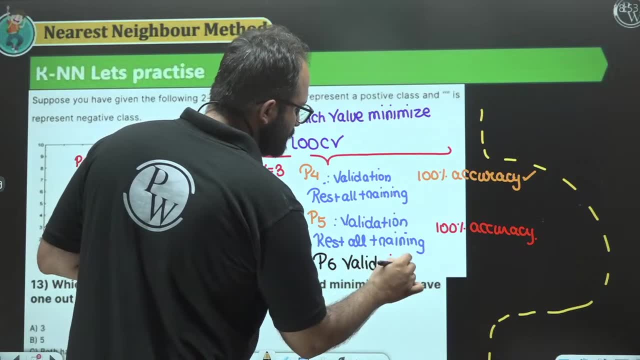 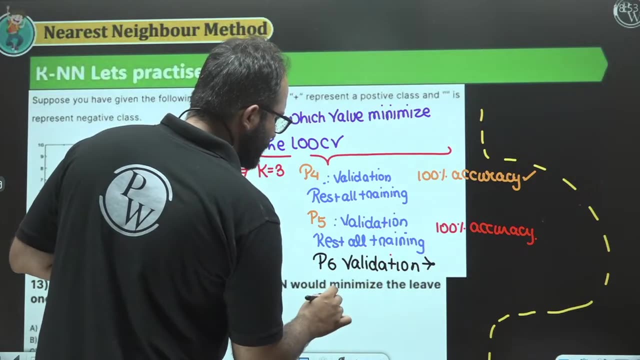 So in the case of P6 and P7 you will definitely get error. Who understood this? If you are keeping P6 for validation, Then here error will definitely come Okay. And similarly, if you are keeping P7 for validation, Then here also you will get error. 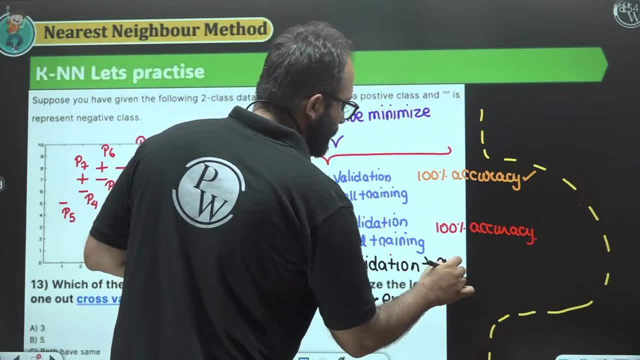 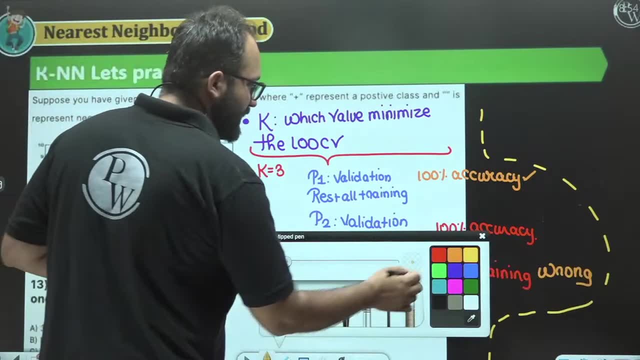 So you can see If we did like this, Then you got error in the above three points, If you are keeping K equal to 3.. If you think a little, Then it will be done easily. There is no need to write so much. 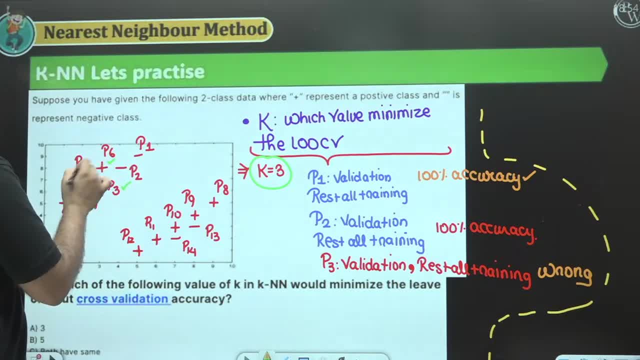 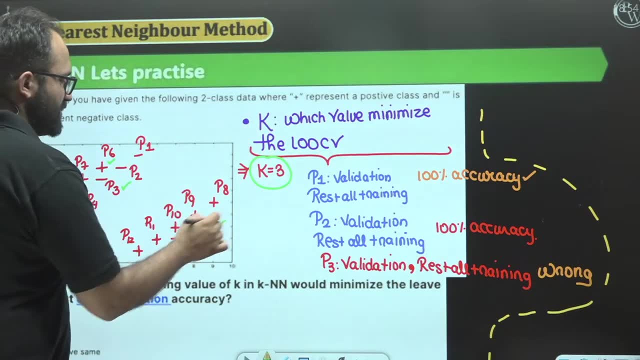 For K equal to 3.. At this point, At this point And at this point, You got error in three places. Exactly same story will be below: For K equal to 3. Where P13, P14 and P10 will give error. 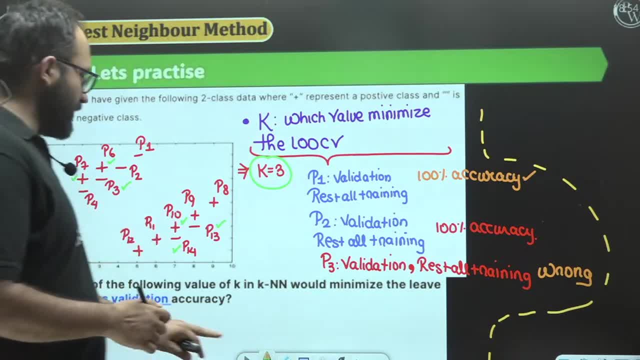 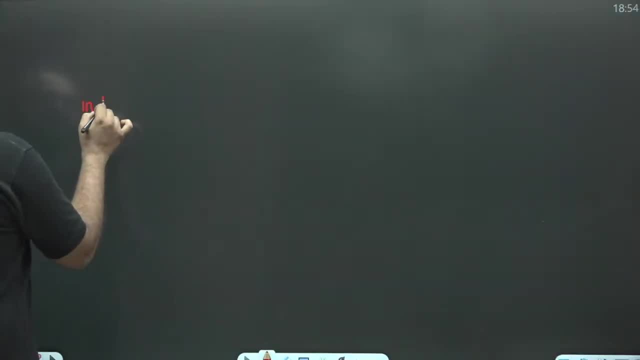 Okay, So here also these three And here these three. So you will see Overall, If you will see here. So, as I told you, In leave one out, cross validation, We have 14 points. So in 14 points, as I told you. 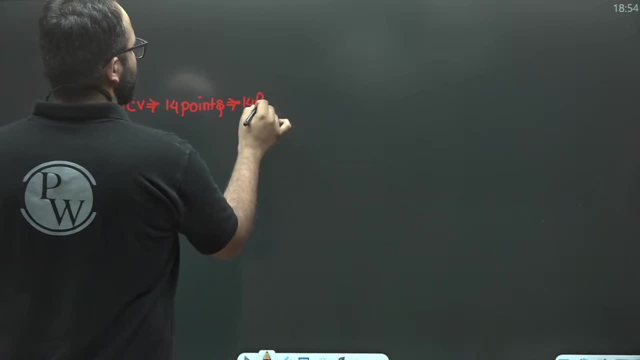 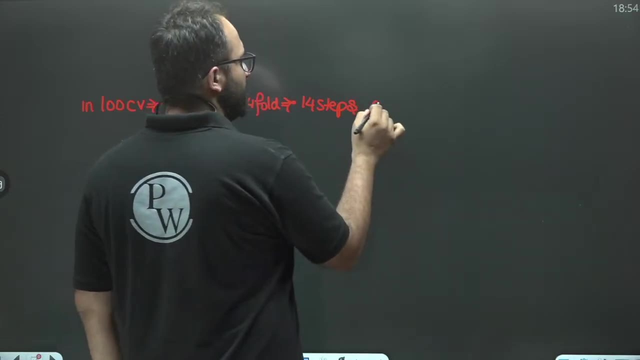 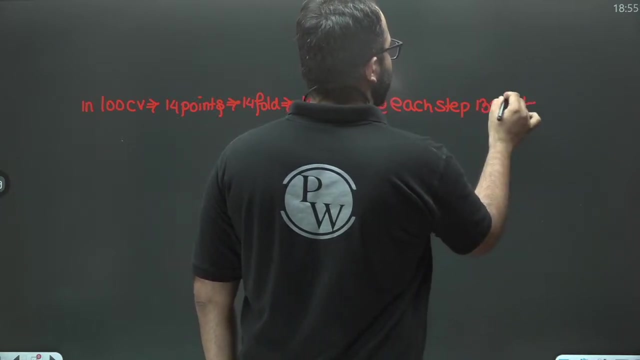 You create 14 folds. So here, 14 steps are done, Friends, Where at each step, We have 13 points of training And one point of testing is done. Okay, One point of testing is done. So you can see this easily. 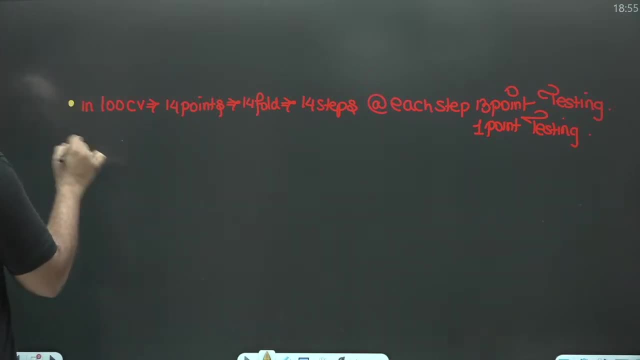 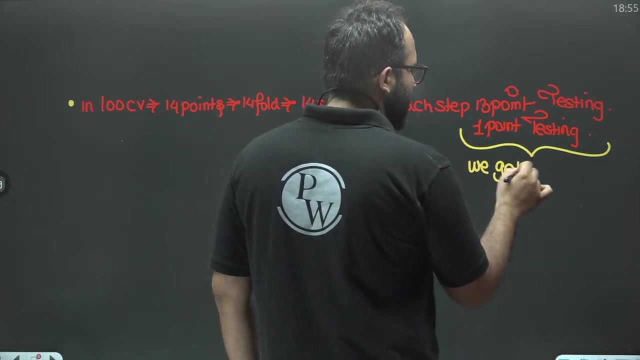 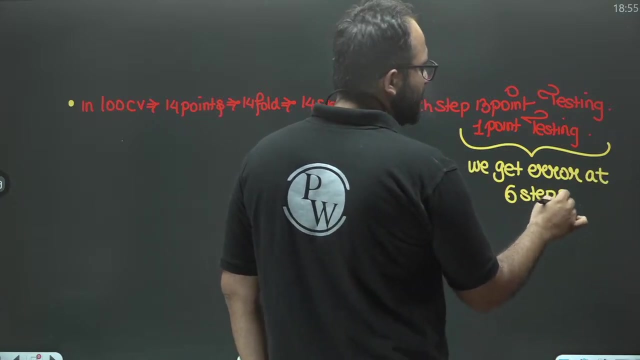 Okay. So this is very, very important. You can see In this whole process How many errors are there, Friends? We get six errors. We get error at six steps. You got error in six steps. Tell me Who understood it fully. 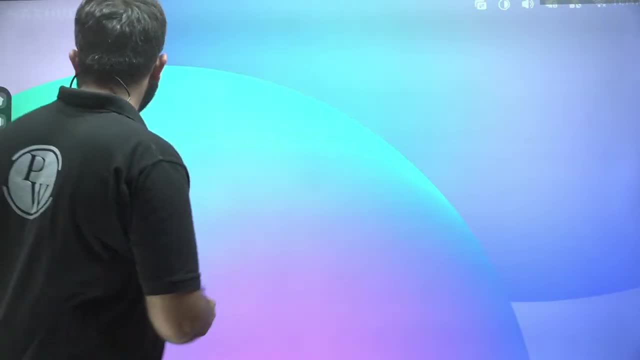 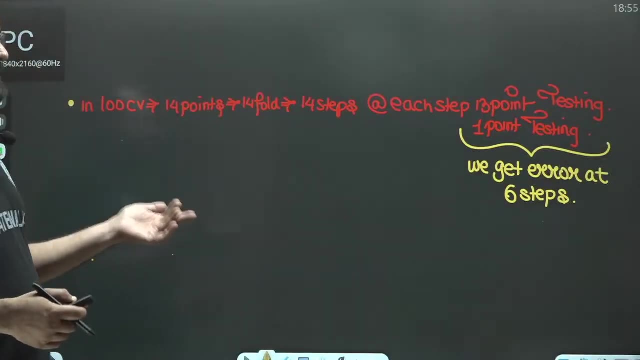 Whole process. Can someone tell me once, Sir, The whole process is clear to us. We have understood the whole process, That That Overall in six steps Means in six points. We got an error Means like If I keep P3 as a validation. 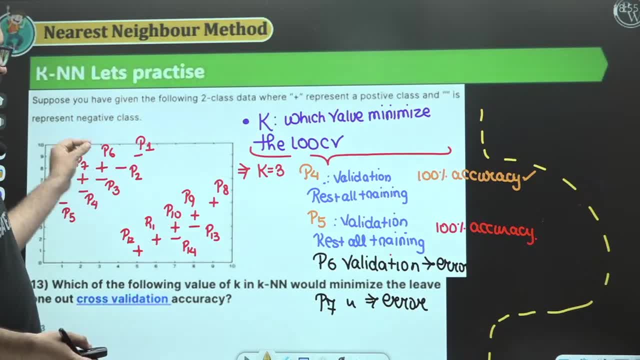 And if I keep all of them on training, Then error will come. P6, P7.. Keep P6 for validation, Then error will come. Keep P7 for validation, Then error will come. For validation: we get error. For validation: we get error. 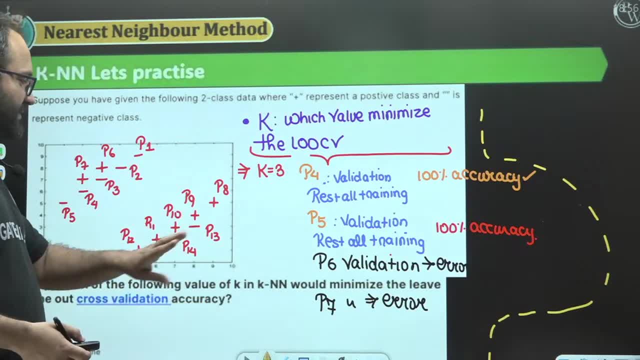 For validation P13.. For validation P14.. For validation P10.. Then error. We will get error like this. So in six points Or in six places, We got errors. So for K equal to 3.. It happened like this: 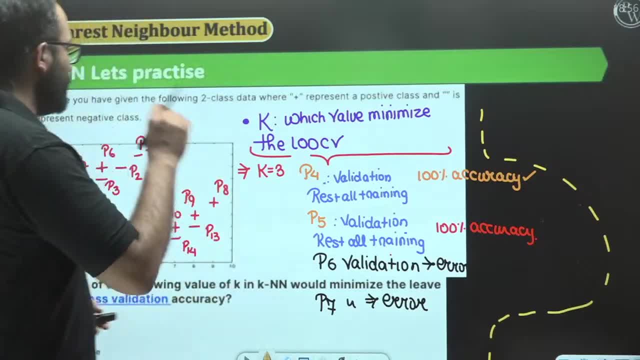 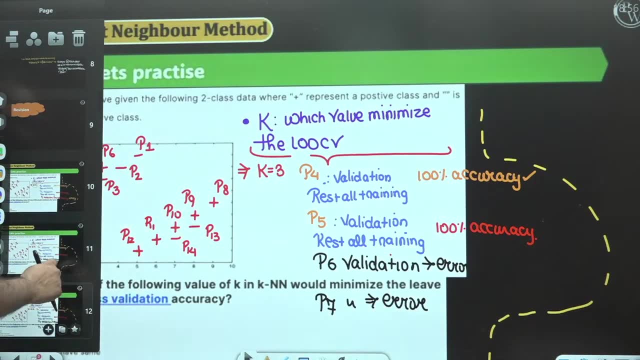 Now, what about K equal to 5.. Think about it: K equal to five. In the case of k equal to 5, I am not going to solve You guys tell me the students who are actively sitting in the class. what do you think? in which points case you will get an error. 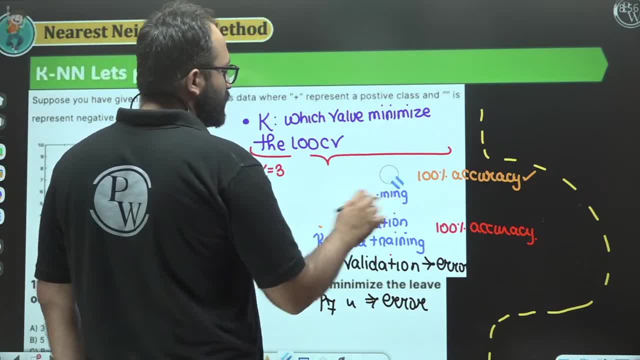 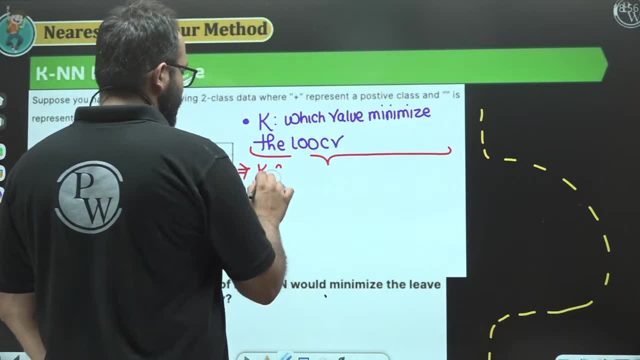 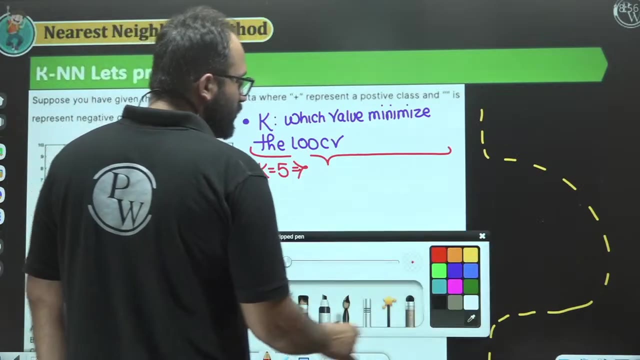 If I take k equal to 5, then now tell me in which points case you will get an error. Think about it. So if I take k equal to 5, then now tell me in which points case you will get an error. 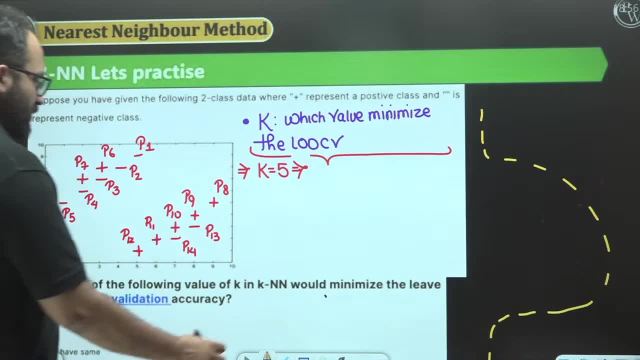 Can anyone tell me? So now you guys do it and see, For example, now I was afraid of p3 first. So if I keep p3 as a validation point and rest for error, rest for distance, then see: 1: minima is this, 2nd is this, 3rd is this, 4th is this? 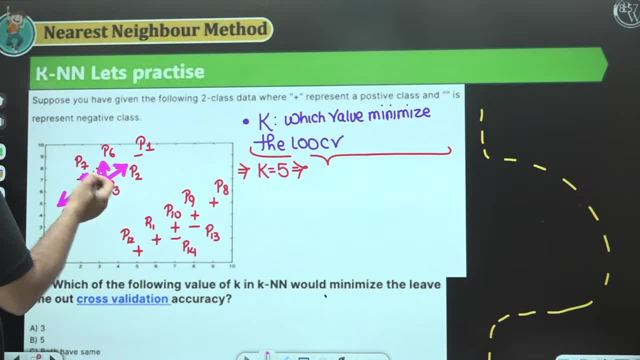 and 5th is this: take any of them. This is the case. So if I take p3, then now tell me in which points case you will get an error. Take this one, come on, So you can see, in this case, in p3, there will be no error. 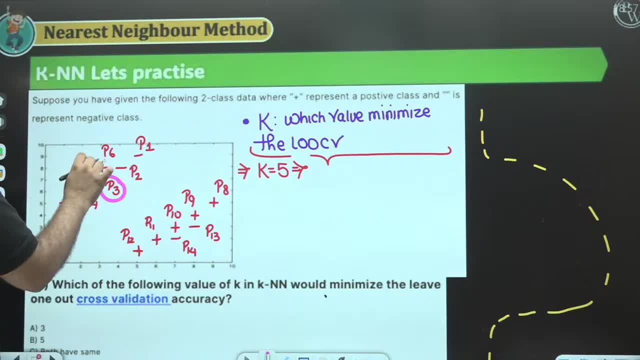 because k equal to 5, means I will see 5 nearest neighbor. so in 5 nearest neighbor, 2 are plus but 3 minus ones will come. This, this and this: Okay, 3 minus ones will come. 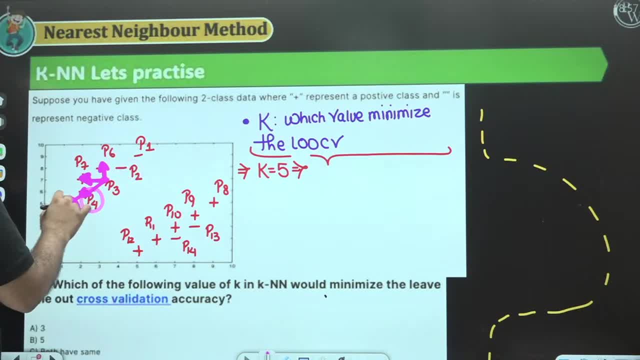 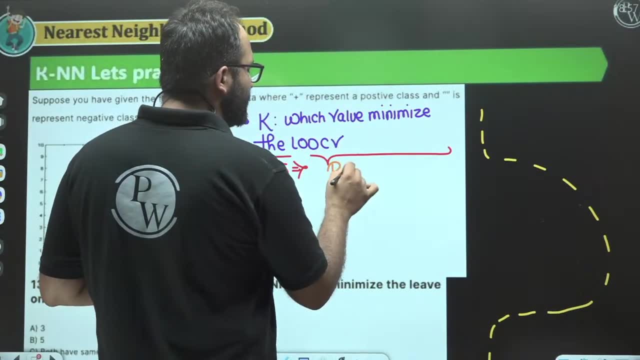 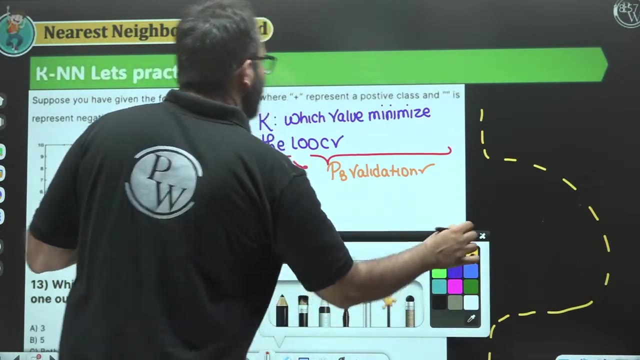 This, this, this. Okay, So we can say: in this case there will be no error in p3.. If we keep p3 as a validation, then it will be correct, there will be no problem in this. But obviously there will be an error in these two. 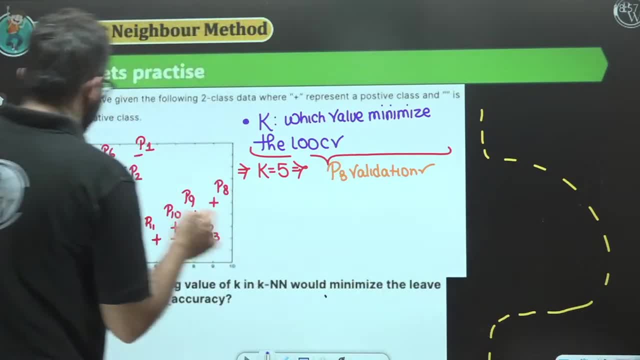 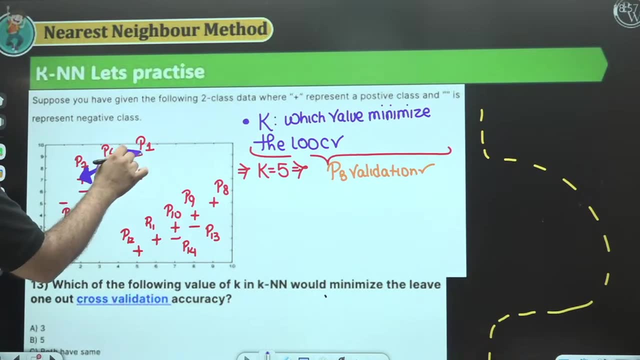 In p6, there will be an error, but no one can stop it, Because if we see p6, then in p6, there will be a minima distance: 1,, 2,, 3,, 4, and 5.. 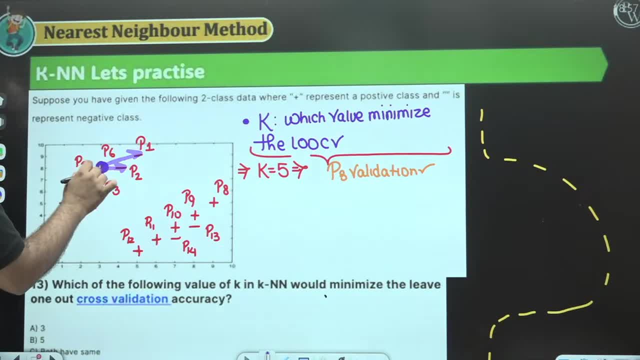 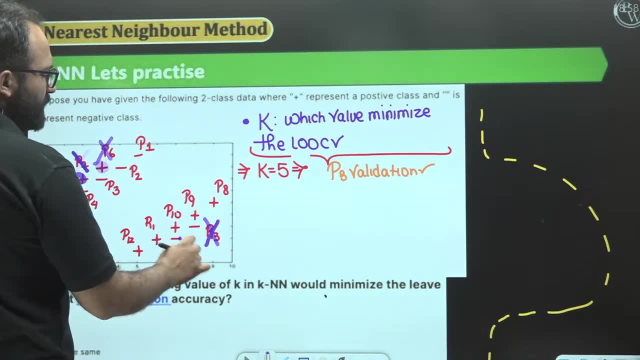 So in this you can see 4 minus 1 plus, so this will be a minus predict. p7 will also be a minus predict, So there will be an error in p6 and p7.. Similarly, p13 and p14, there will be an error in p6 and p7. 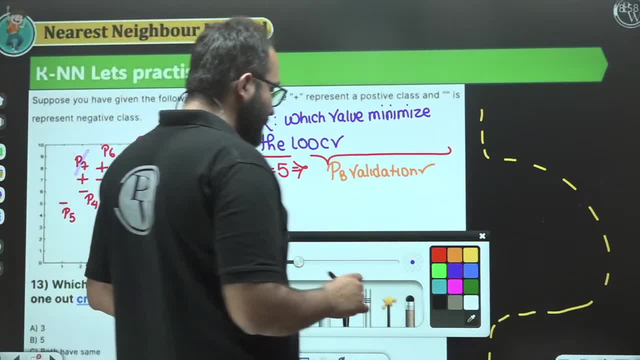 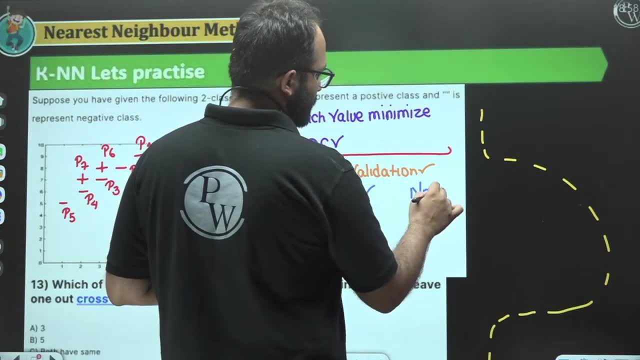 So there will be an error in p13 as well, but there will be no error in p10.. So here, p3 and p10, there will be no error in validation. There will be no error in this case. There will be no error in p3 and p10. 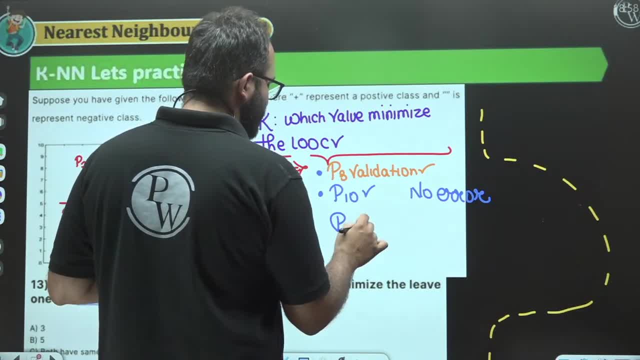 Only here. obviously, there will be an error in 4 points Like p7,, p6, and p10,, p14, and p13.. There will be an error in these. There will be an error in this. 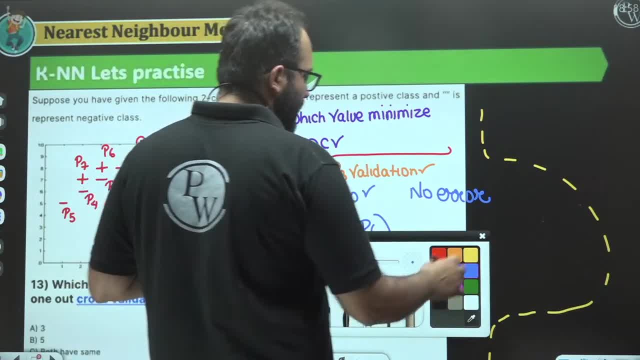 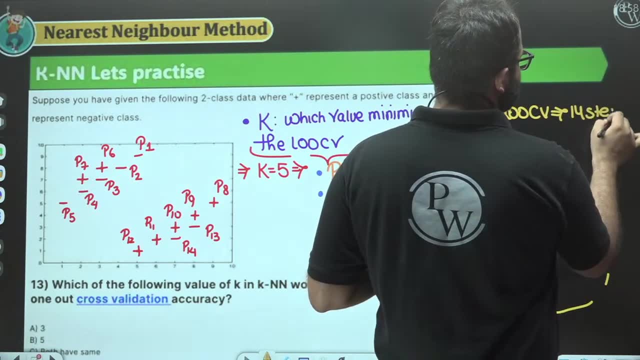 So here you can see if we are doing leave-one-out cross-validation or if we are doing leave-one-out cross-validation, then in that case, out of 14 steps, there will be an error in only 4 steps. 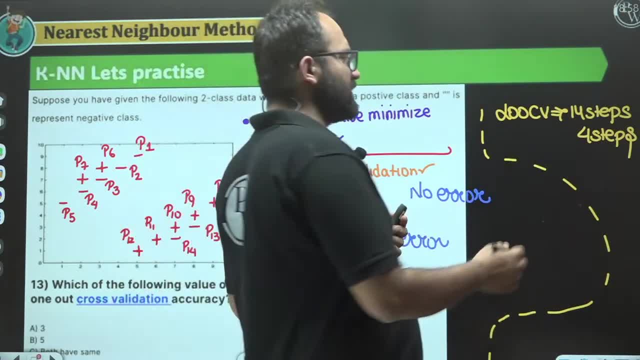 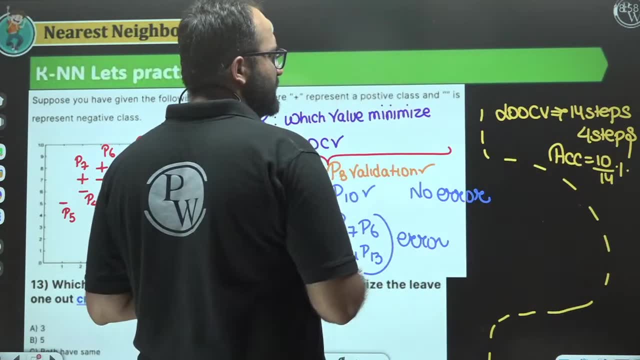 Rest, everything will be fine. So here you can say how much accuracy will it have. Accuracy will be 10 upon 14%, Because out of 14, there is a mistake in 4, 10 is correct. 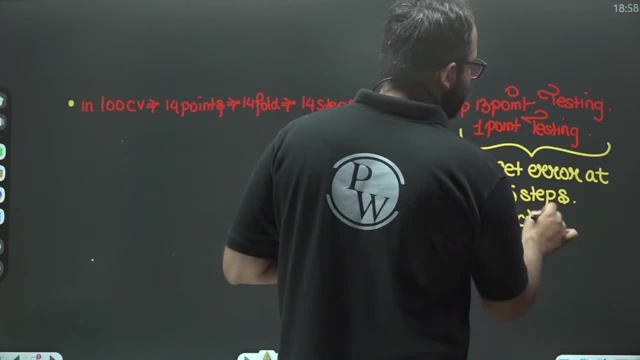 And similarly, how much accuracy will it have here? Accuracy: out of 14, 6 is wrong. So 8 divided by 14 into 100.. Okay, right, This is how the story will be made. So you can say: out of 14,. there is a mistake in 4, 10 is correct. 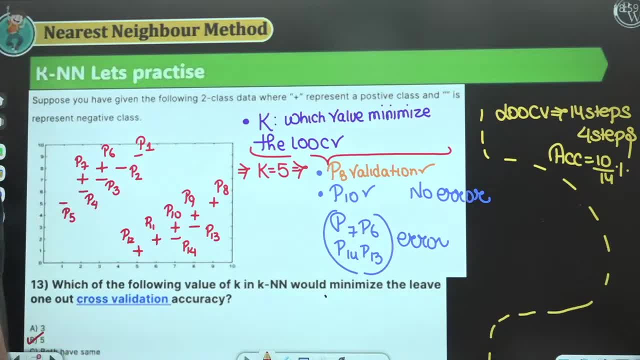 And similarly out of 14, there is a mistake in 4,. 10 is correct. B is the correct answer of this. I mean 5 will give you lesser error. This is a very good question. This is a very good question. 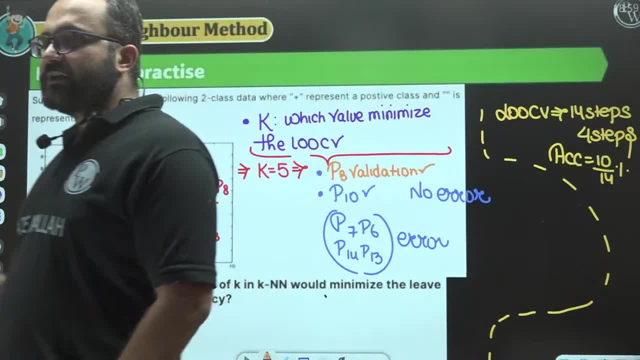 It is a very good question. It is a mind-related question. That's why, if you think it's a little lengthy, but this is a question which can be considered in an exam, This is a question which can be hung in an exam. 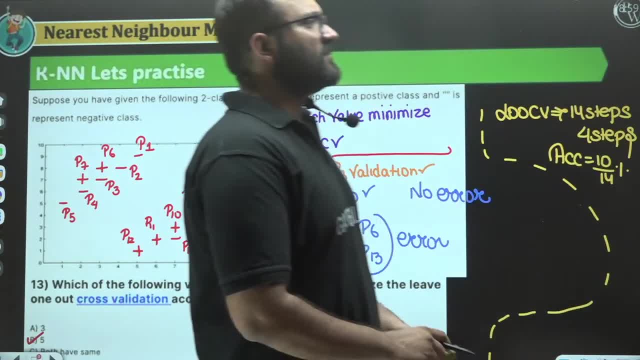 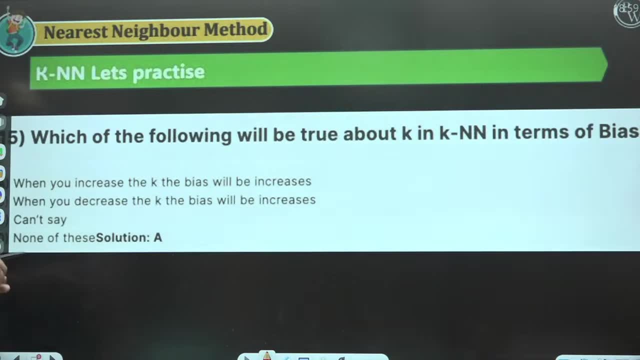 It's a good question. I mean, it's a question of the mind. Who all can understand this? Let's take a look at it next time, Come on, Okay. So it's a very simple question. Which of the following will be true when K is? 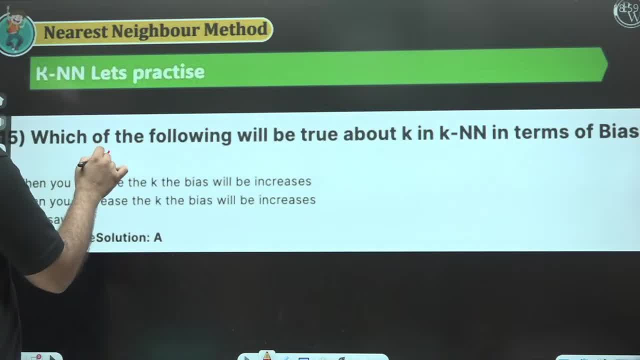 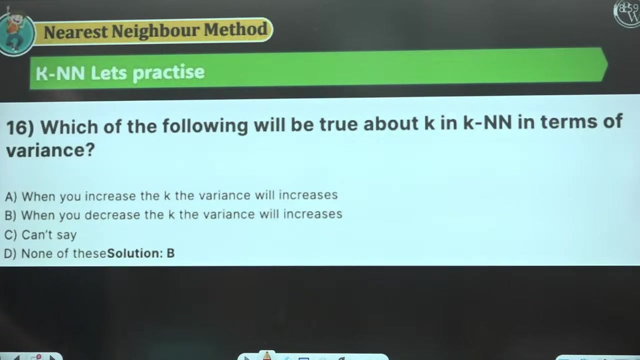 K in terms of market of y's. so you know that as k increases, y's increases. so when you increase the k, the y's will increase. there is no doubt in this. we have read it right. how k creates our problem means: when k increases, y's increases but variance decreases. we all know that. okay, which of the 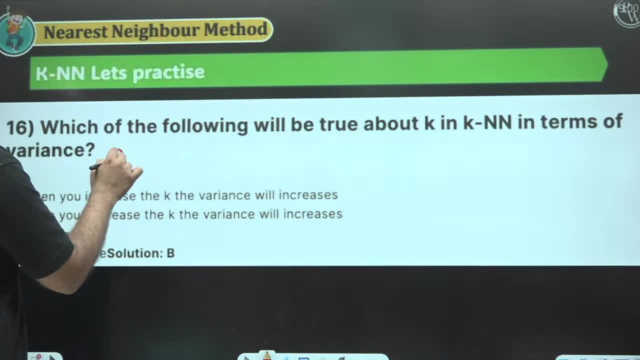 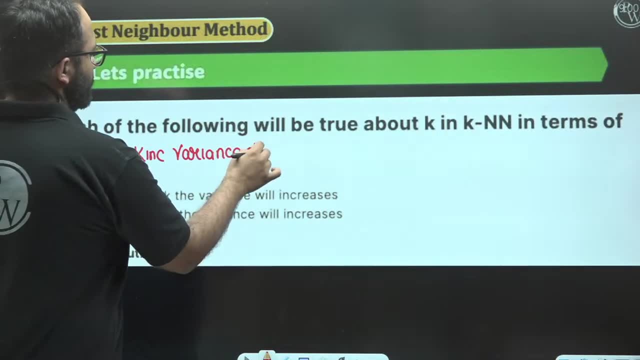 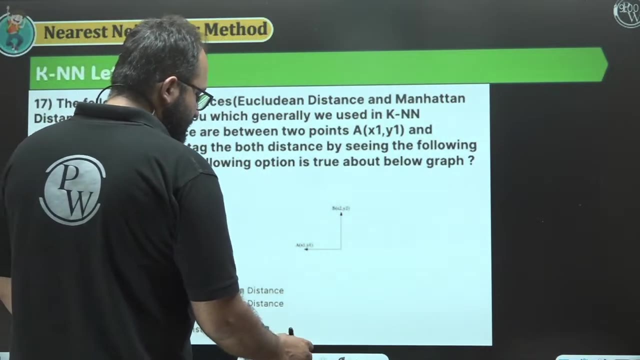 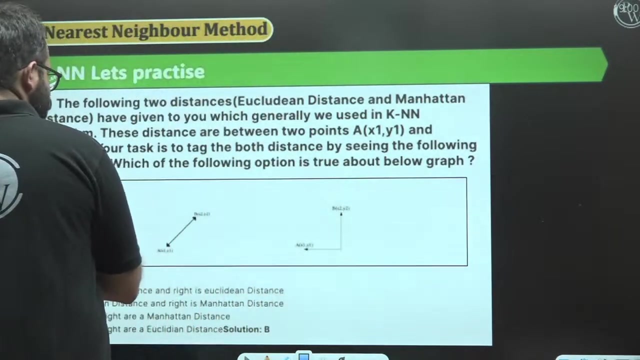 following will be true in terms of the variance. you also know that as k increases, variance decreases. okay, now see here, friends, which one do you think is manhattan distance i have taught you yesterday? tell me which distance is manhattan and which is euclidean distance. i will remove it because obviously you can't see clearly. what do you think? which distance? 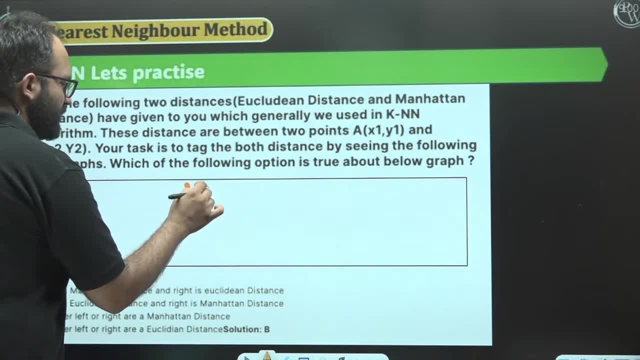 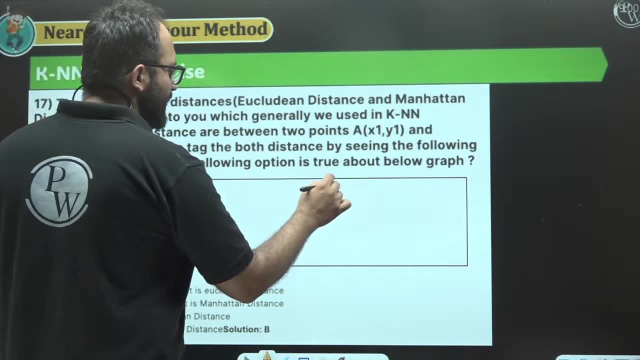 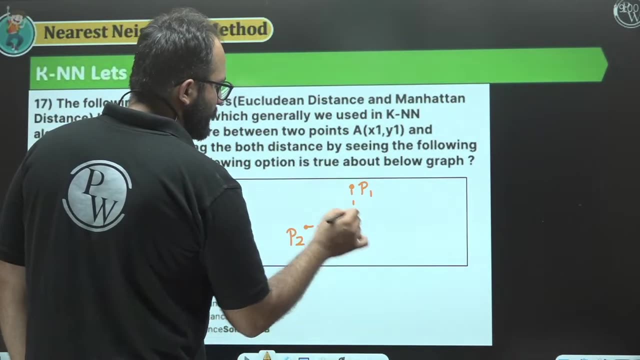 is manhattan distance, as you can see its 4 column, which means we have two points. now, lets say there are two points, friends. this is point nr 1, this is point nr 2. so what do you think that, which one doing my dilation and which one doing the euclidean distance? 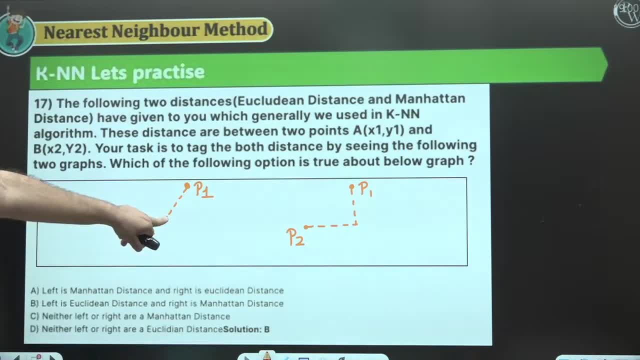 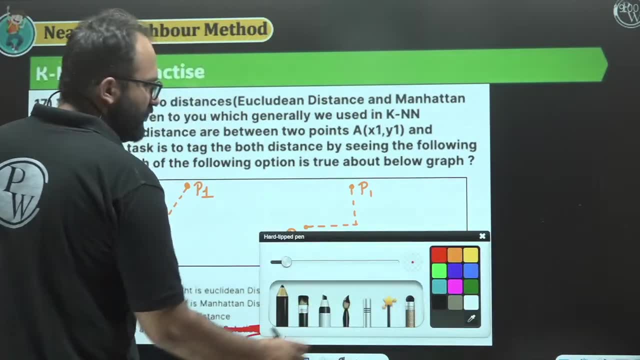 tell me which one doing that to us is euclidean and which is m, or to e? for this, four options we will give you, so count them for sure and tell us the formula of manhattan and euclidean. Let me know in the comments below. 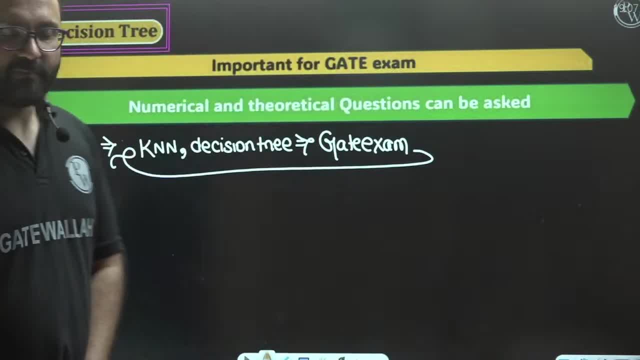 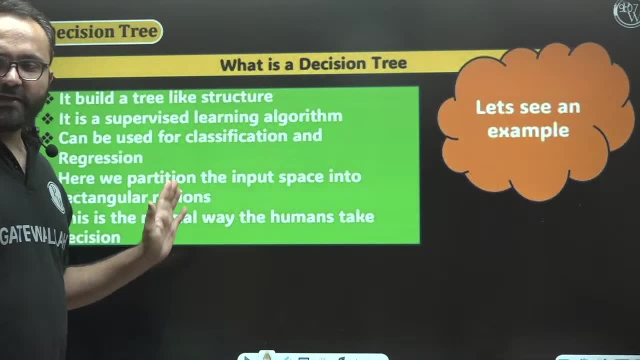 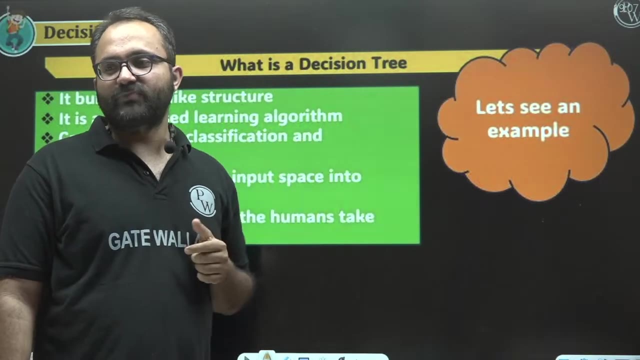 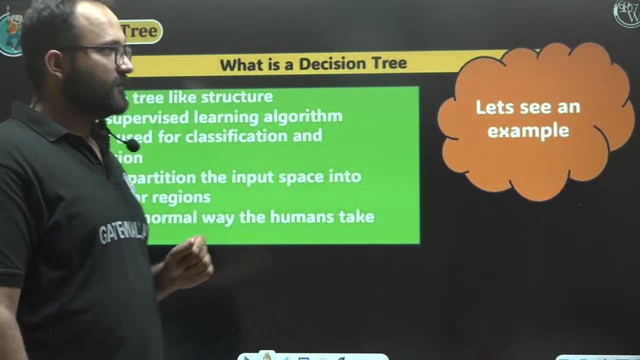 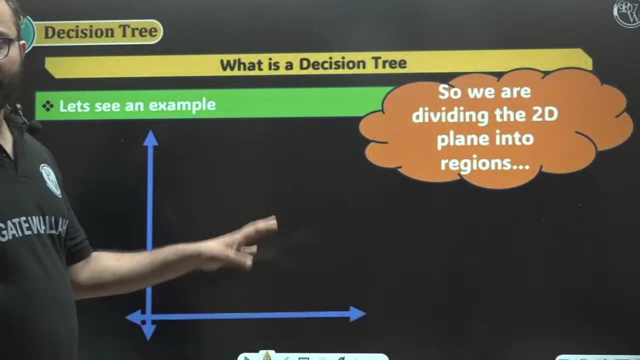 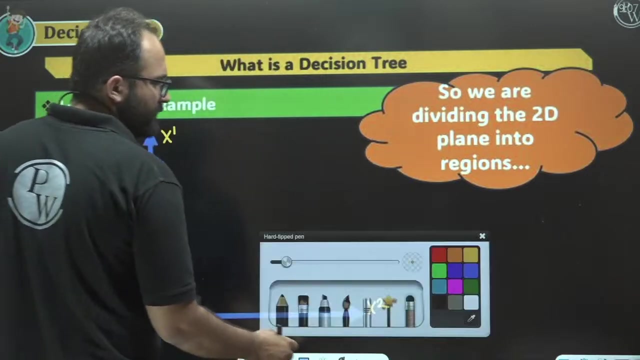 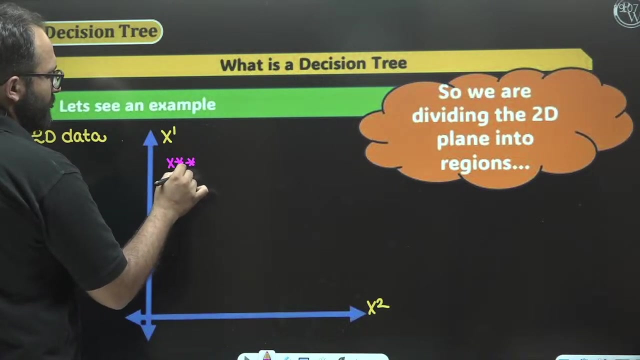 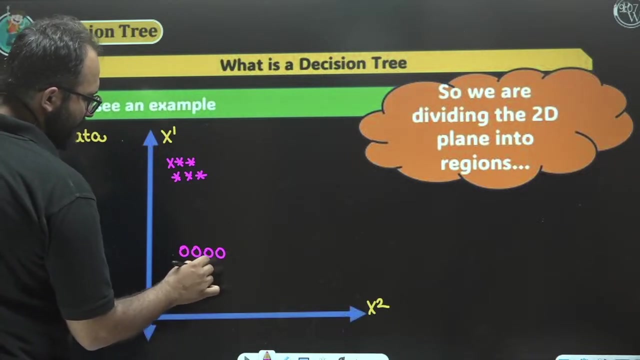 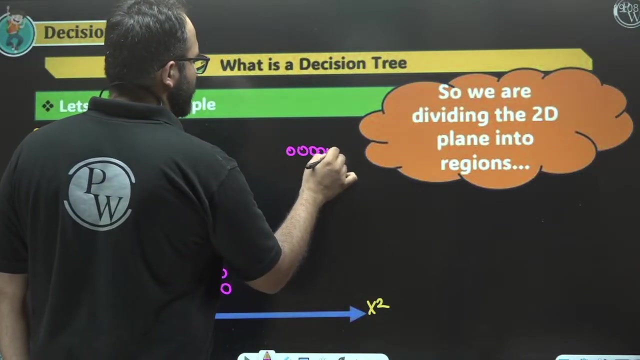 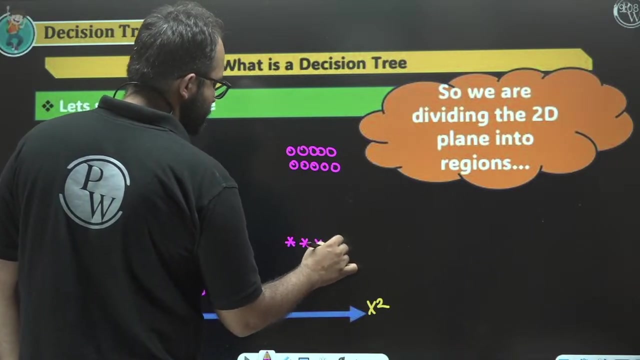 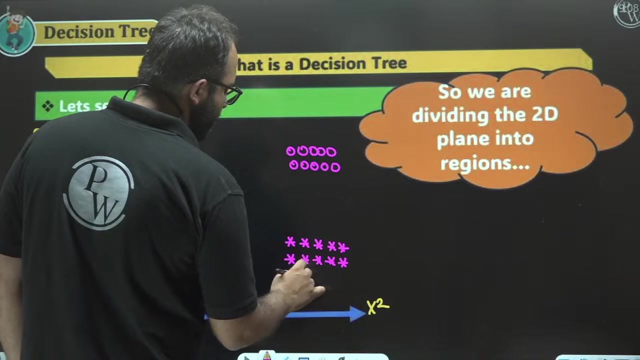 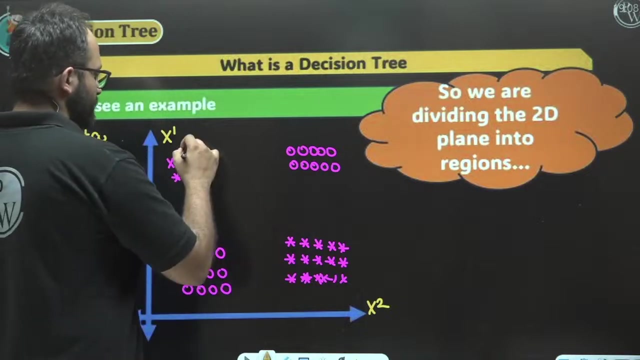 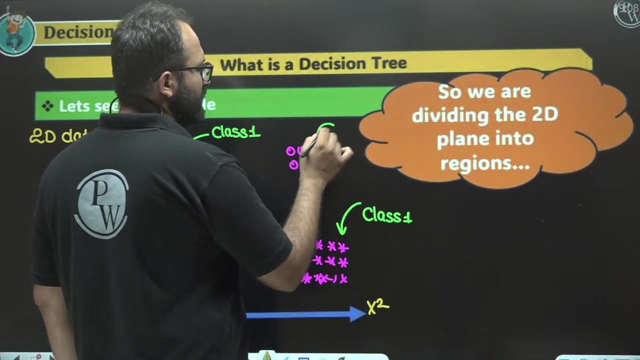 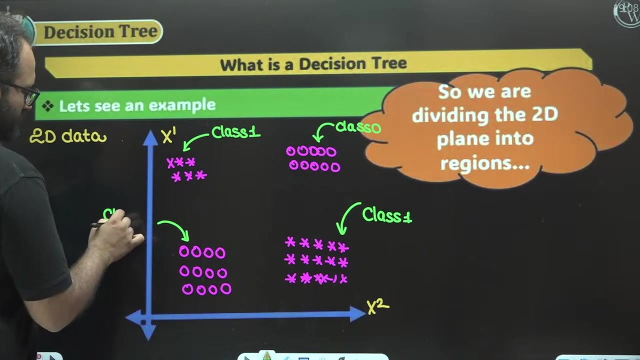 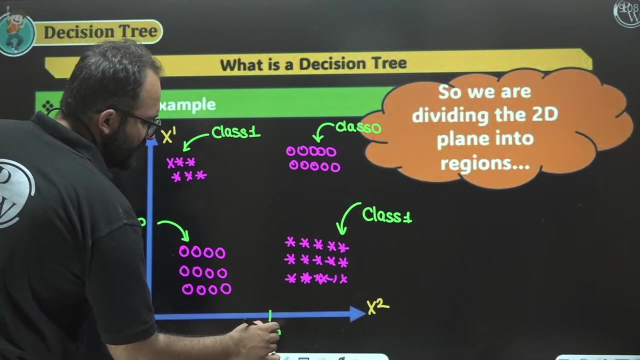 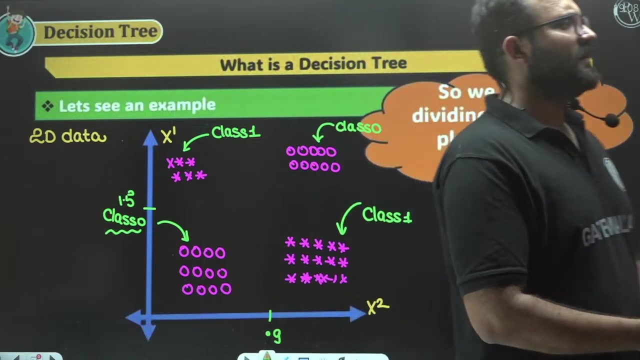 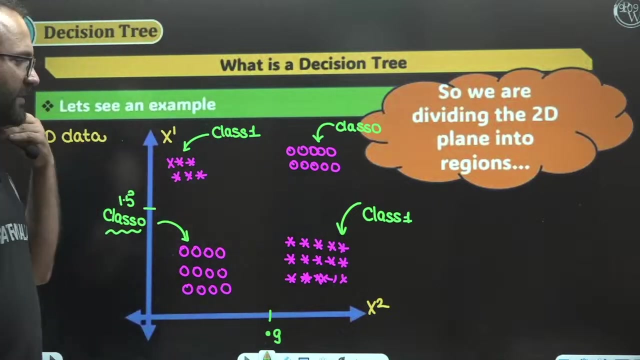 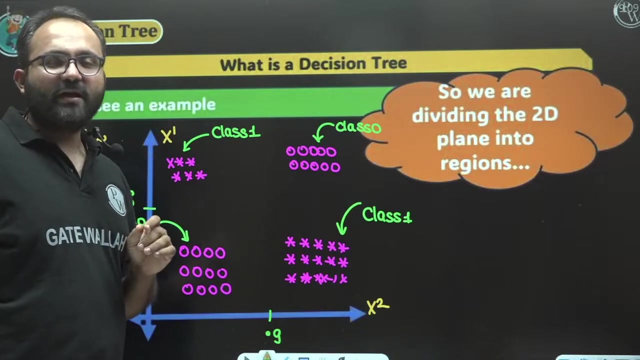 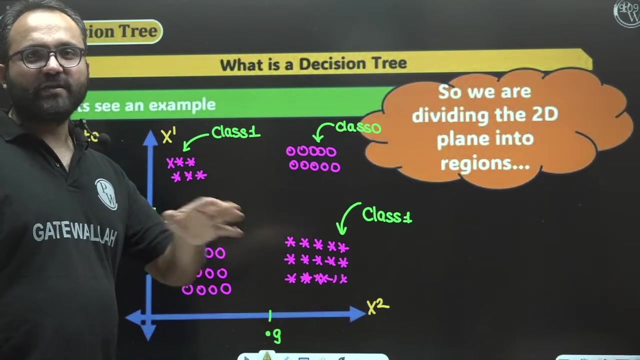 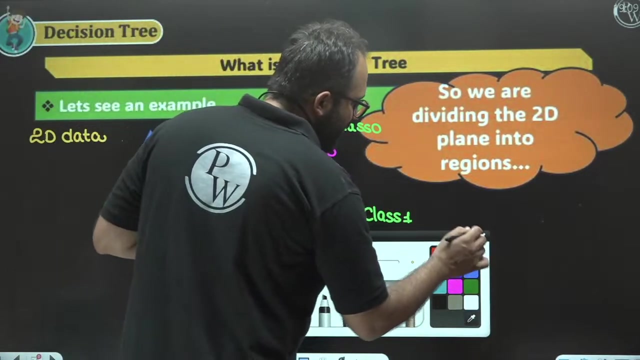 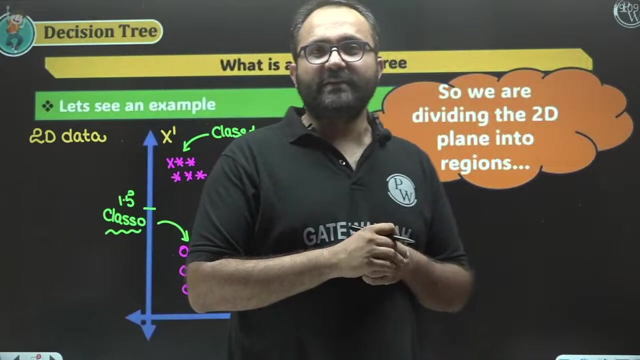 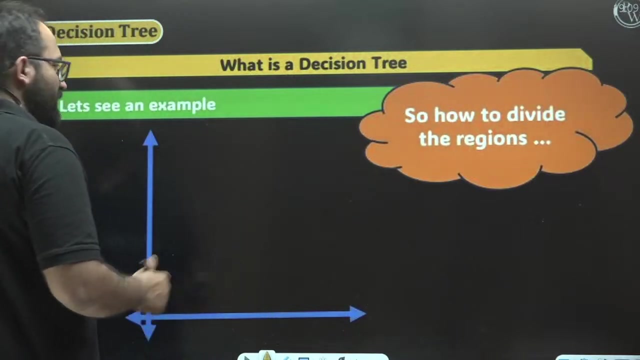 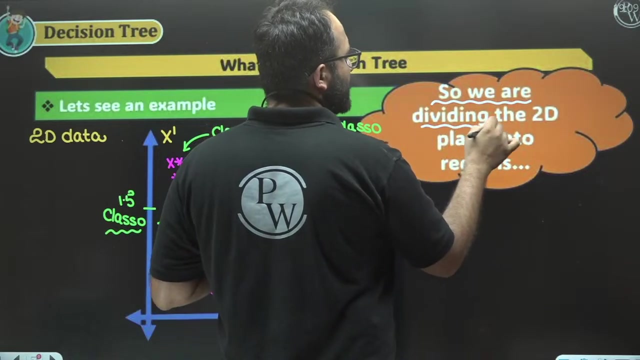 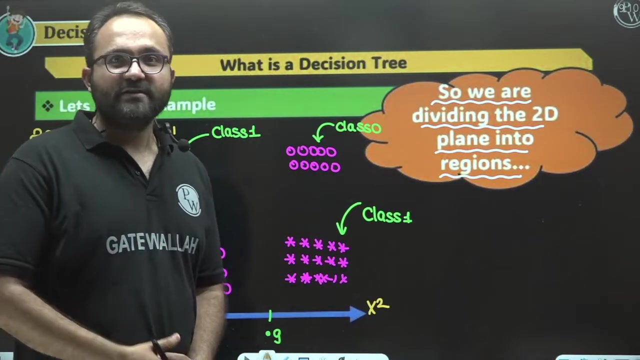 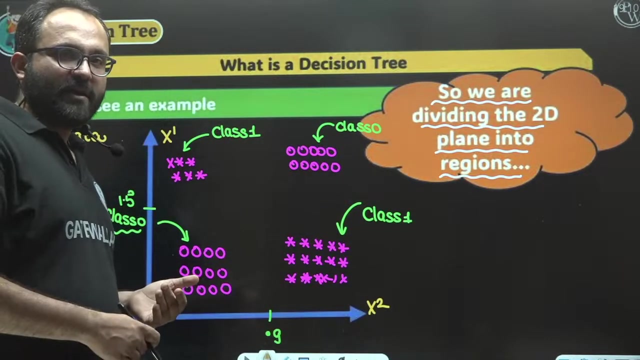 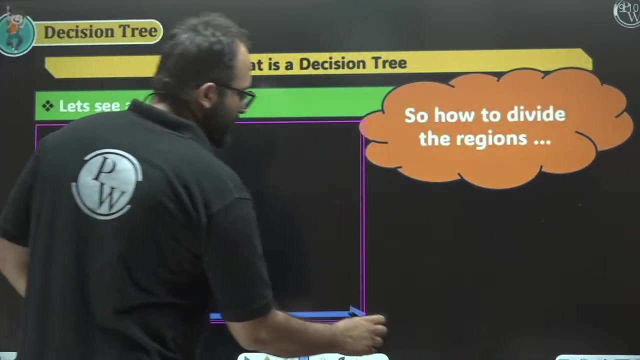 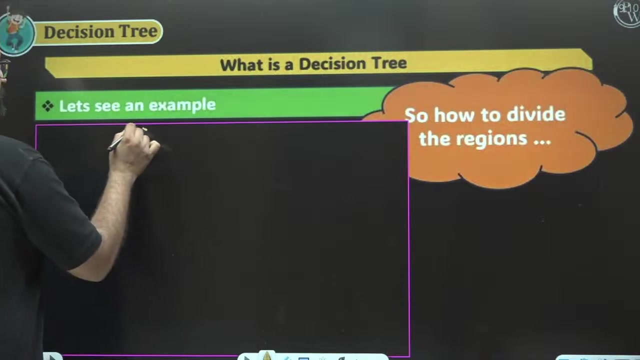 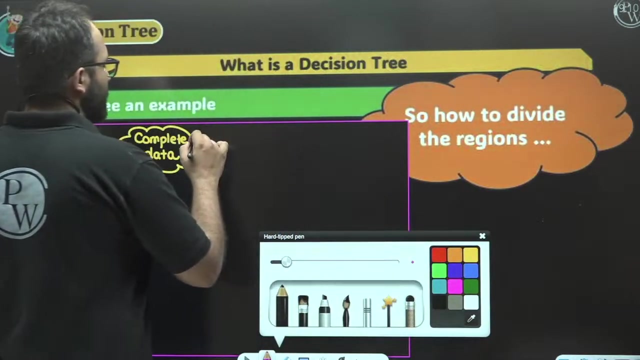 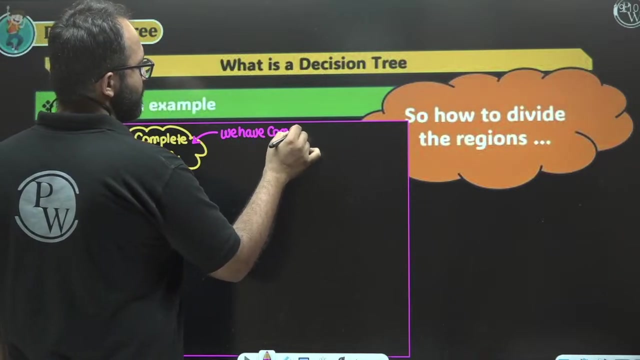 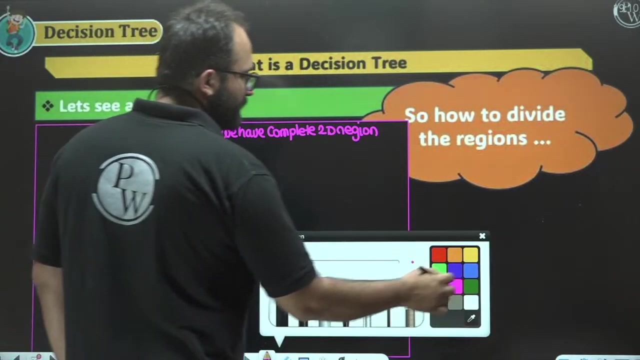 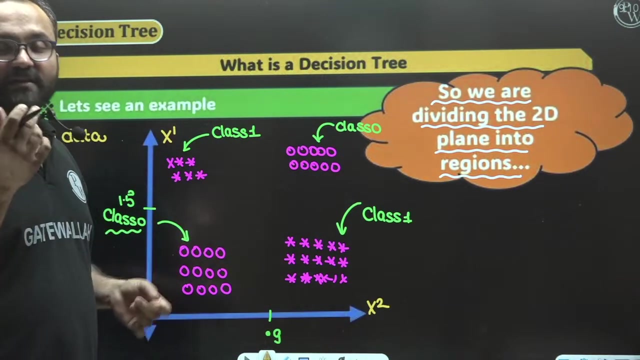 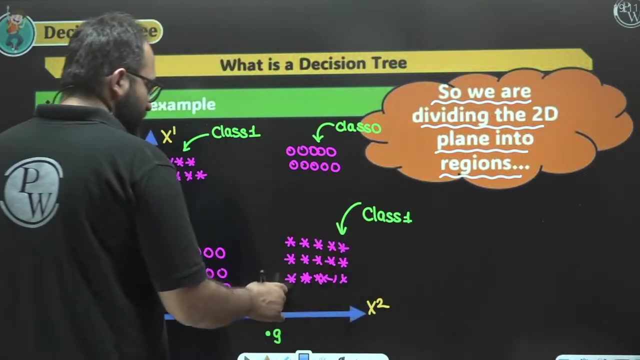 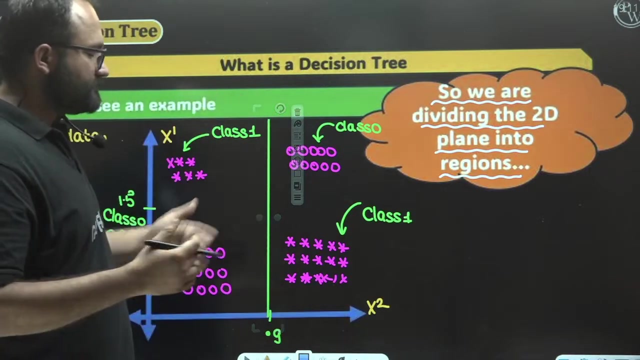 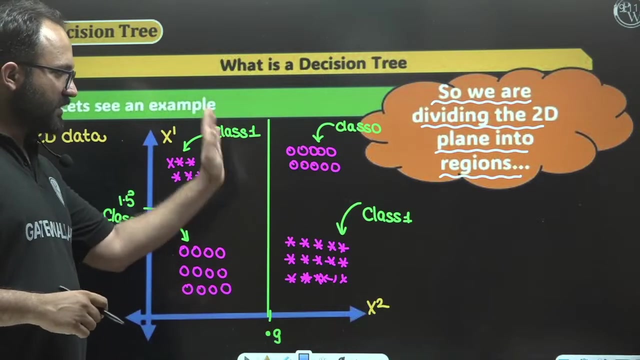 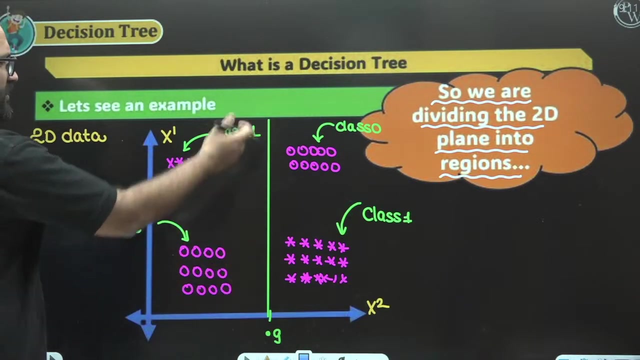 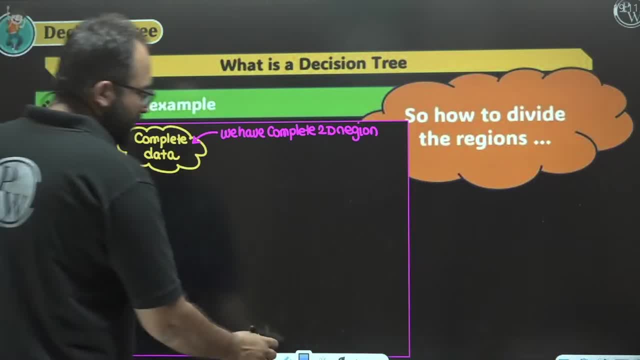 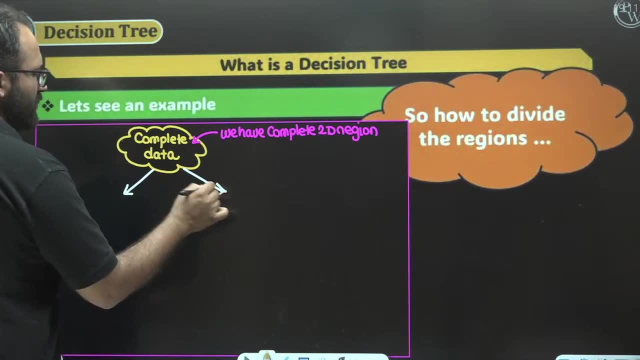 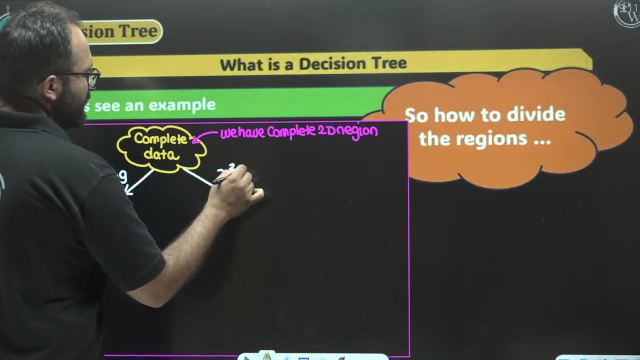 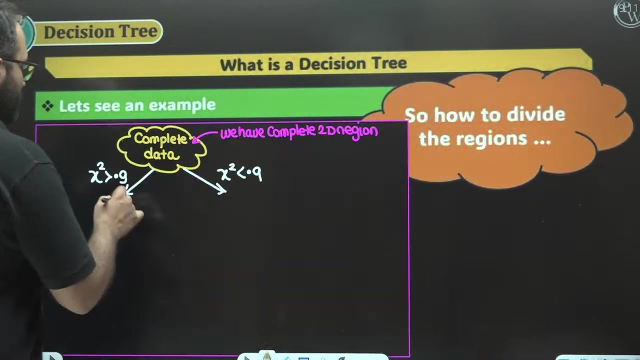 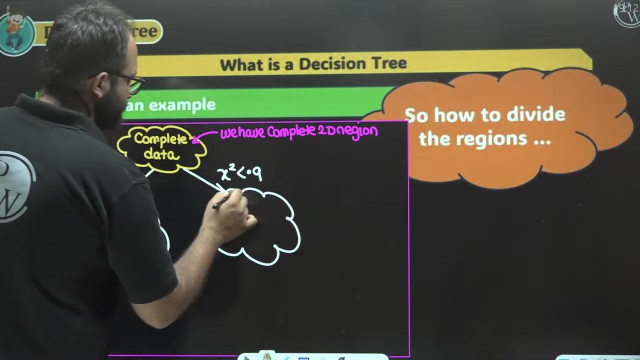 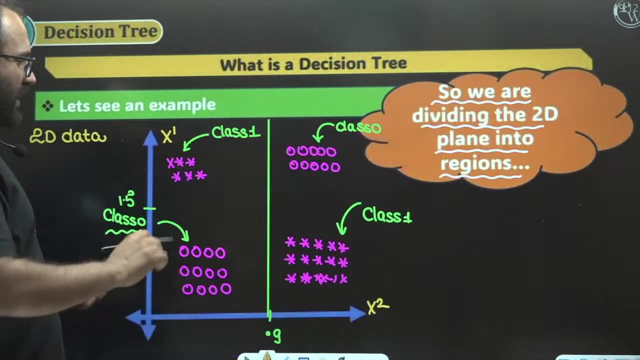 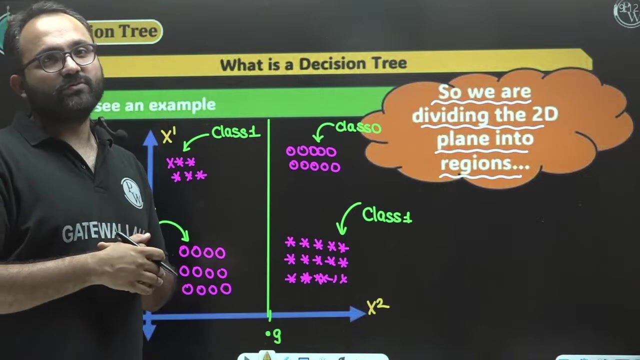 Thank you for watching. Thank you for watching. Now, what will you do? now? is the matter completely clear to you? that is, we want to find a region that is homogeneous. we want to find such a region that is homogeneous. homogeneous means: 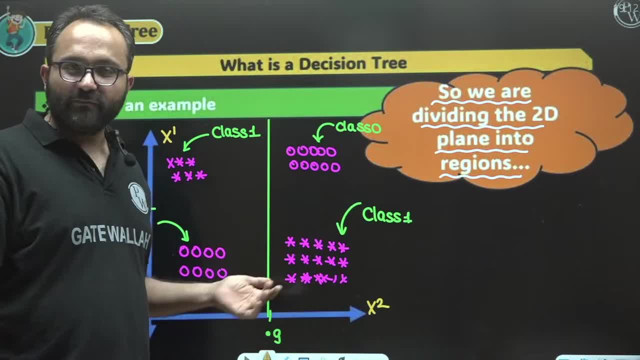 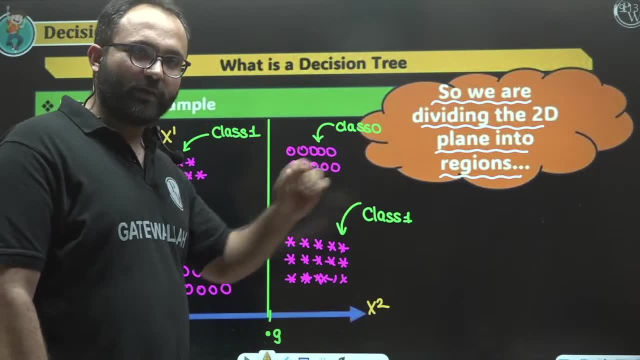 in which all the points are of the same category. so did we get that region? we have not got that region yet. then you will say that now this region has been found, which is not homogeneous. now I will use that word. don't worry, ok, we are going to see it now. so this region is. 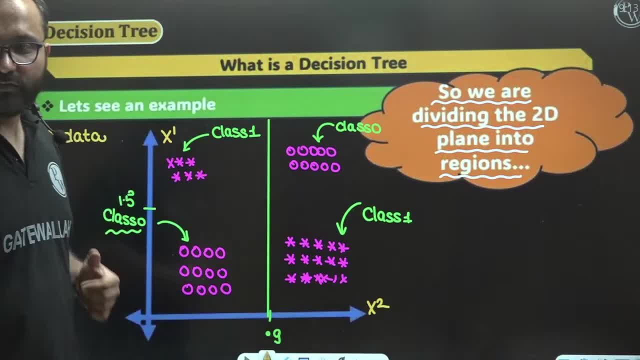 found which is not homogeneous. here, both class 0 and class 1 have points. similarly, this region has been found where class 0 and class 1 are both points, but these two regions are not homogeneous. so, friends, where will we break it to make it homogeneous? now you? 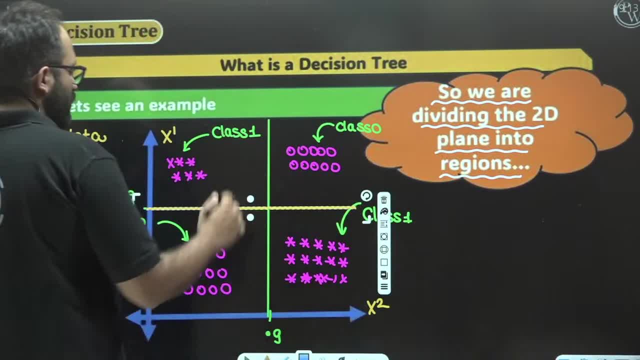 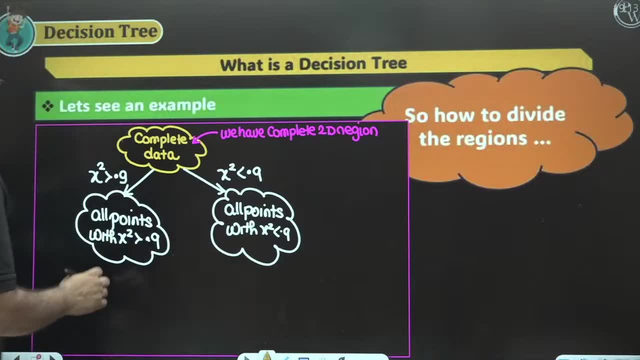 will say, sir, it is very simple, we will break it here. we can do it a little up and down too, but where we will break it, we will break it to 1.5. now you see, friends, so here you have first brought these points. 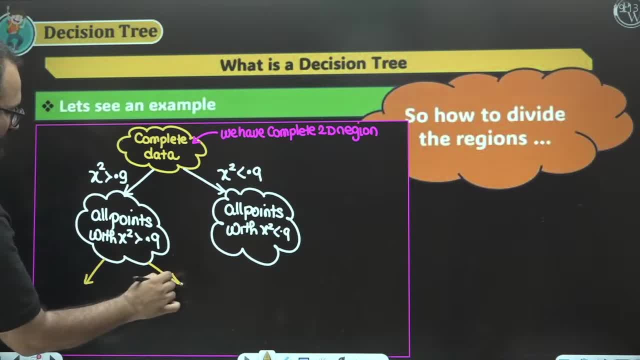 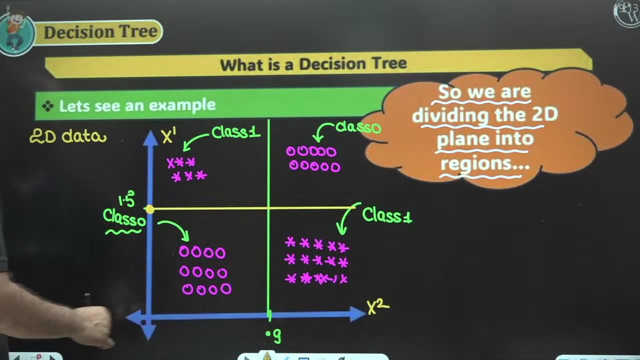 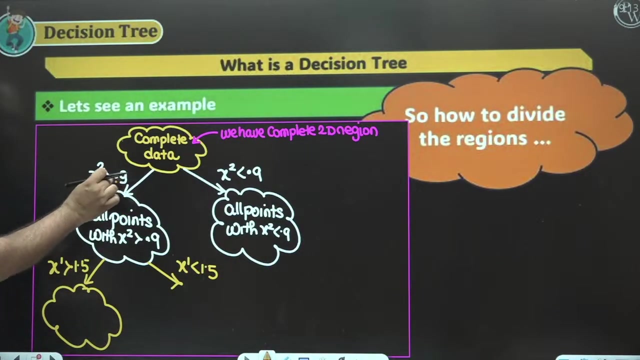 now you will break it further in two regions. one will come first, dimension greater than 1.5 and one dimension less than 1.5. now see, friends, did you get homogeneous region? yes, you will see, friends. the region you have got here is x greater than 0.9 and x1 greater. 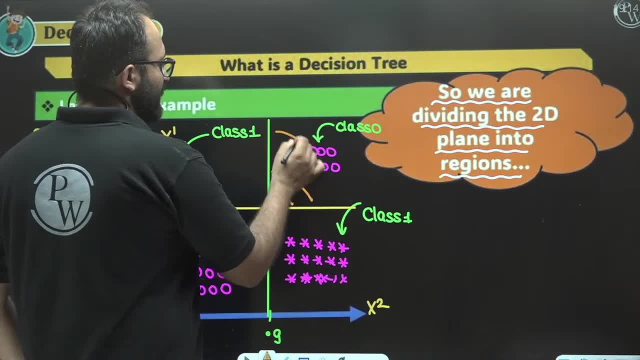 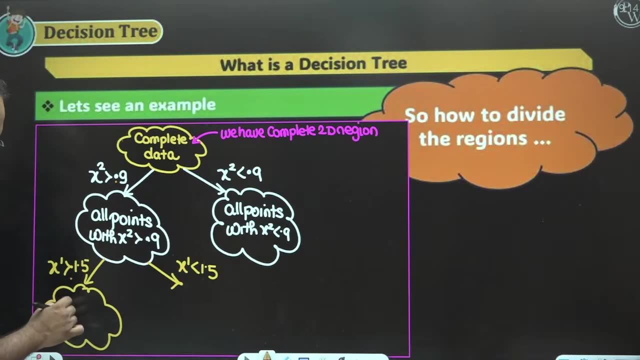 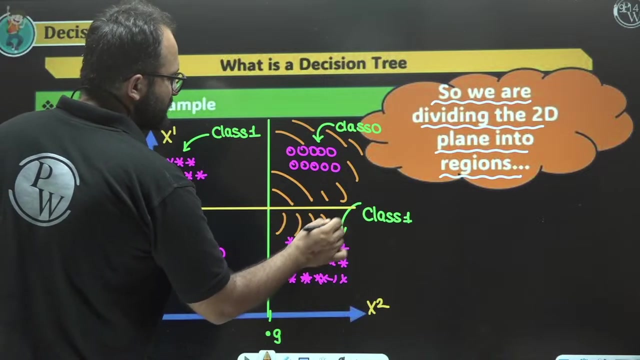 than 1.5 means this region. you have got this region here, okay. you have got orange region, okay. or you can say you will get class 0 points here. class 0 points, you will get here, similarly, x1 less than 1.5. so that is the region below where x2 is greater than 0.9 and x1 is less than 1.5. so you will. 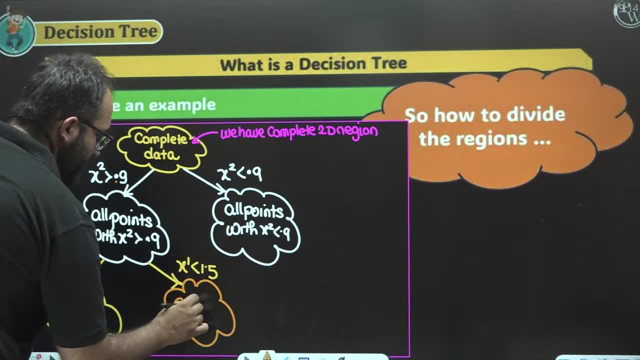 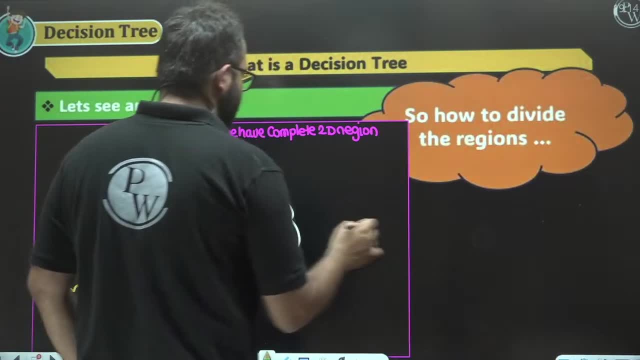 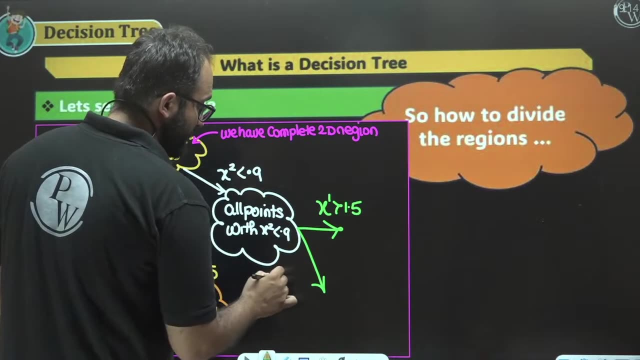 get class 1 points. similarly, we can break this too in two parts. one is x1- greater than 1.5 and one is x1- less than 1.5. so greater than 1.5, you can see that this region will come further. 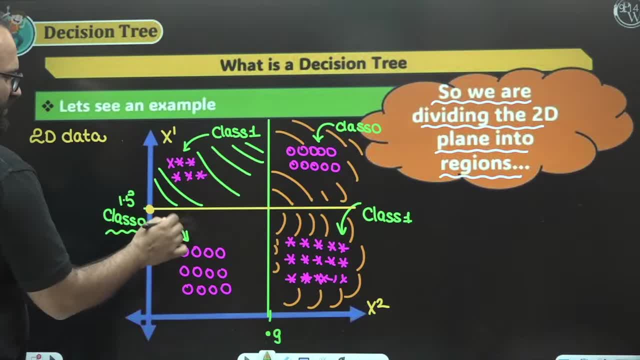 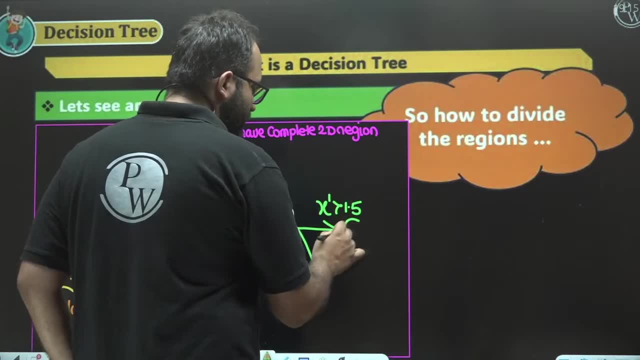 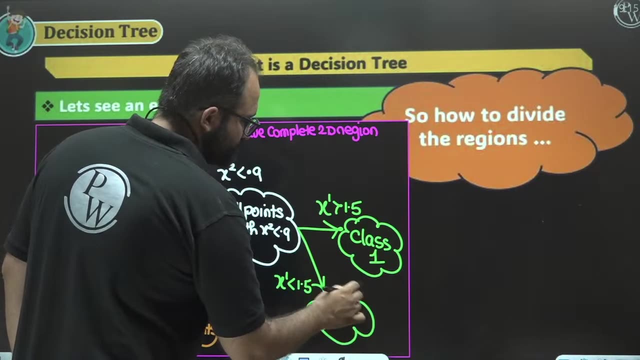 region which is of class 1 and this one is of class 0,. first of all, tell us who understood this. we are breaking in regions. who understood this quickly? tell us who understood this quickly. how many of you are able to understand this, that what we have done here we have. 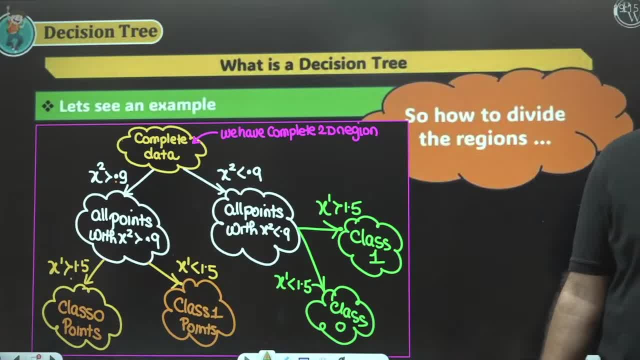 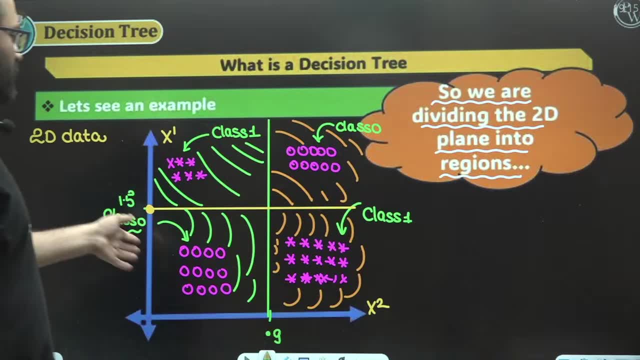 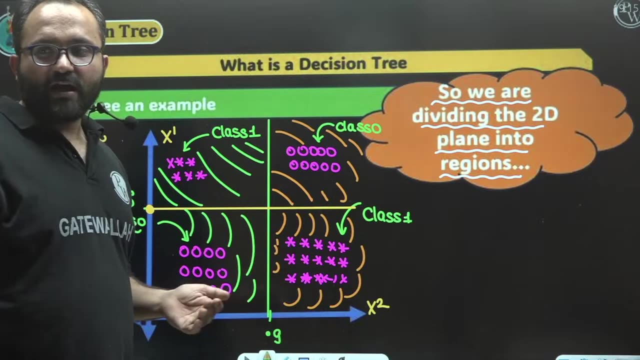 broken it in regions first of all. we have broken it in regions. we have broken it in regions first of all. we have divided it based on x2, so you can see this one region is one region, but we have to divide further because the homogeneity, or homogeneous region, 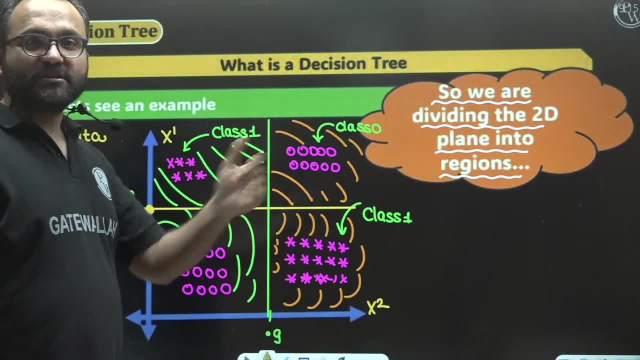 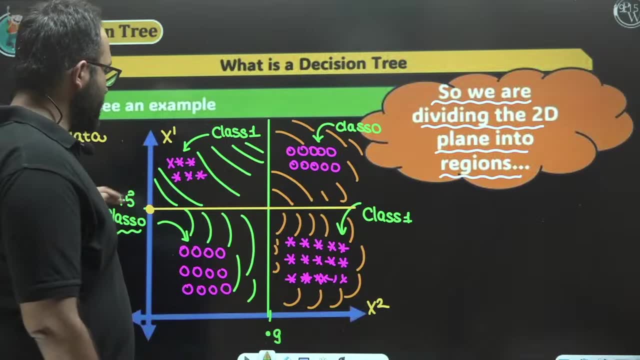 is not made. homogeneous means such a region where mainly points of class 0 and class 1 are there. so we have broken it here. so we got these 4 regions which you can see here. here we have these 4 regions, but where are the points of class 1 and class 2, we had 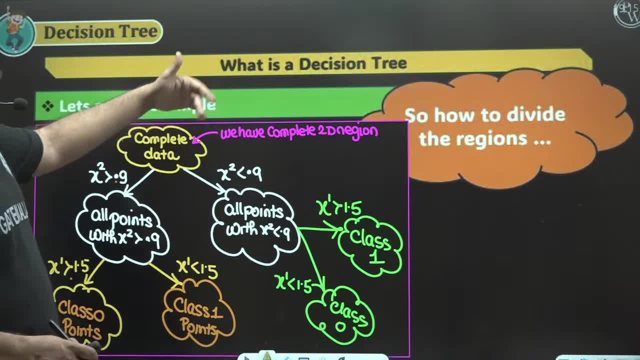 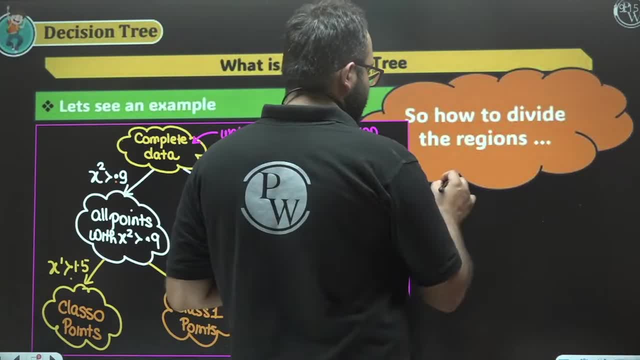 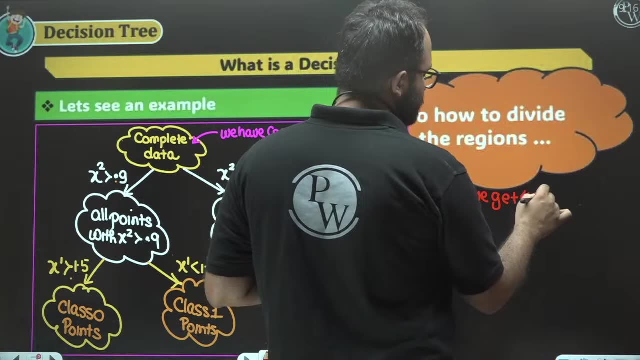 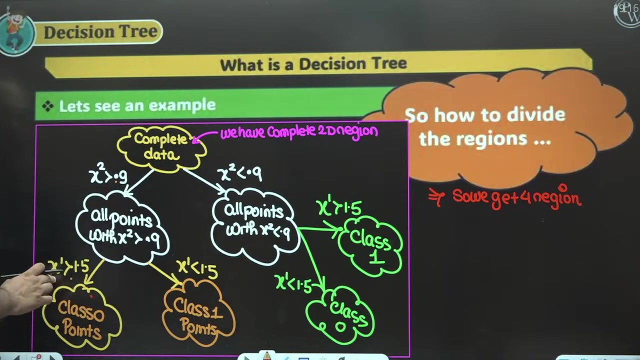 So this is our decision tree, which we can easily create. So we get four regions. We have created four regions. You can see the four regions: The region here is x1 greater than 1.5 and x2 greater than 0.9. Here is x1 less than 1.5 and x2 greater than 0.9. 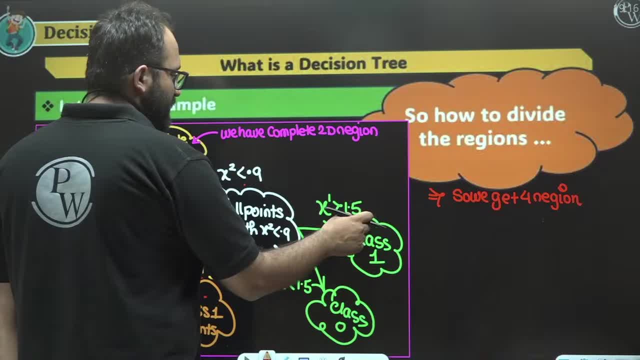 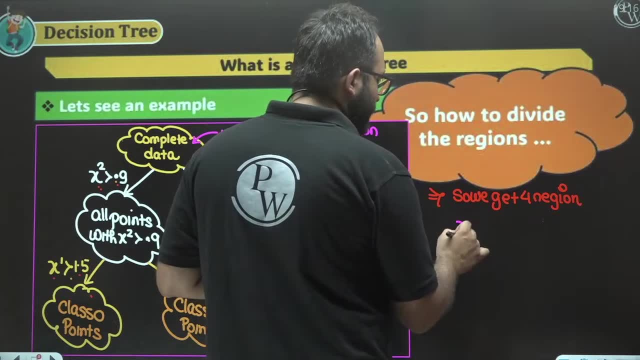 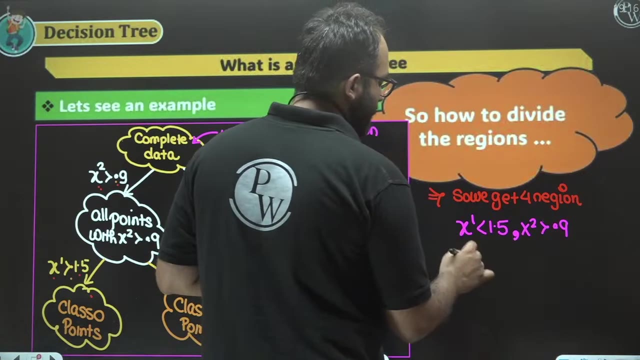 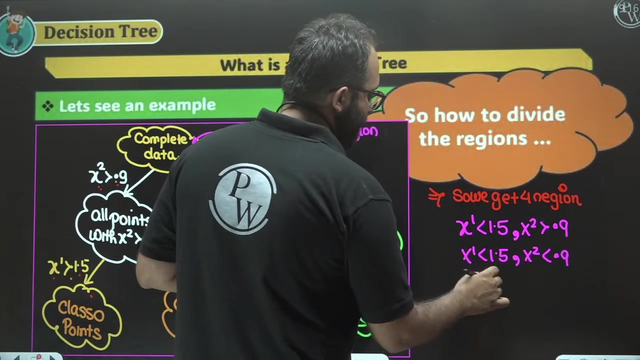 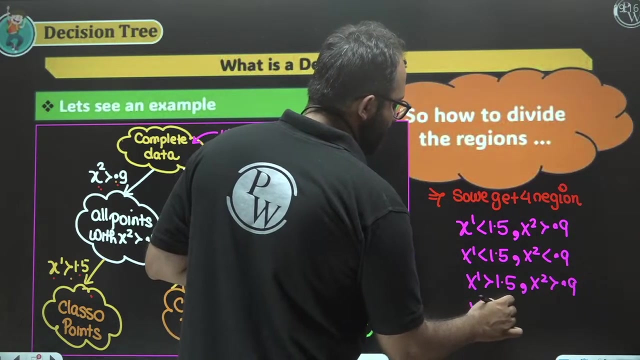 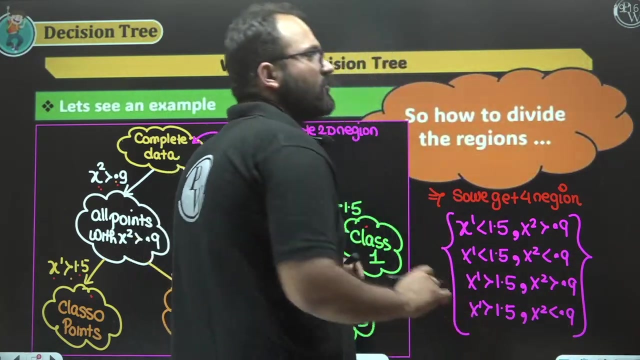 Here is x2 less than 0.9 and x1 greater than 1.5, x2 less than 0.9 and x1 less than 1.5. So we have created four regions. So we have created four regions. Now can we easily tell the class of any new point. 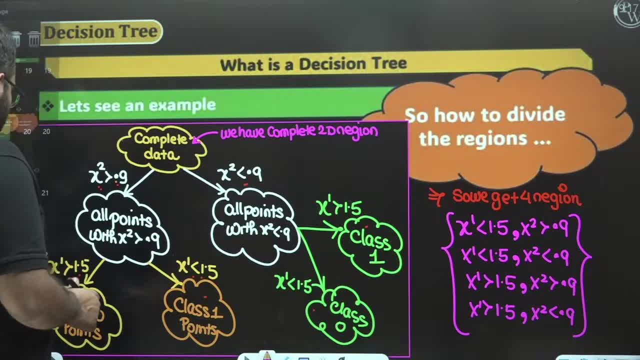 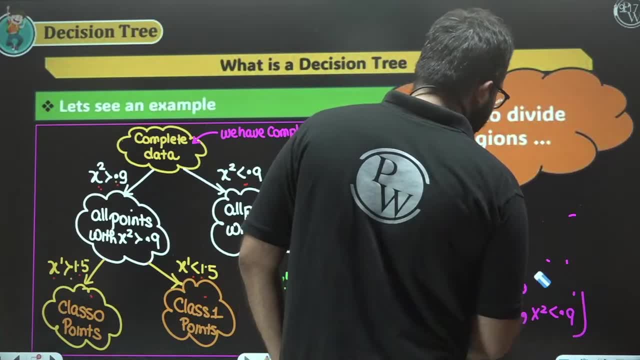 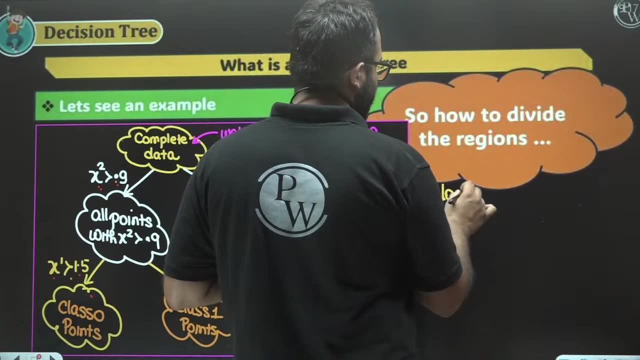 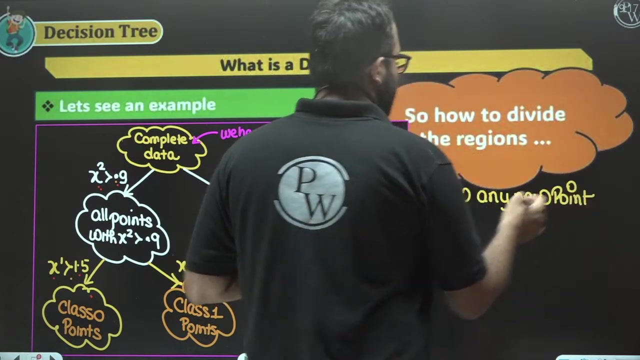 Now any new point and we can easily find out. Now for any new point, we can easily find out its class. Now for any new point, we can easily find out its class. Now for any new point, we can easily find out its class, Suppose any new point is there. 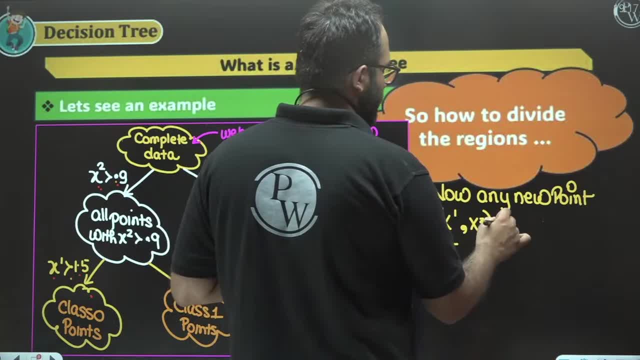 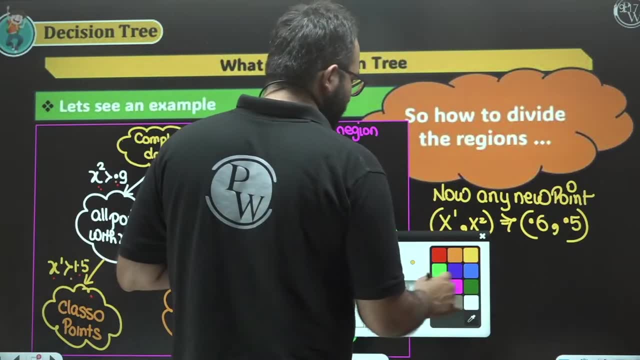 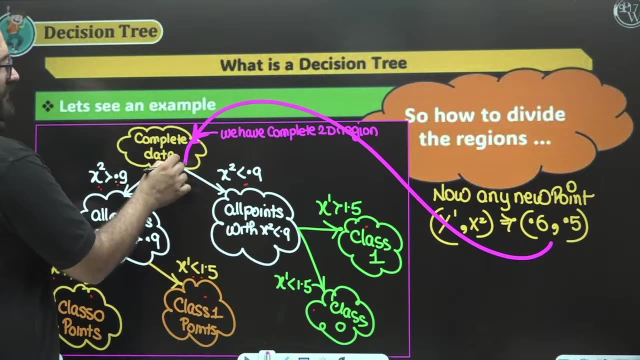 Suppose any new point is there, Suppose this is our point. So first of all, what you will do, First of all you will take this point and reach here, Then you will see here. So here x2 is 0.5, So means it will come in the region less than 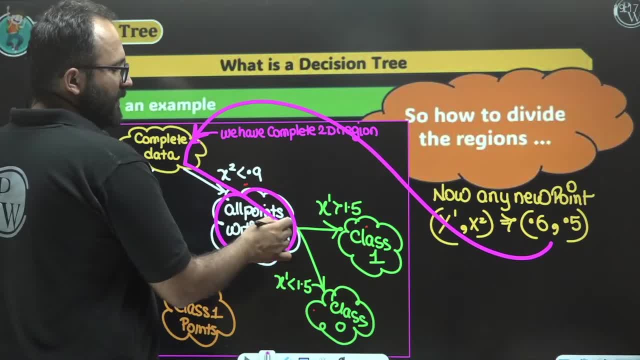 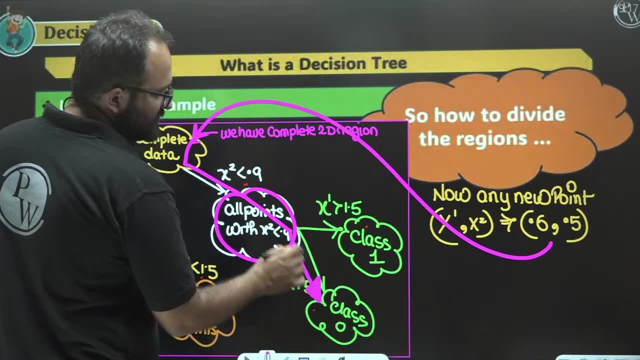 So here it will come in here Now. here you will see That x1 is 0.6 Means it is less than 1.5. So here it will come, So you can see whenever it is coming here. So it is entering in this box. In this box because class 0 is written. 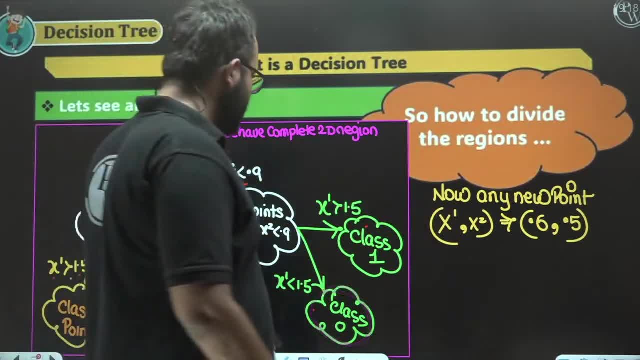 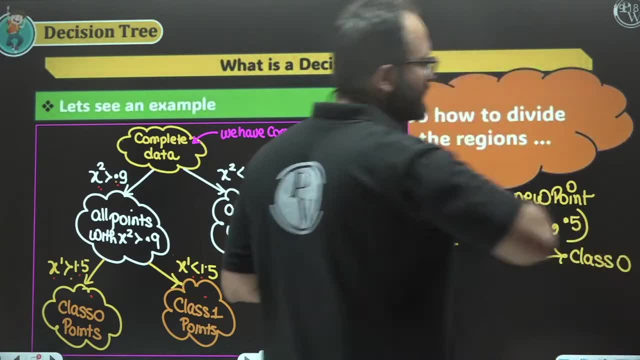 Means, friends, what we will give it. It will be given the tag of class 0, that its predicted is class 0. why I will tell you again. first of all, you take this and reach here. you see, x2 is greater than 0.5, 0.9 and less than 0.9. 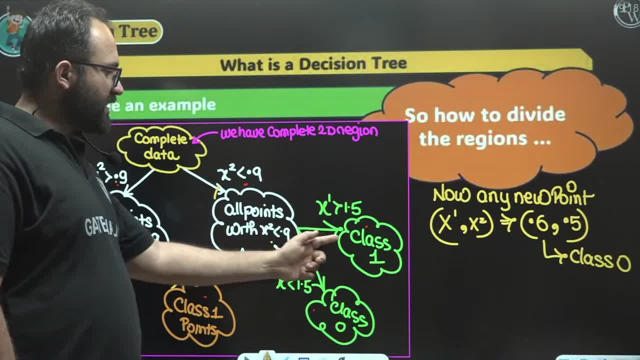 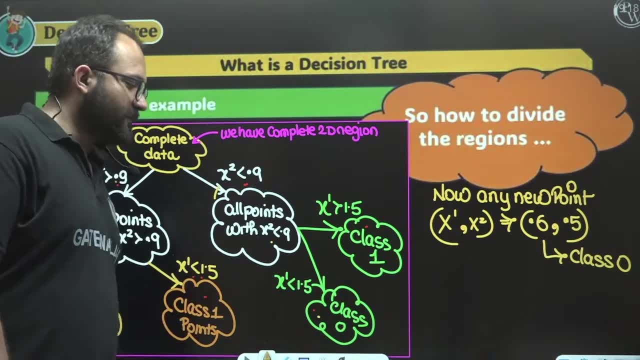 so less than 0.9 will come here, then after reaching here. if it is less than 1.5, then it will reach here. so you can see very easily that it will sit in this box and class 0 is happening here. ok, in this way we learnt that. 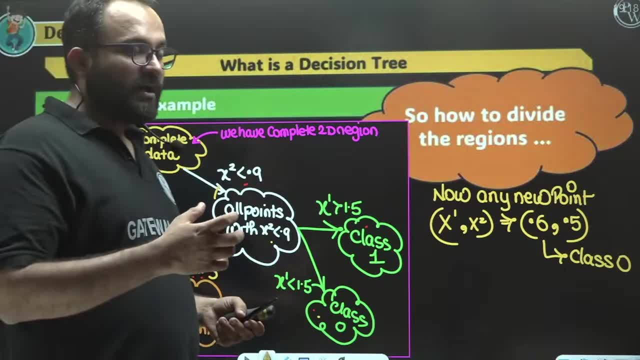 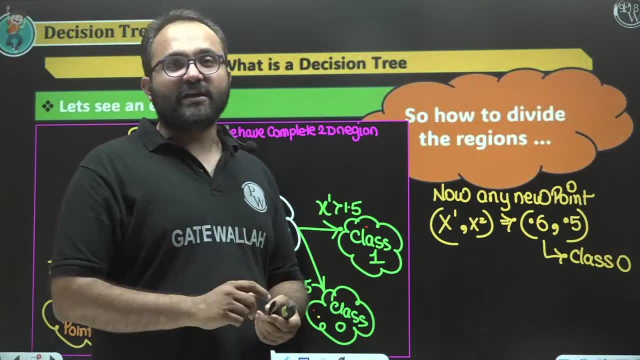 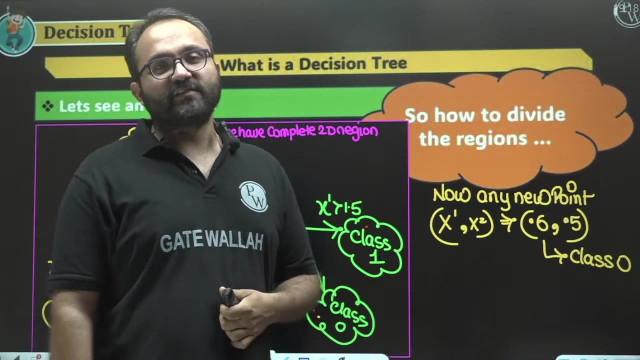 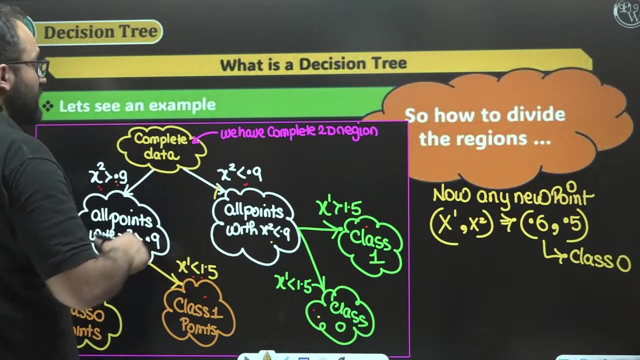 in decision tree. we break our region, we break our 2D plane or whatever dimension plane we have, whatever dimension region we have, we break it in small, small regions. we break it in small, small regions. ok, so now here a question arises, that many questions arise. many questions can arise here. 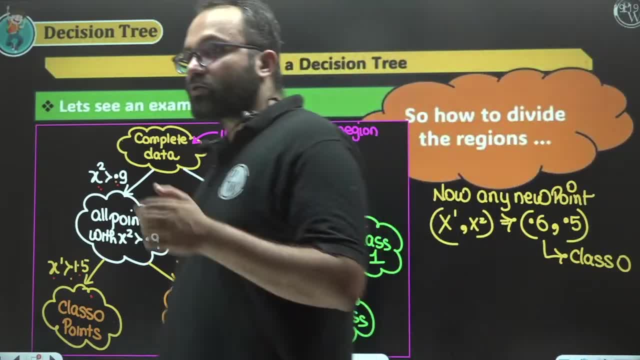 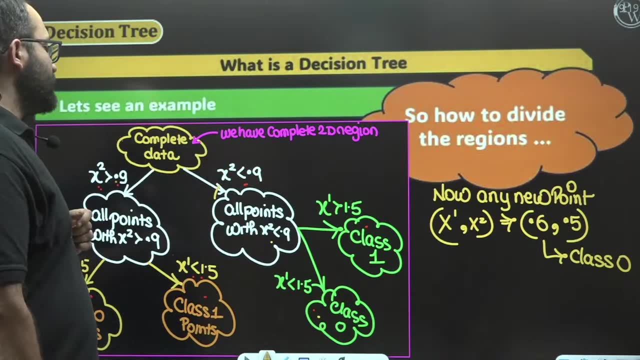 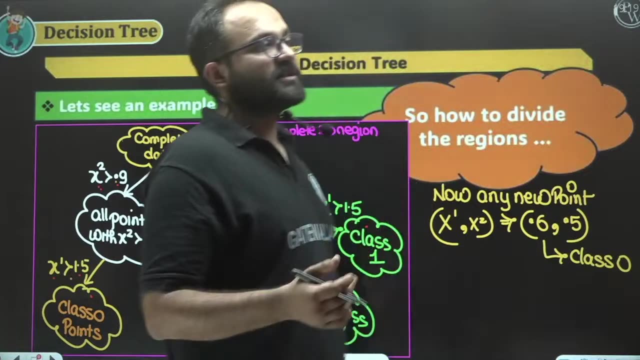 that, sir, how we will divide. ok, which dimension to choose, because you will say, sir, why did you choose x2 first? why didn't you choose x1 first? ok, in this way we can have many dimensions. so there can be a number of questions, and if we have to answer them, 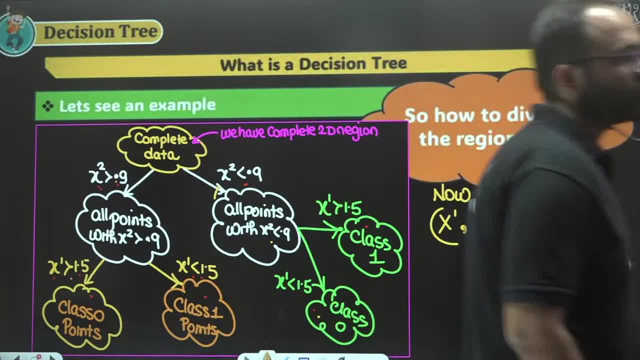 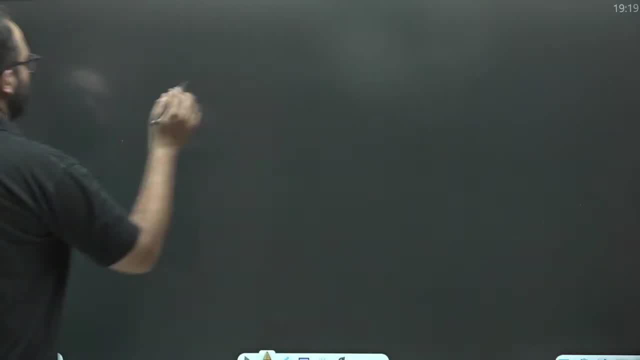 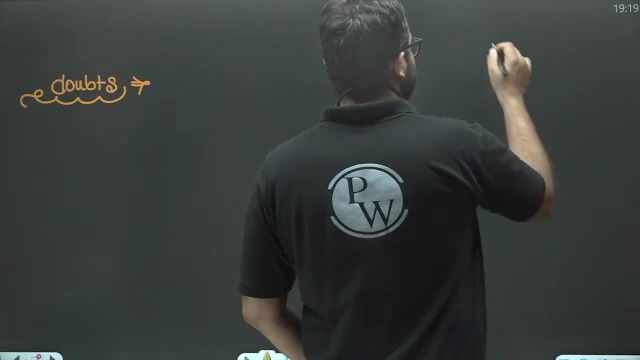 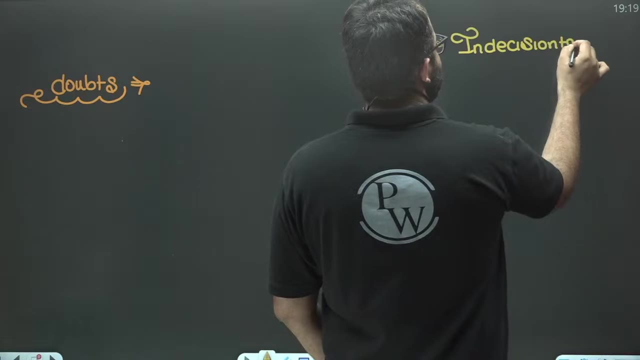 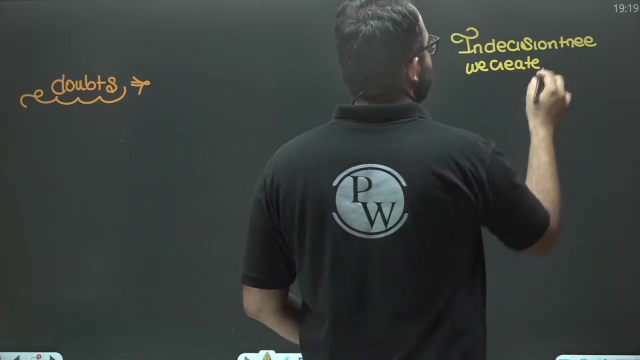 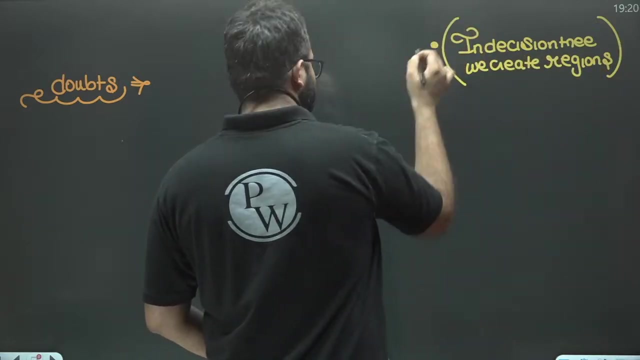 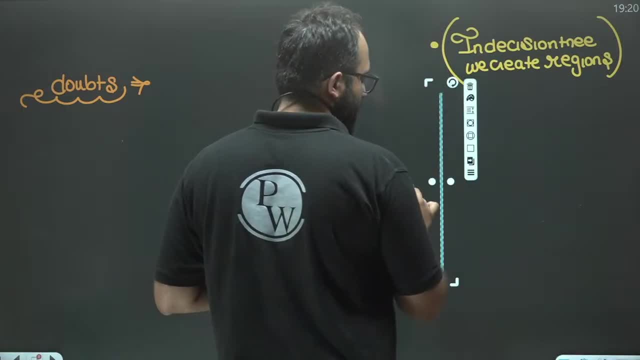 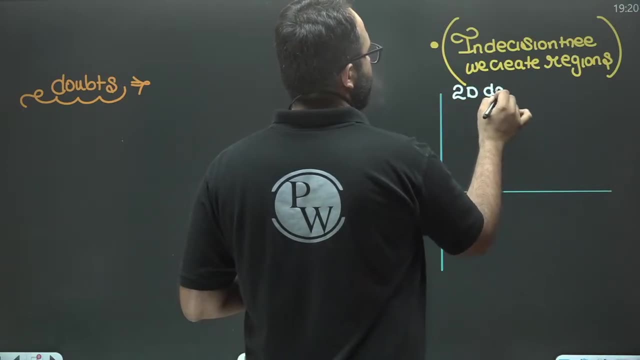 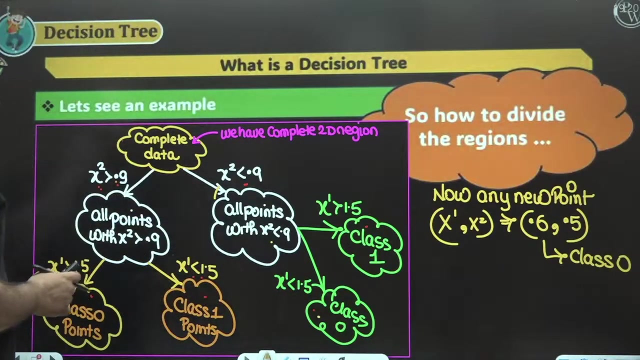 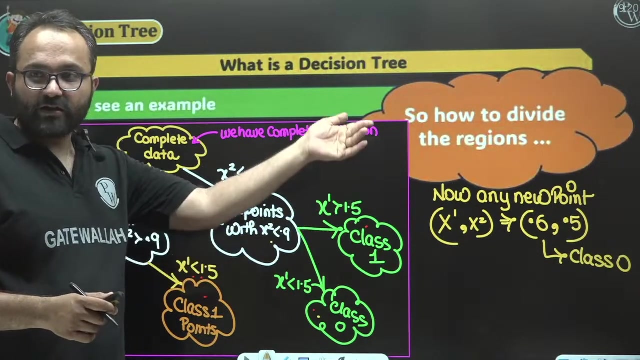 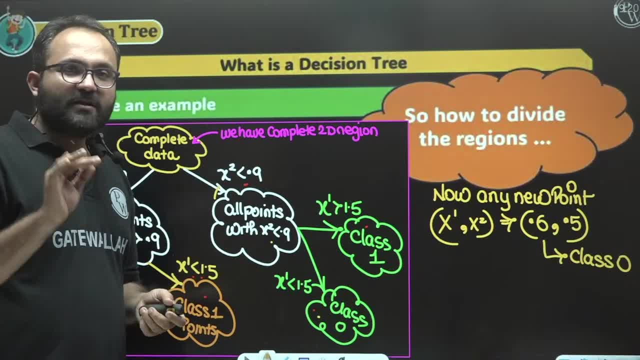 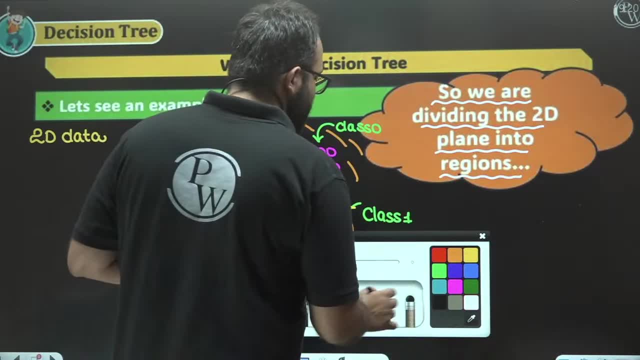 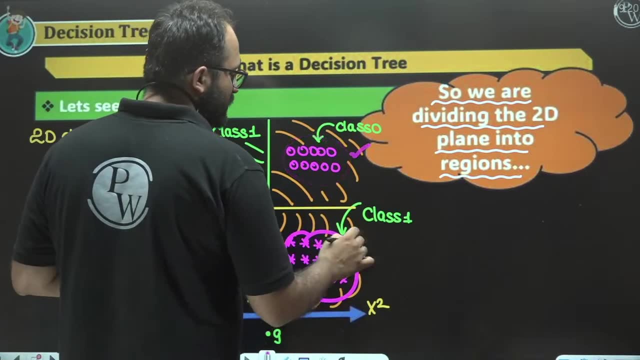 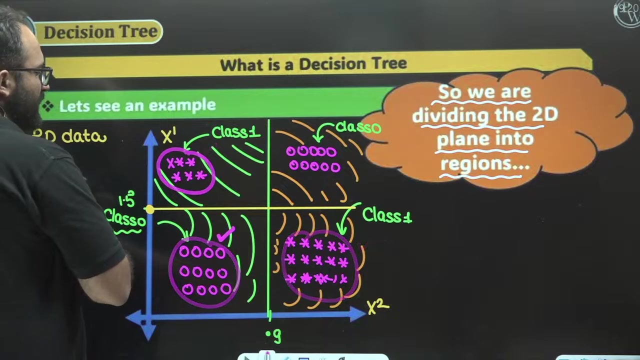 listen carefully, listen carefully, listen carefully Till your homogenous region is not created. So you can see till we want to break till. our homogenous regions are not created. But there is a problem in it. What is the problem? Let's see, See. 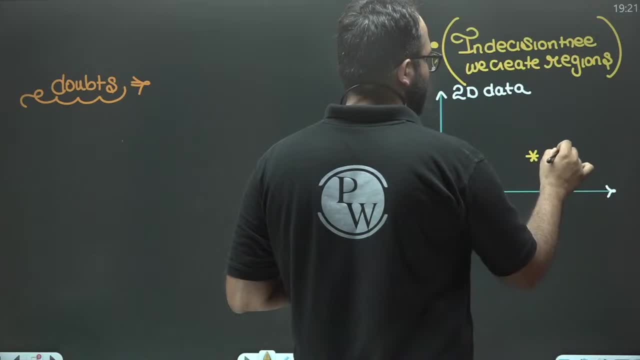 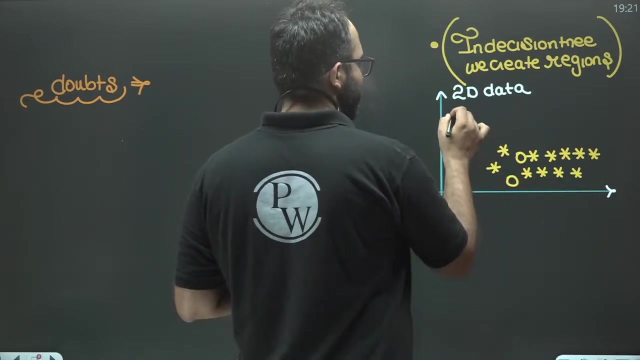 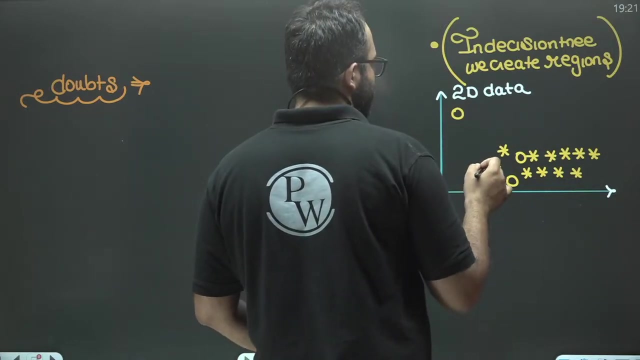 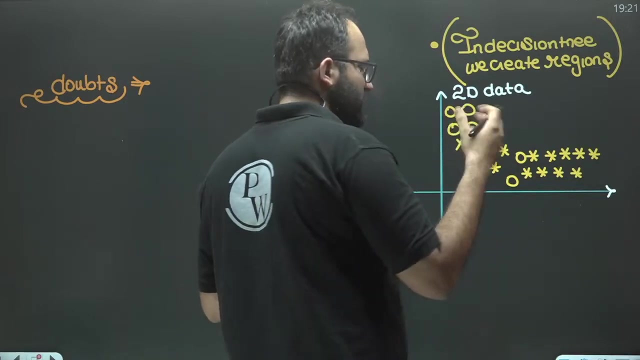 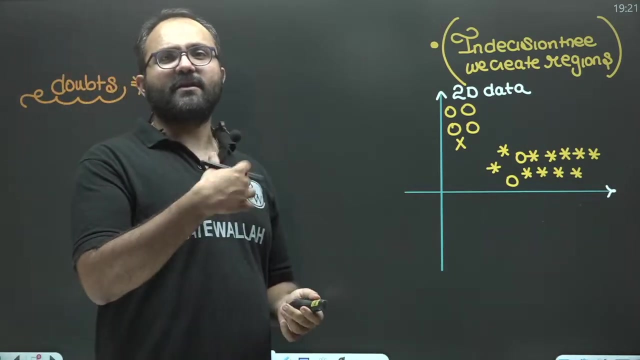 As I told you that we have some points like this. Assume that we have given some region like this. We have given some points like this. Now you will say that we will break in two regions And we will break till we don't get homogeneous regions. 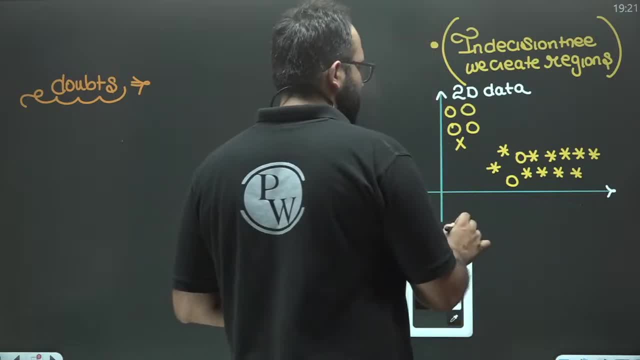 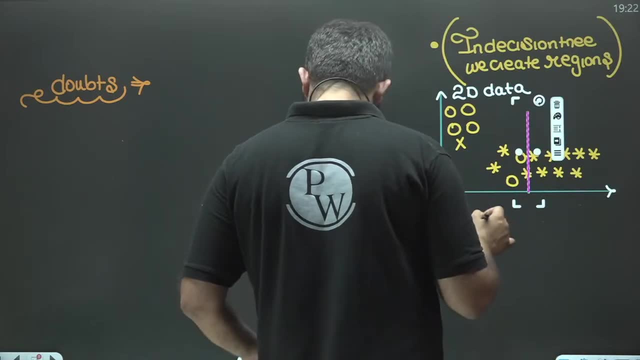 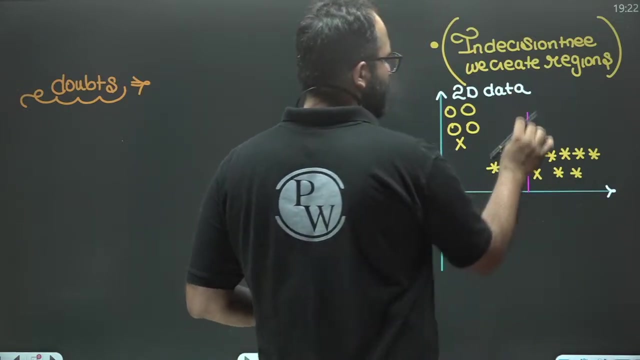 So there is no problem in breaking. You will say that first of all, we will do like this: We will break here at this point. We will break like this: I will remove this cross. Okay, Just for So you can see that we can create one region here. 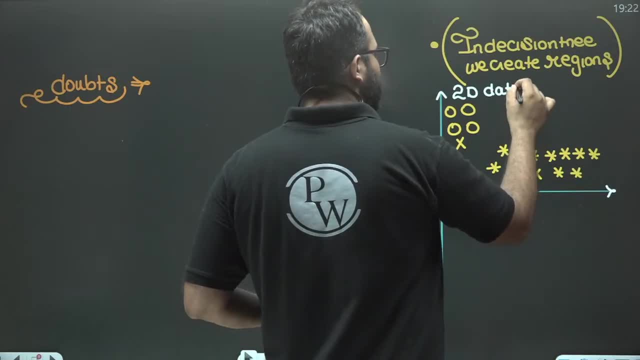 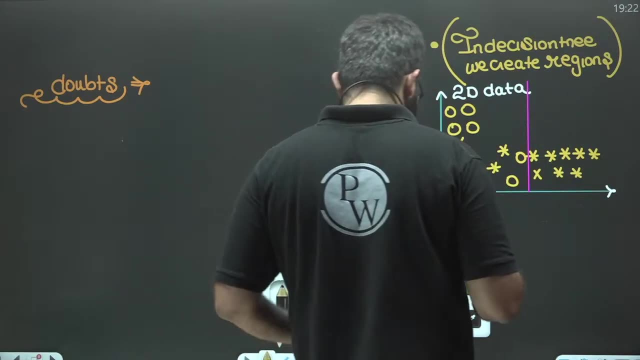 What kind of region will it be? Look carefully, We have created some such region. We have broken one here. We have broken it. like this: One region is created, So you will say that here it is homogeneous. I can see the whole region of class 1.. 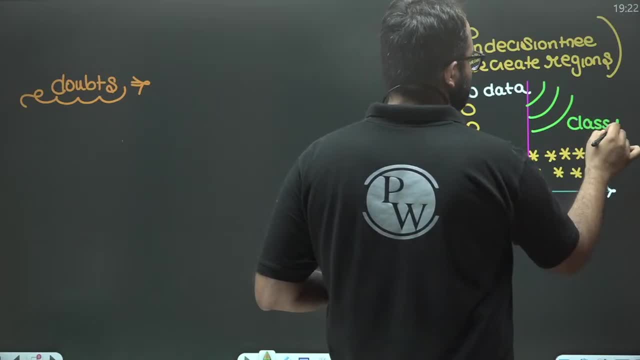 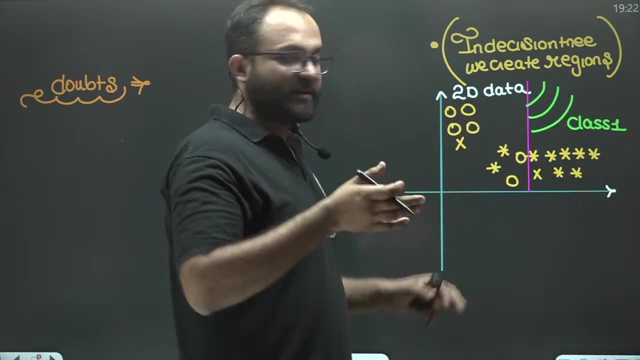 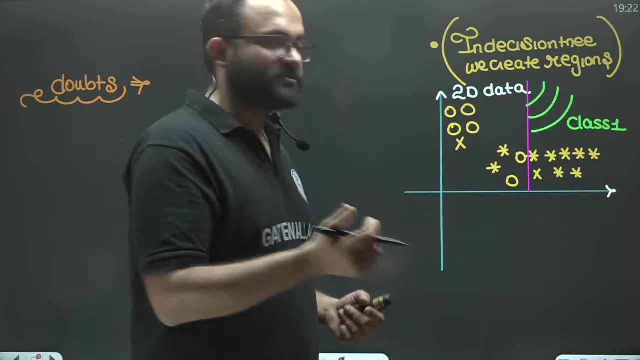 Okay, Now look at the second. Is there any problem in this? No, Because we can create only rectangular region. We can only create rectangular region Because the condition can be X2- greater than something or less than something. The second region which we can see is this: 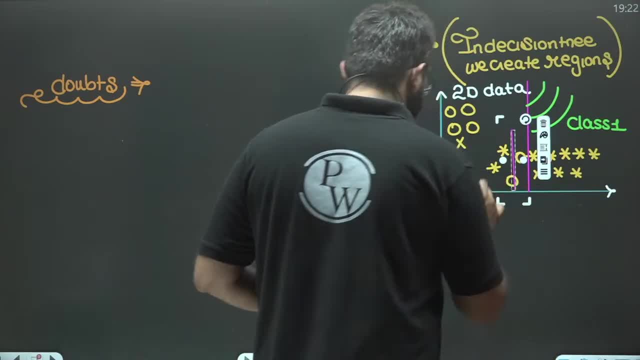 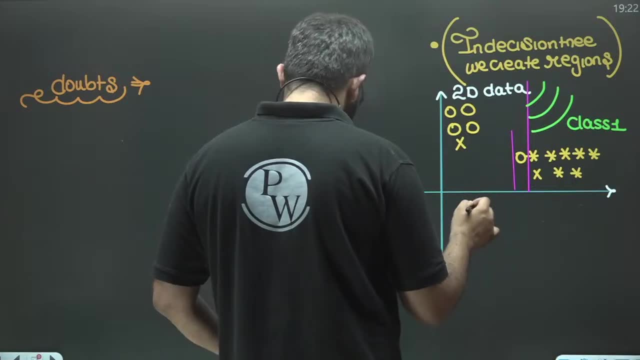 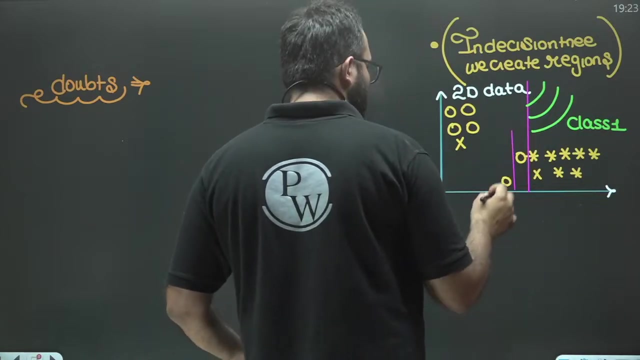 I will move this circle a little bit here. Now you will say that the second region which we can see is this, And If you want, then you can take it up. There is no problem in it Because there is no blockage over it. 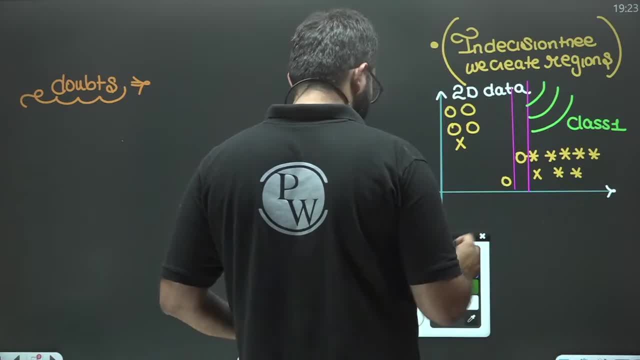 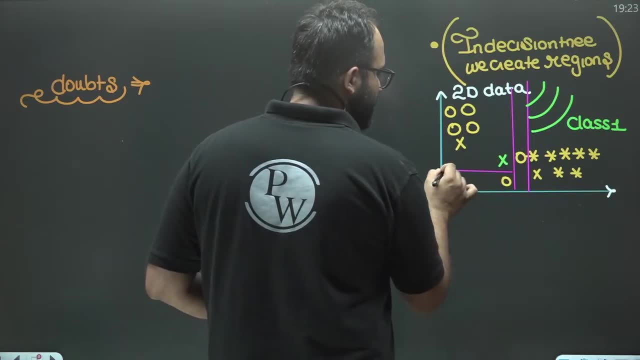 So there is no problem. The third region which is seen Here is a cross, Here is a circle. So you will say, sir, I can see this. We will call class 0 in this region. In this region, we will call class 1.. 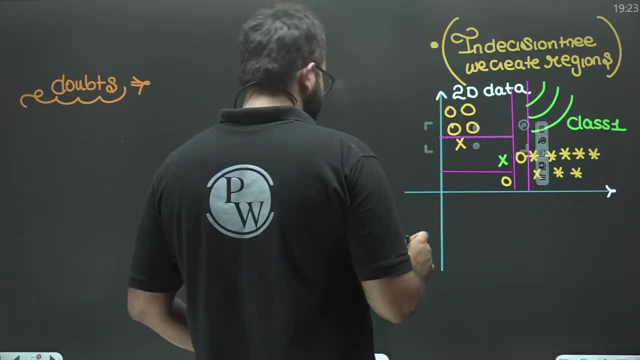 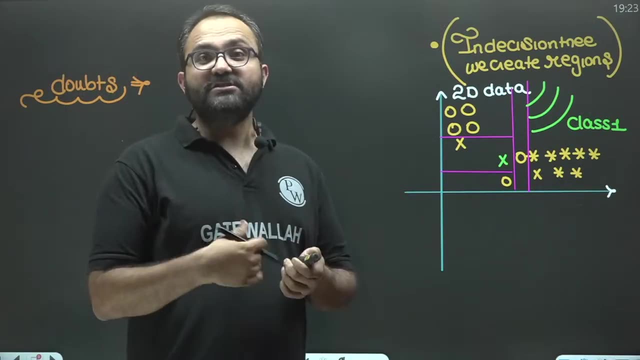 From here to here, And then we can create this whole region with this Yes, Yes, and then in this whole region we will call it class 1. in this way, it created region means if we see homogeneous regions, then in this way we will do breaking. 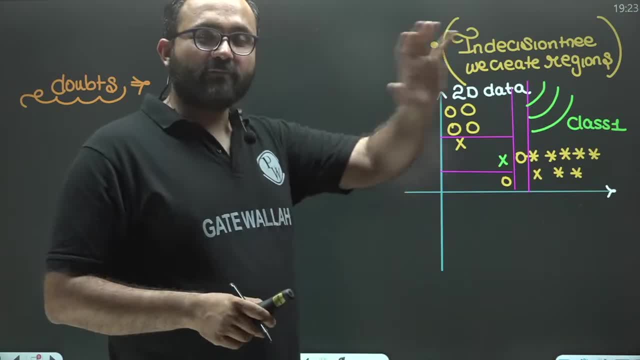 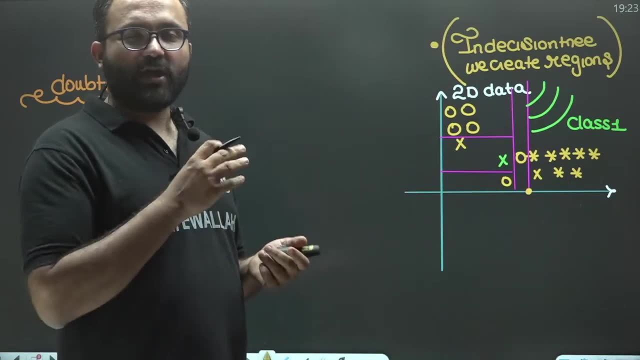 of our whole region. of our whole region, how you will say, sir? one region, because we have to create region only by doing greater than or less than we can create any region. we have two dimensions: by doing greater than or less than we can create any dimension. 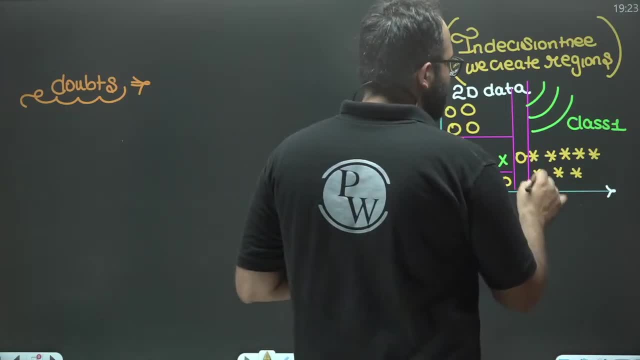 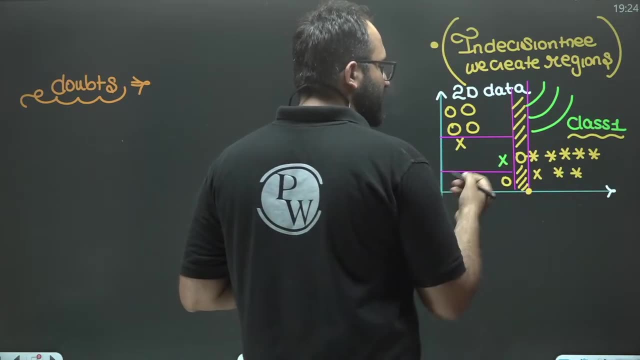 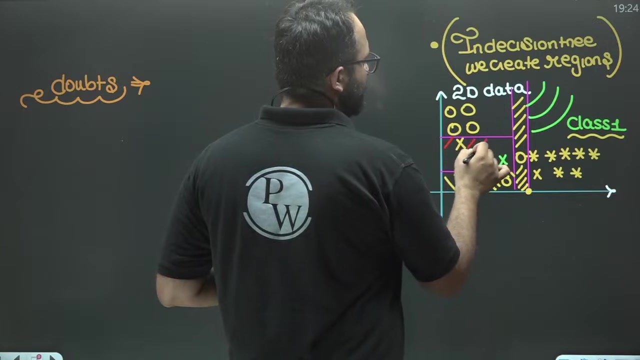 we can create any region so we can see. one region is here where we have class 1 points. second region is here where we have class 0 points. third region is here where class 0 points will be declared. fourth region is here where class 1 points will be declared. 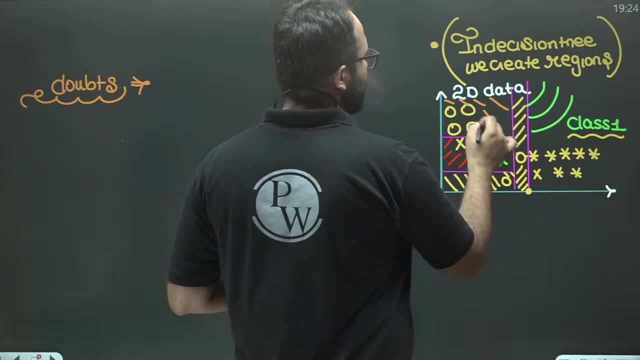 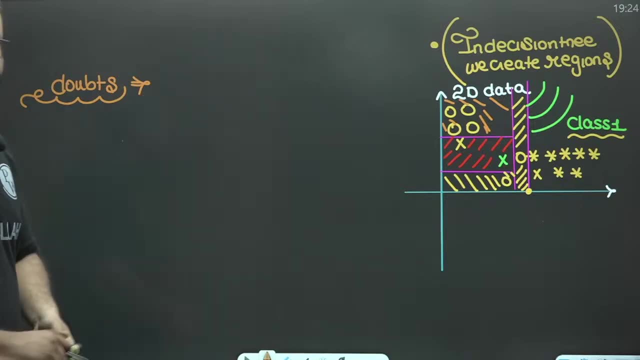 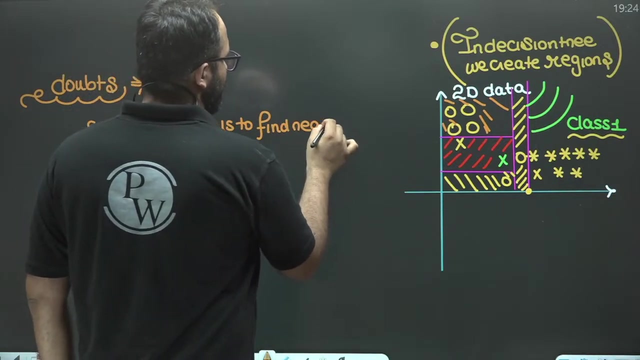 and one more region is here where class 0 region is. so in this way we can create many regions. but what do you think, what is our mechanism doing here? so if the target is to find the regions of homogeneous points, then the algorithm. you can see what the algorithm is trying to do. 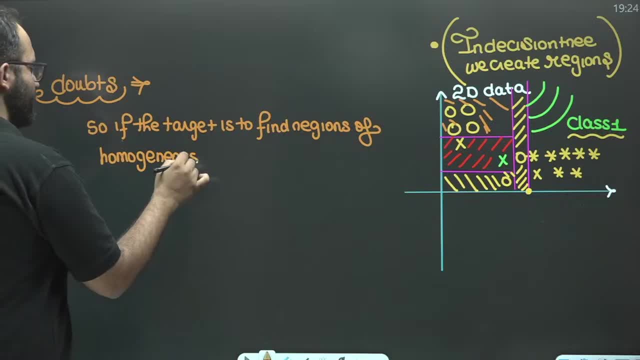 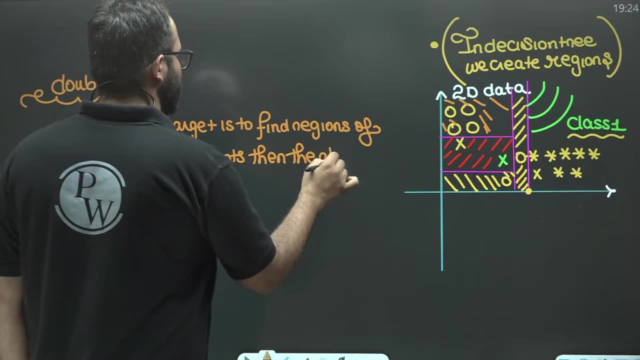 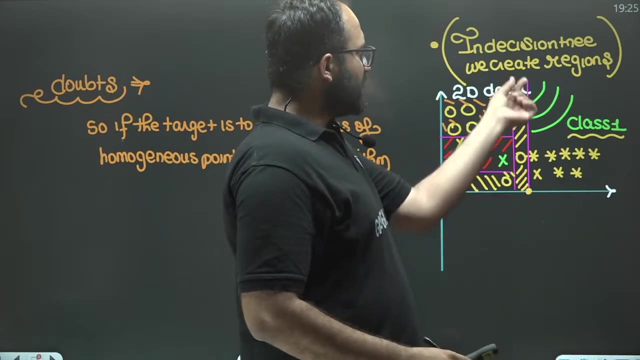 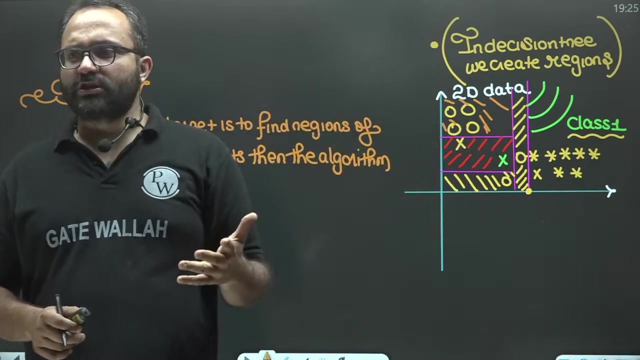 so if the target is to find the regions of homogeneous points, then the algorithm you can see is trying to create regions. here is become this rectangular region, there a this more, here, now this and this. so here what the algorithm is trying to do. here the algorithm is over fitting. 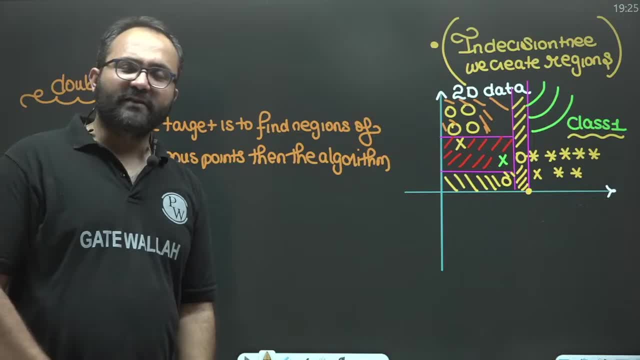 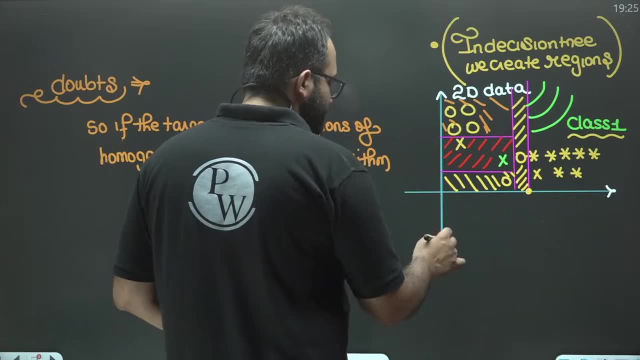 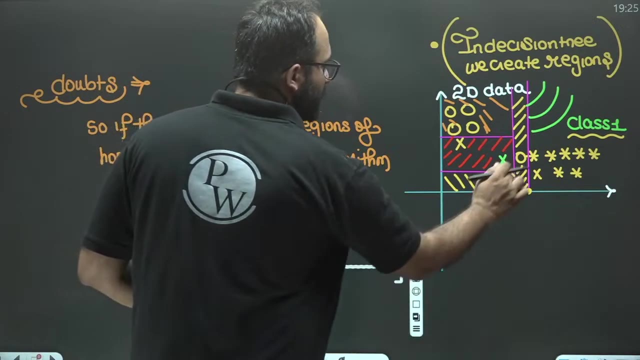 here the algorithm is over fitting. ok, then you may ask: how is it doing it? see, let me tell you here our algorithm is over fitting, because you can say that it is possible that these two circles are noisy points. this can be the thing, right, suppose this is it. 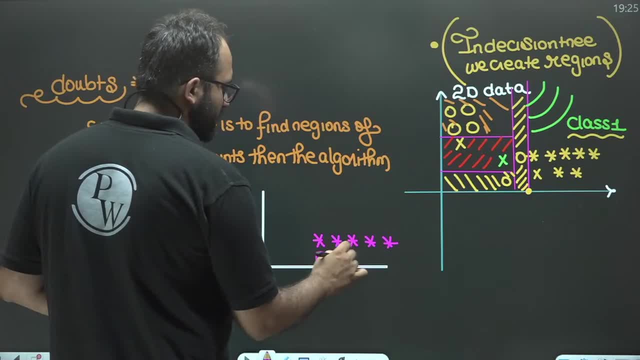 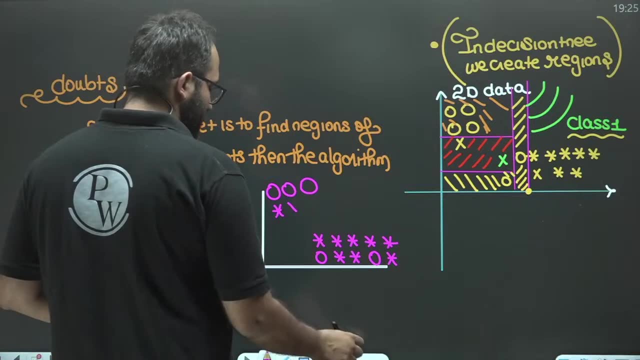 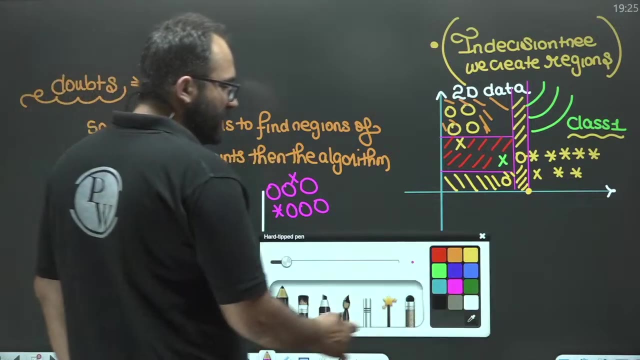 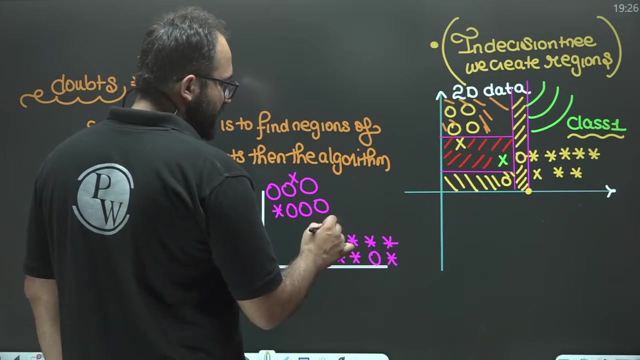 here is a circle. here is also a circle. here are round, round, round points. suppose we have something like this. so if we over fit it, then how will we make the regions? as we need homogenous regions, we will make this region, which will be the graph of class one. 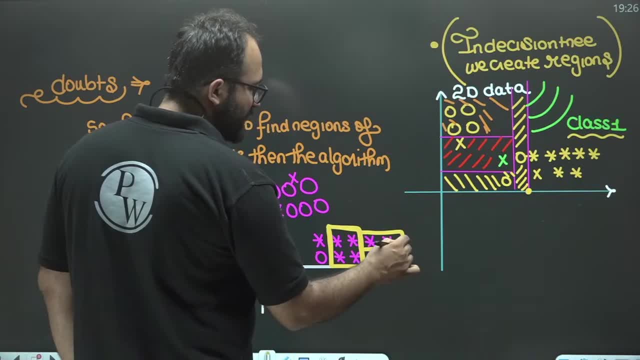 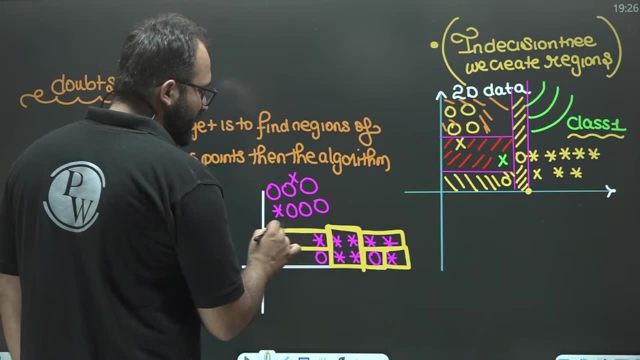 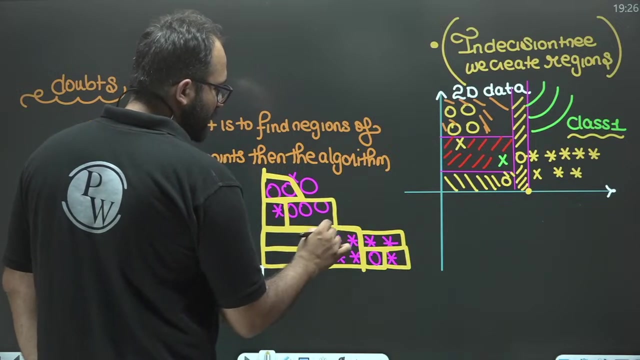 we will make this region of class one. the region in the middle will be of class zero. then it will be reverse of class one. similarly, it will say this whole region, because we can only make rectangular region. this whole depth, This region is of class 0, this is of class 1, then this is of class 0, this is of class 0. in this way and we can make it like this: 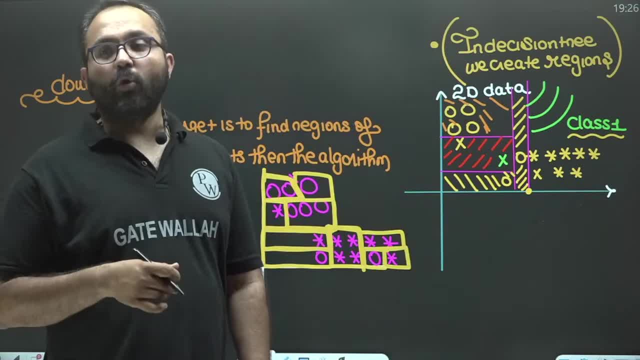 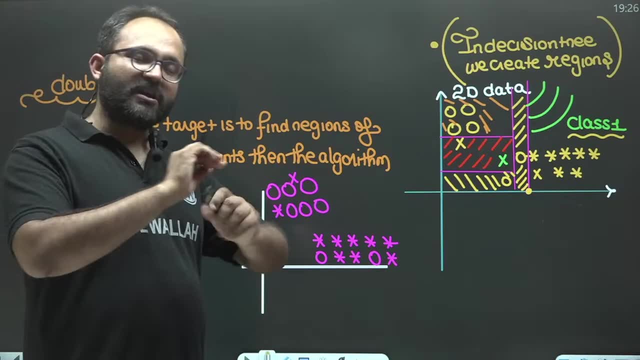 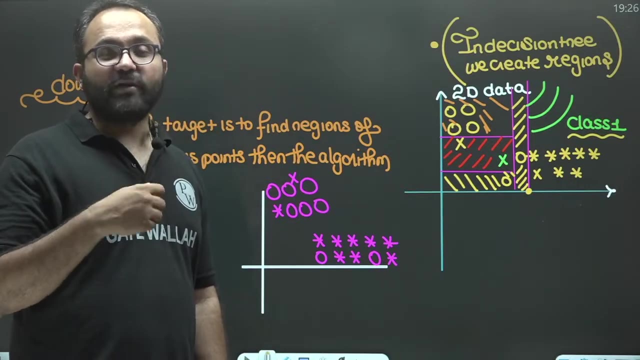 So here, in this whole scenario, our algorithm will try to over-fitting If we just follow the same rule that we need such a region, keep breaking, I don't mean anything, keep running and we just need homogeneous region or homogeneous point region. 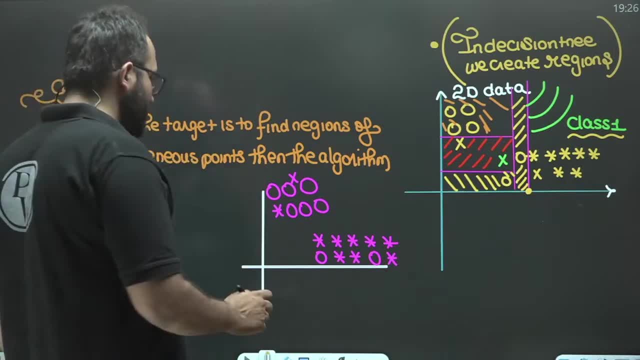 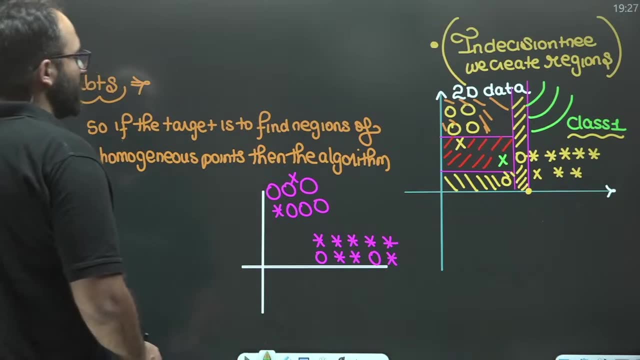 Then you will say that this is wrong algorithm, because here our algorithm will over-fit the whole data. Who all understood this thing? So if the target is to find the region of the homogeneous point, then the algorithm will surely lead to over-fitting, Our algorithm will over-fit, and this is obviously wrong. 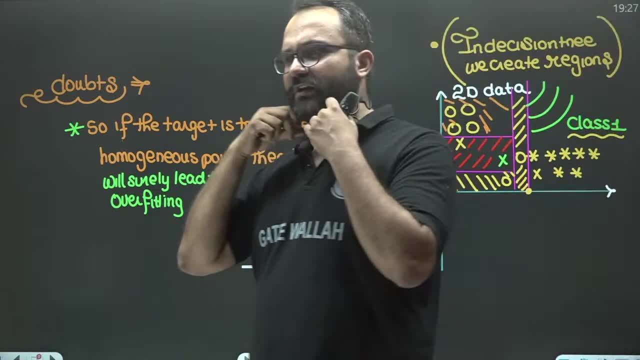 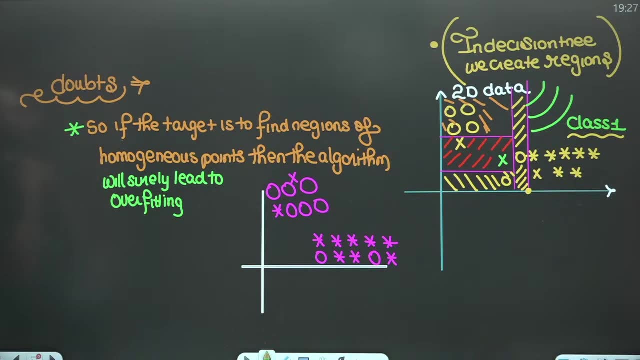 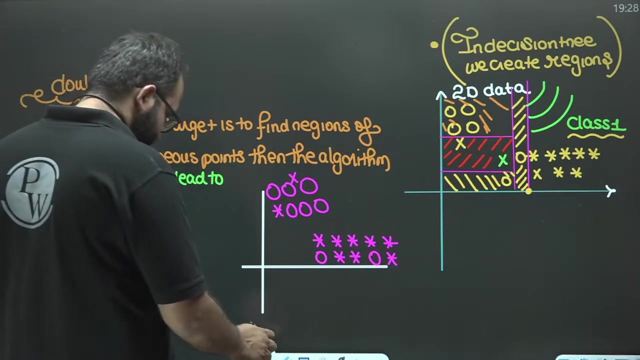 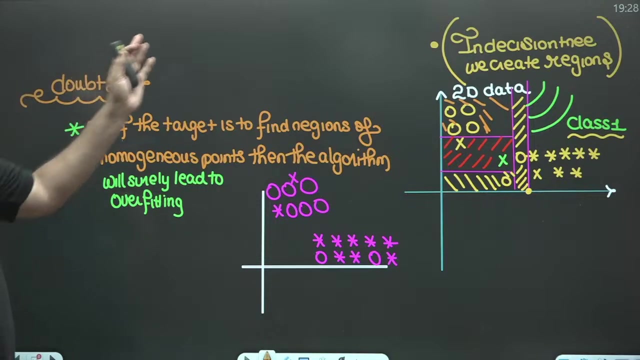 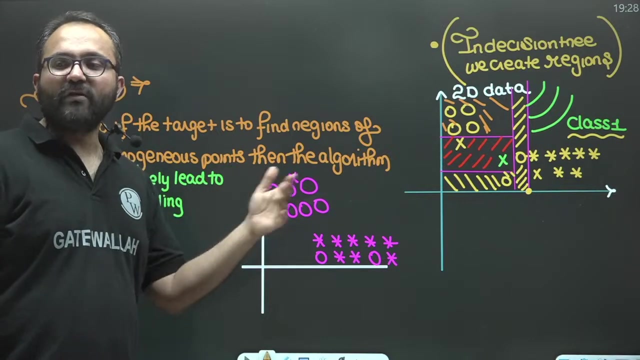 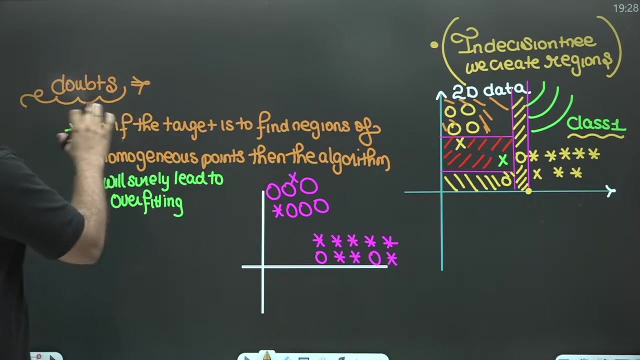 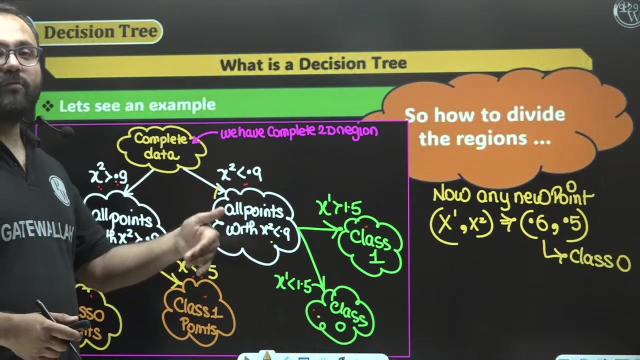 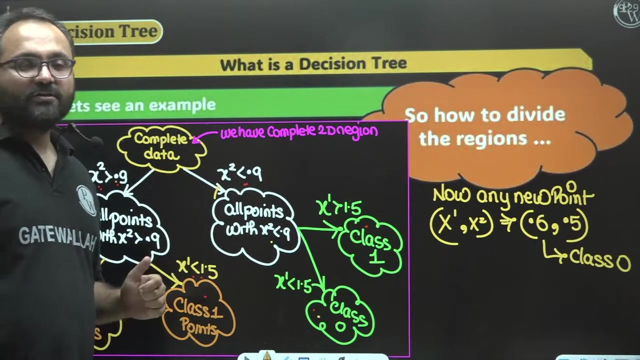 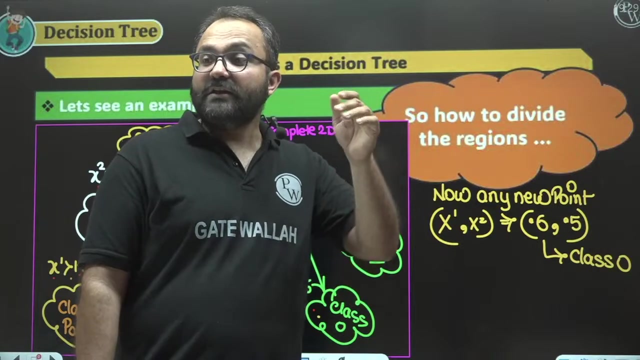 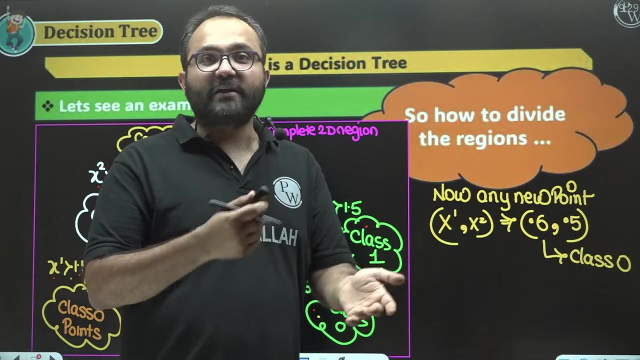 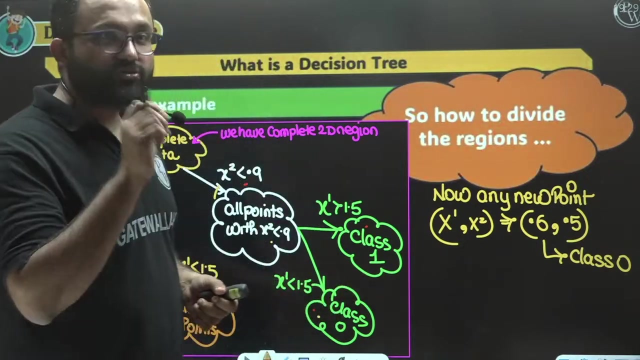 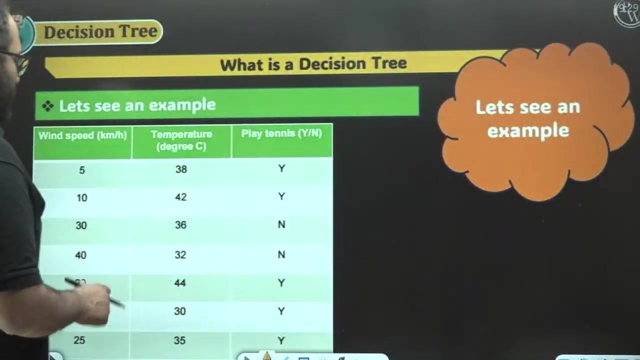 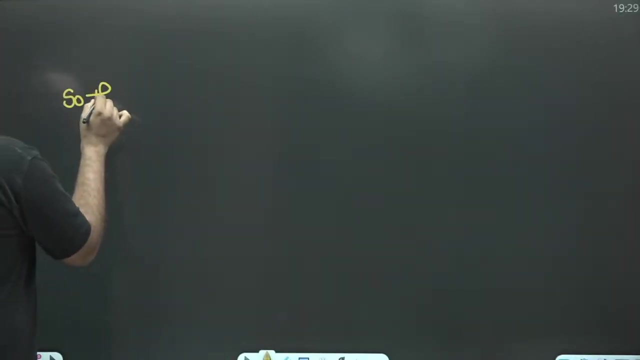 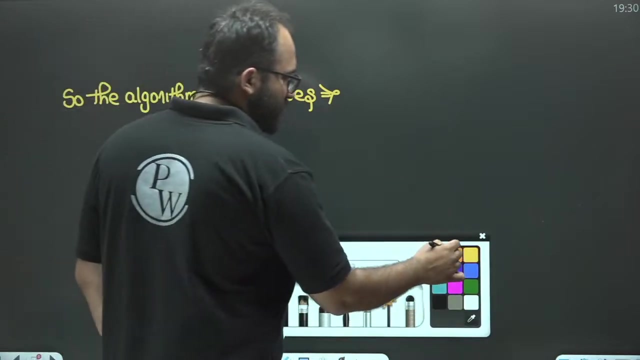 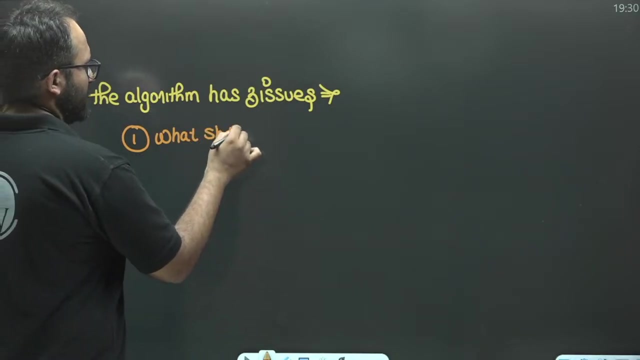 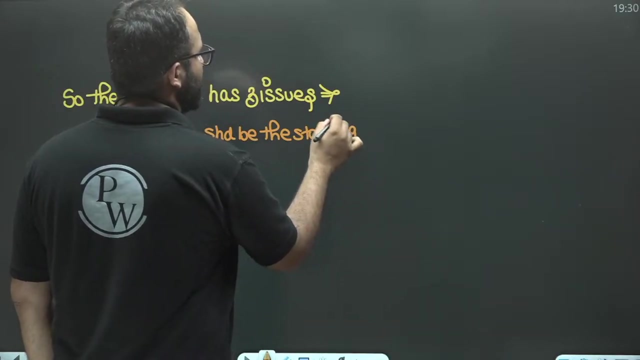 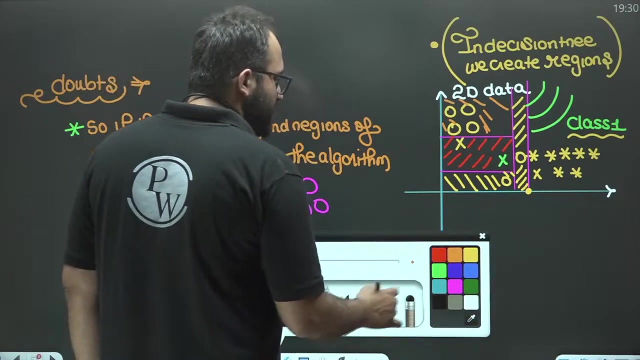 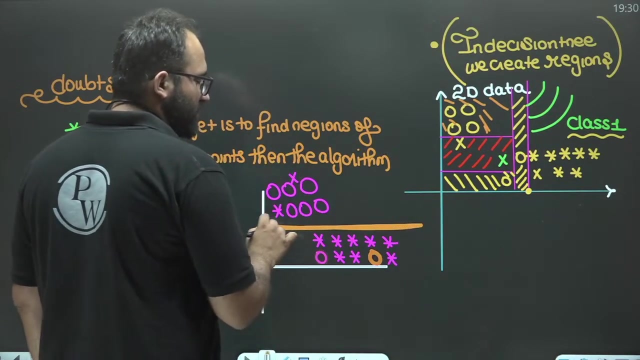 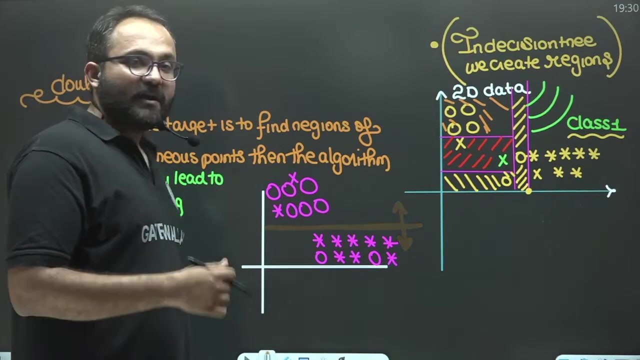 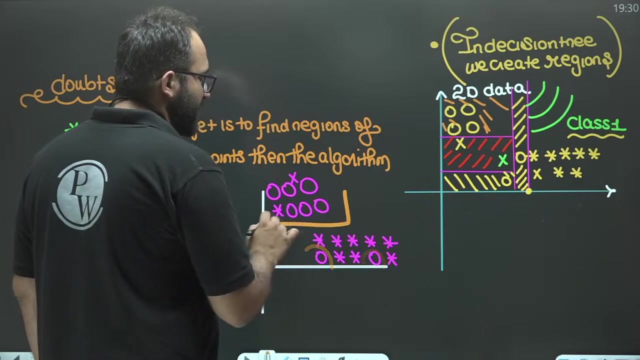 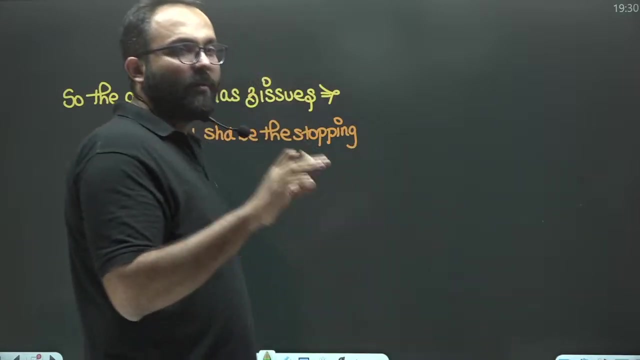 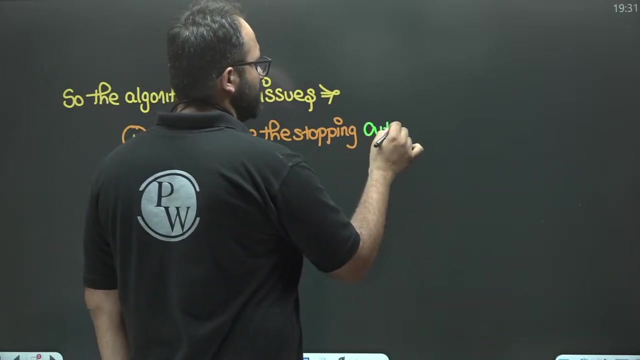 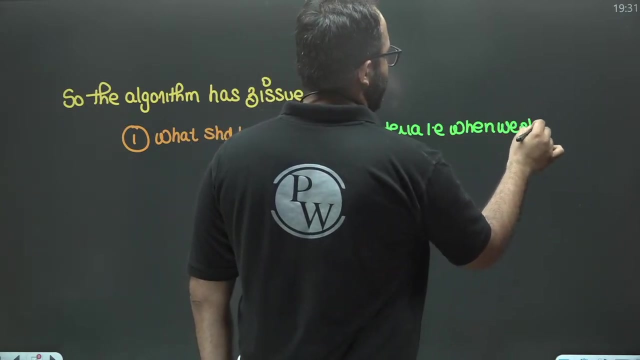 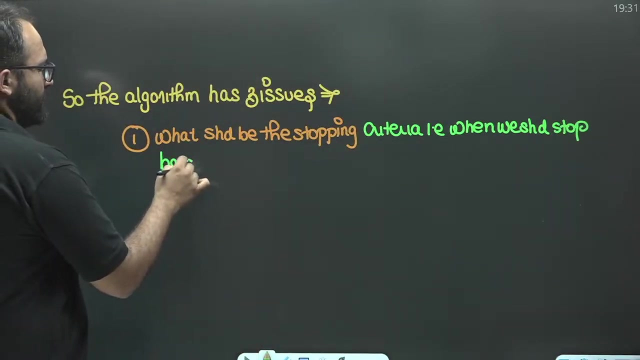 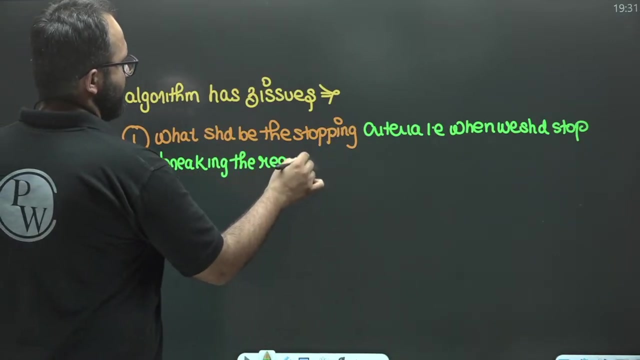 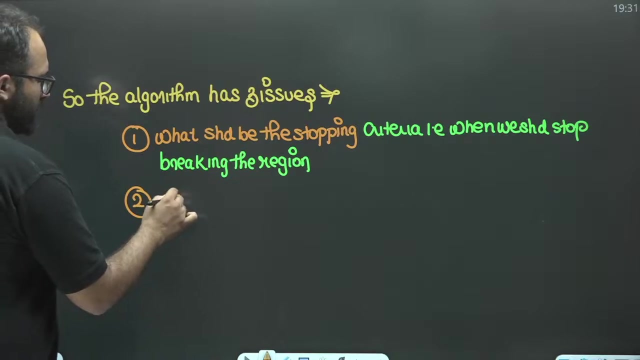 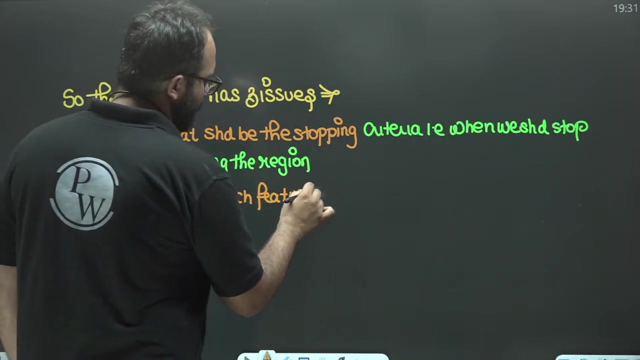 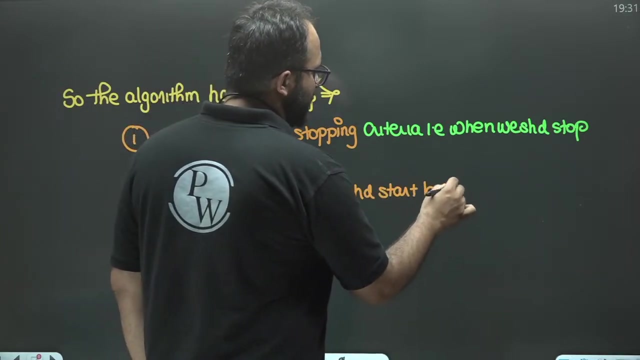 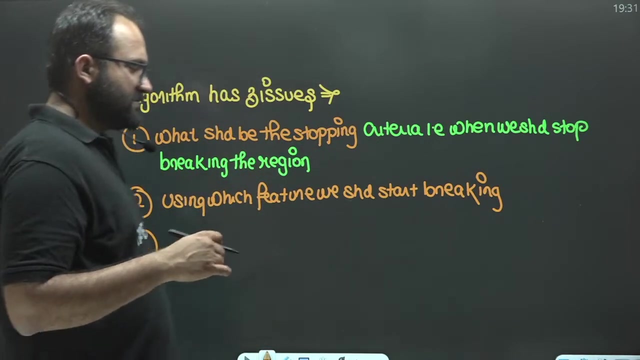 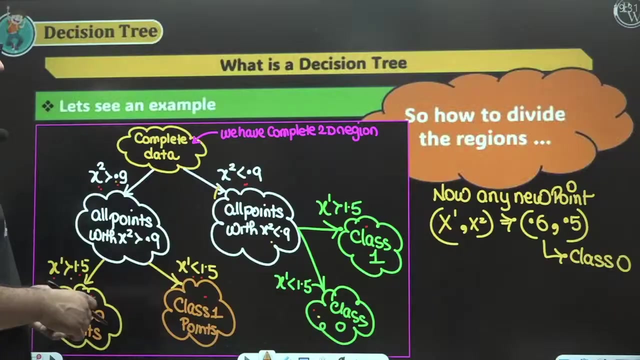 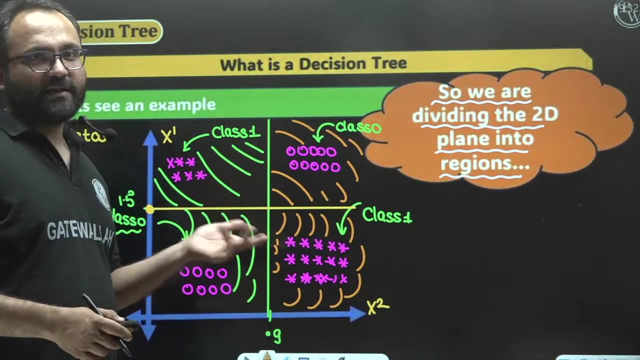 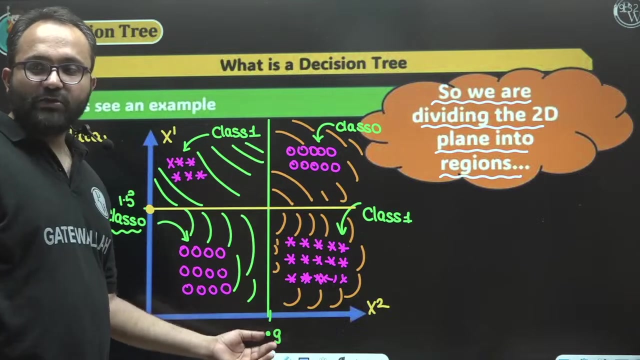 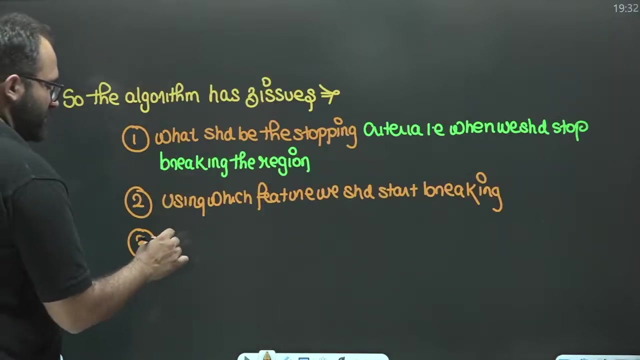 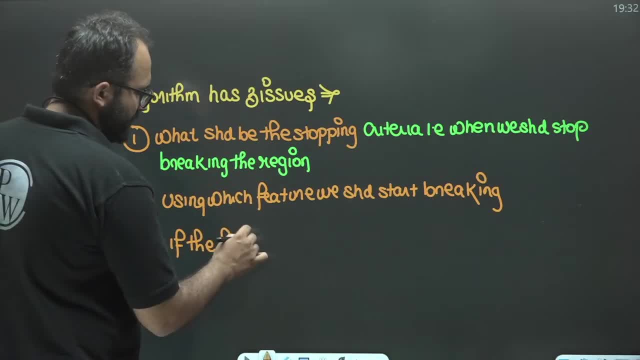 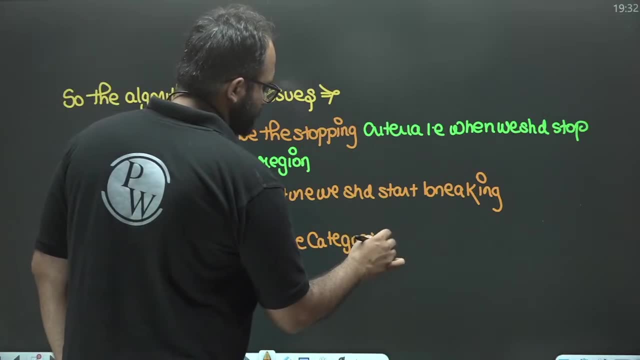 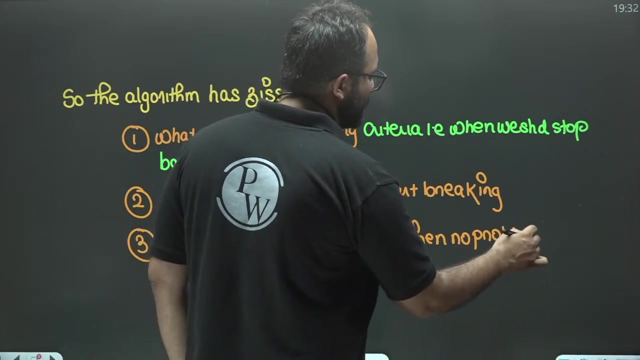 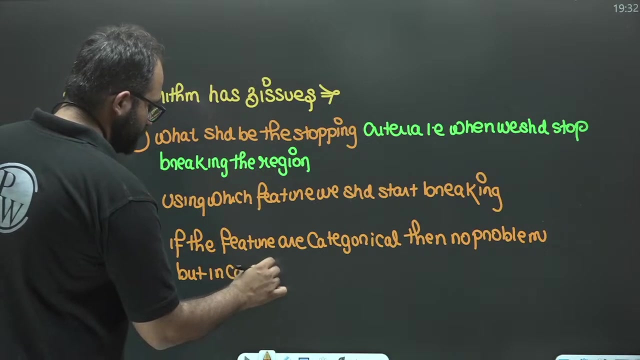 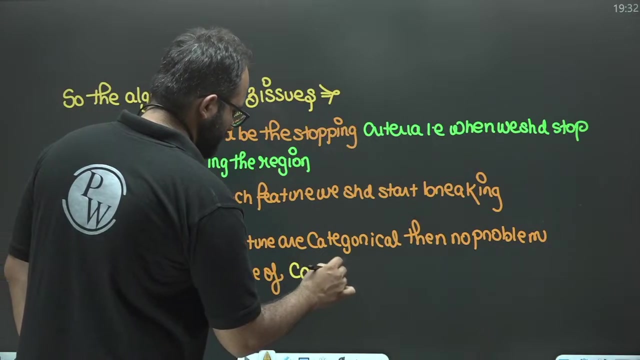 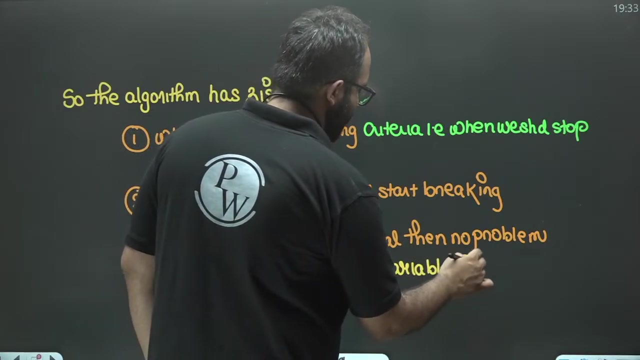 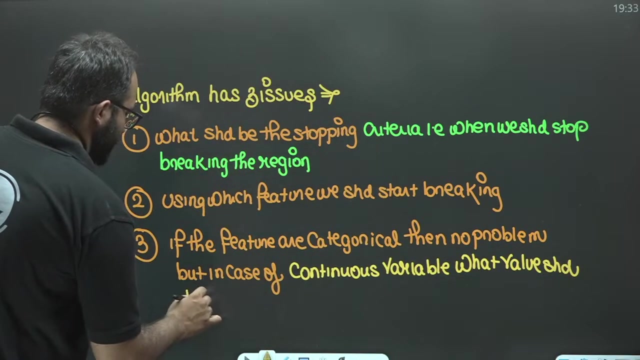 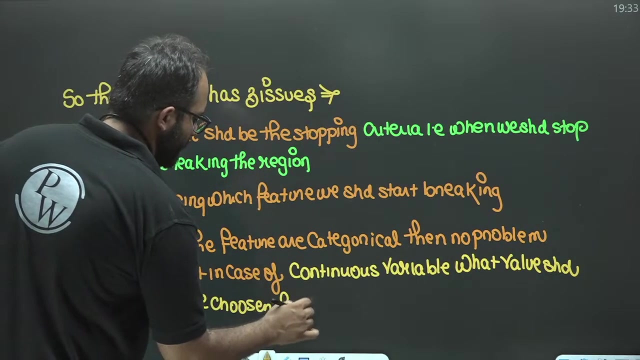 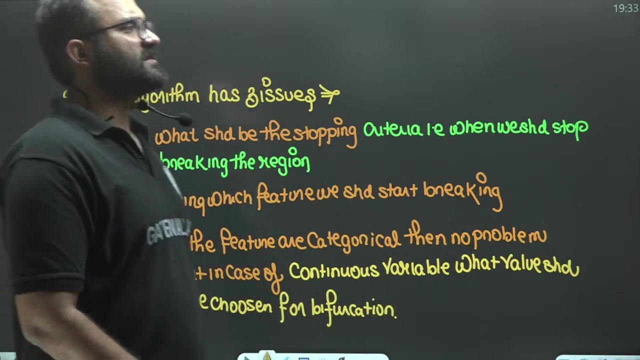 If the features are categorical, then no problem. but in case of Continuous variables, what value should be chosen for breaking? What value should be chosen for breaking or bifurcation? Which value should we choose for bifurcation? Which value is best? So we have to understand all these things. 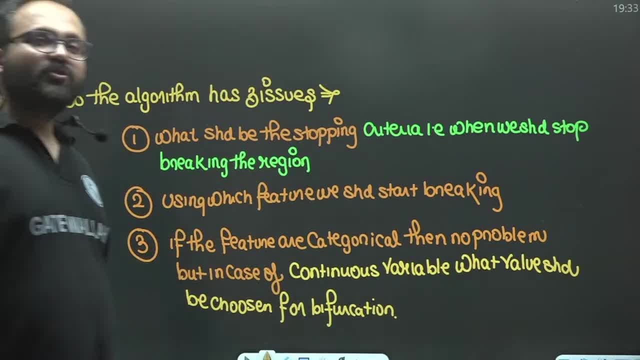 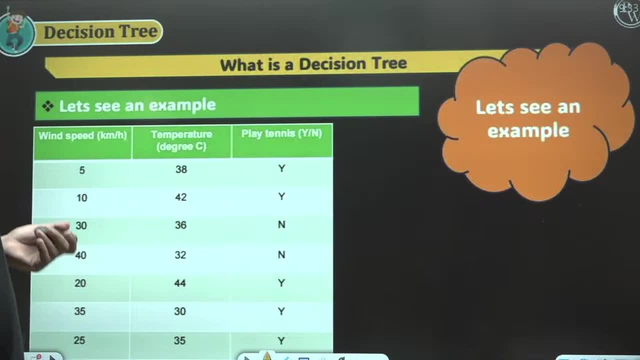 If you understand these three things, then you will be able to solve the numerical of the decision tree. So let's move ahead. friends, let's assume this is an example. So now, how will we do it? We have so many points: 5,, 30,, 10,, 42,, 30,, 36,, 40,, 42. 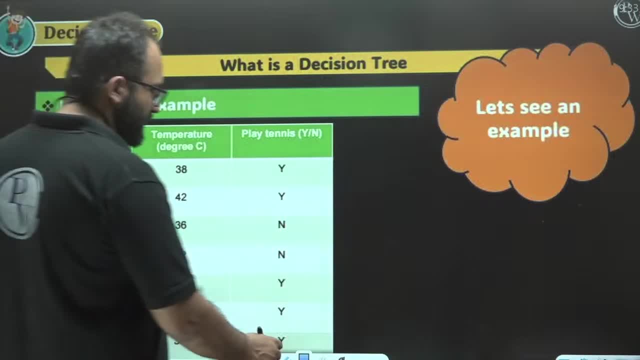 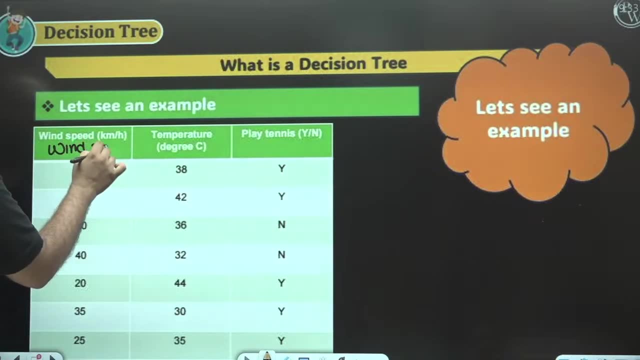 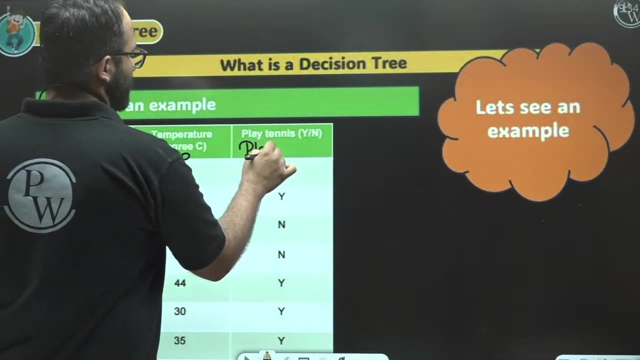 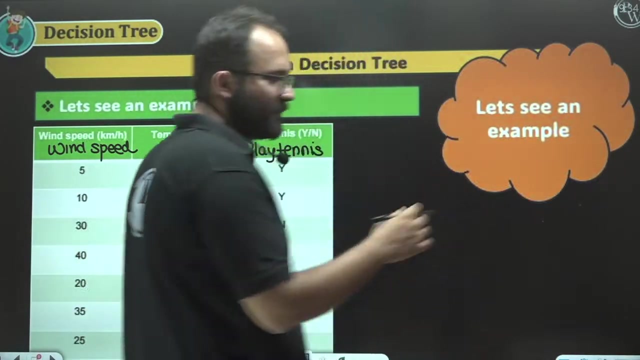 It has given us wind speed and temperature, and play tennis or not is written here. So here is wind speed, Here is temperature, Here is play tennis, yes or no? Will we play tennis or not? It is written here Now you can see if you want. you can draw it if you want. 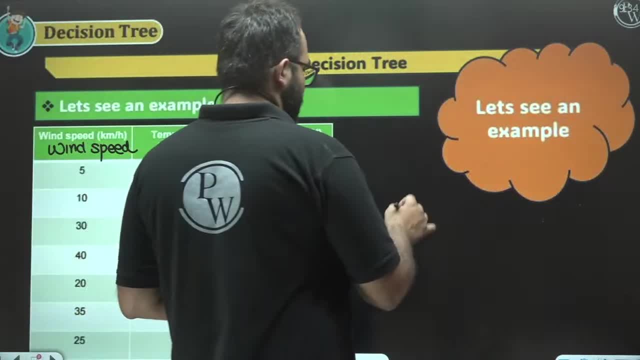 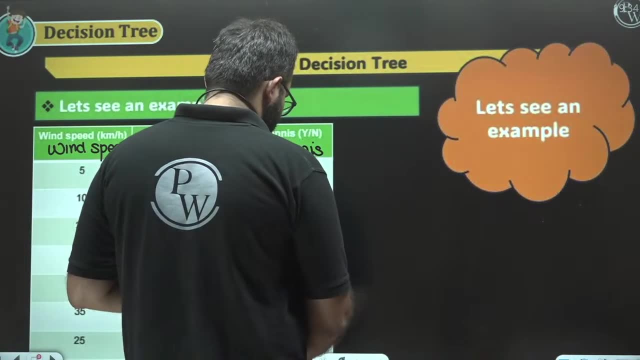 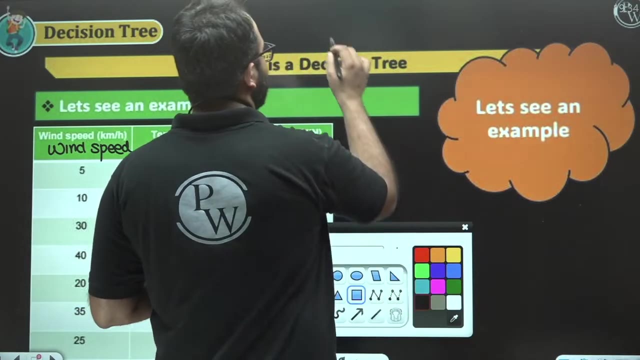 Or you can bifurcate it like this: If you want, you can draw here too, But I don't think there is a need to draw, So we start with the complete data. I will remove this in front of you So that we can do it very easily. 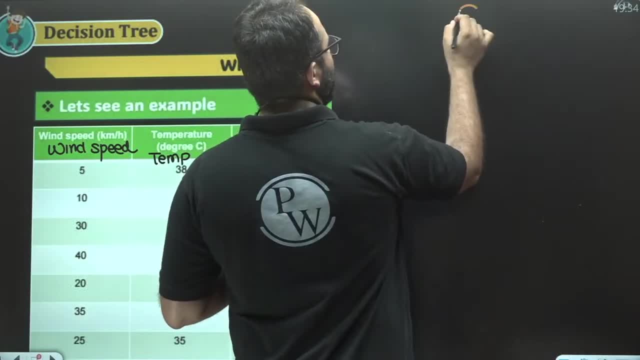 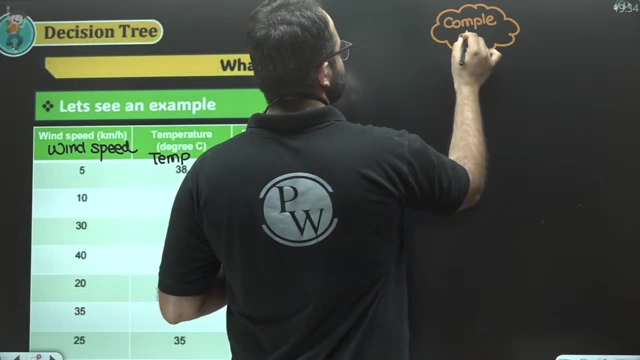 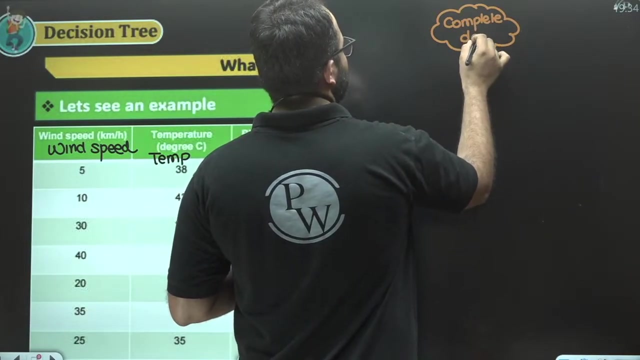 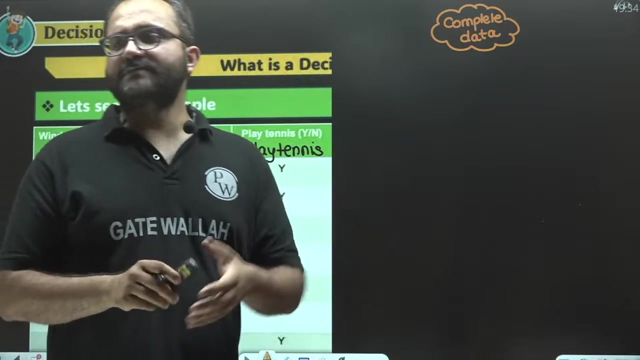 See, So we start with a point where there is complete data. So we have the complete data in this box. Okay, There will be two things here: That now we have two variables, x1 and x2. So which one to break? Now I am selecting randomly, But in the future we will see which variable is best. 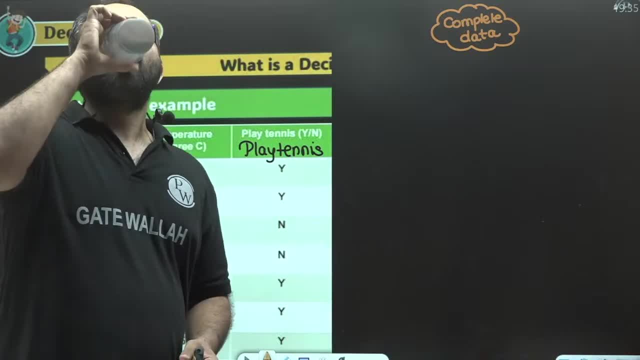 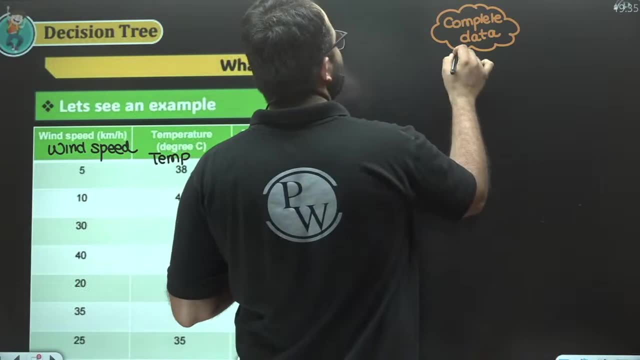 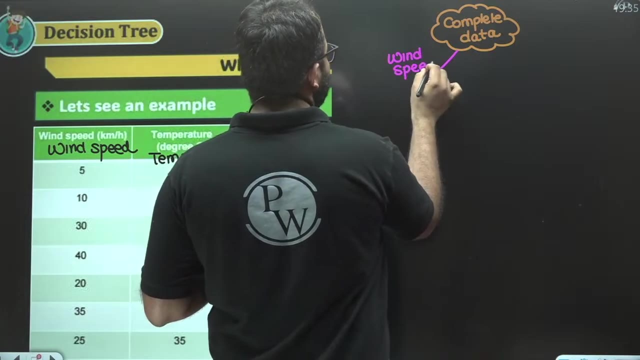 Still, we have some rules Which we will see in the next class. But now I am choosing randomly, I am just choosing any one. Or assume wind speed. Now you will say, Sir, why didn't you bifurcate with temperature, Brother, we could have done it with that too. 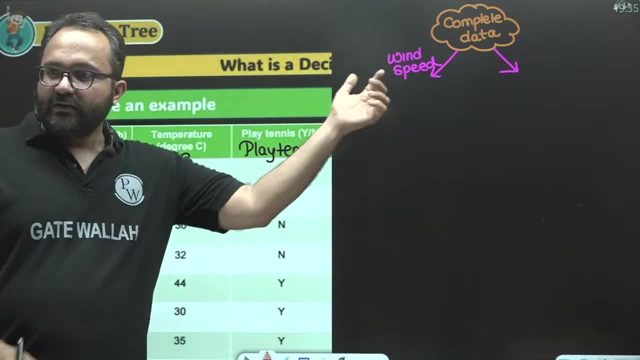 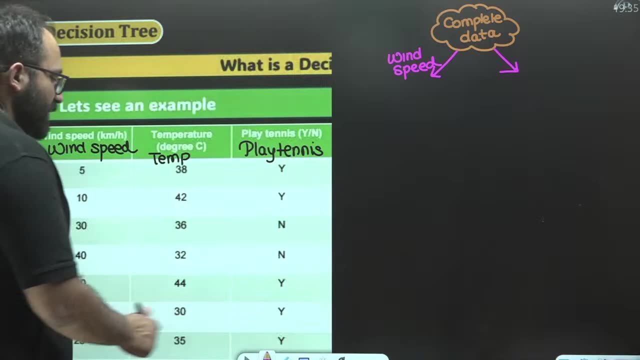 Okay, And this kind of question can come in the gate exam- That we should bifurcate at wind speed Or at temperature, And you tell me So. now you see friends Here, you will be able to see things very easily Here. 5 is yes. 10 is yes. 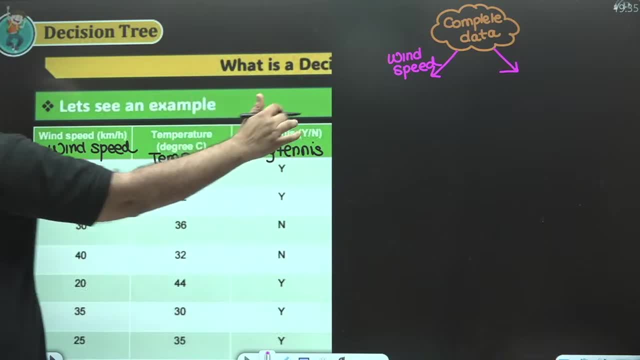 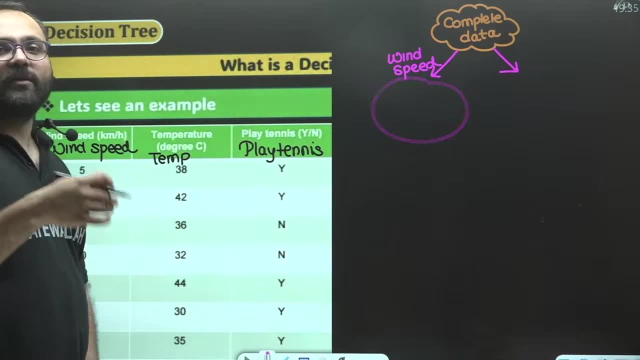 We want homogeneous points, Okay. We want homogeneous points in the region made here, Okay. Homogeneous means We want points of one category. So here, 5 is, 10 is In the case of yes, 20 is, 35 is And 25 is Okay. 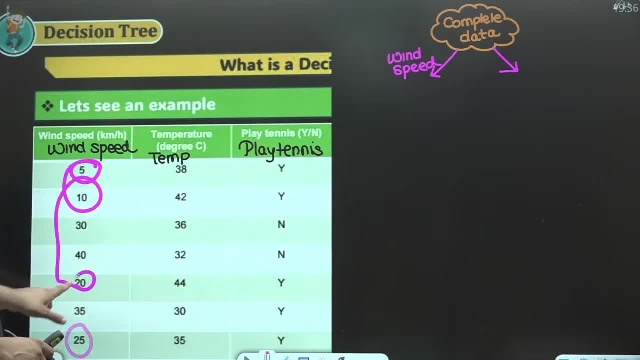 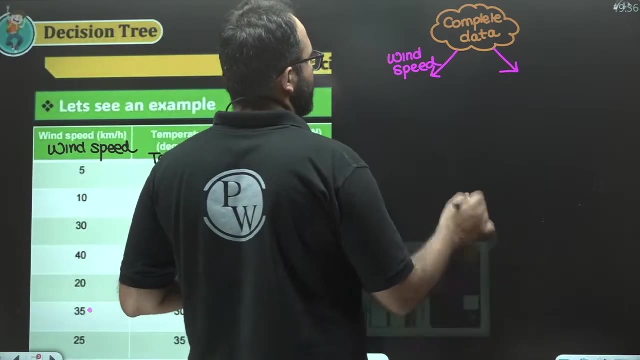 5, 10, 25, 35 And 25. Okay, Now, here you can see: 30 has 9 and 40 also has 9, But 35 has yes. So what can be the best thing That you can do, Sir? here we will bifurcate. 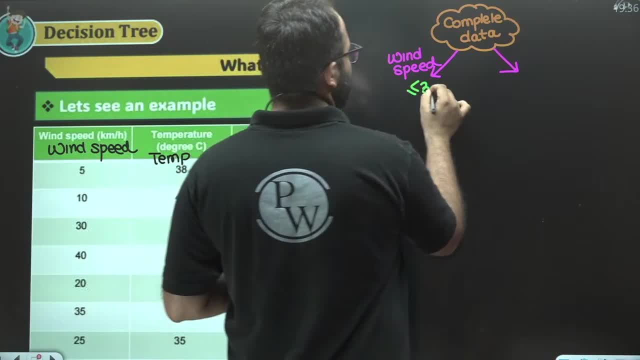 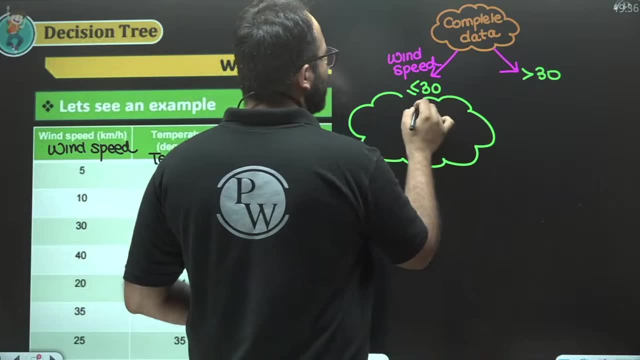 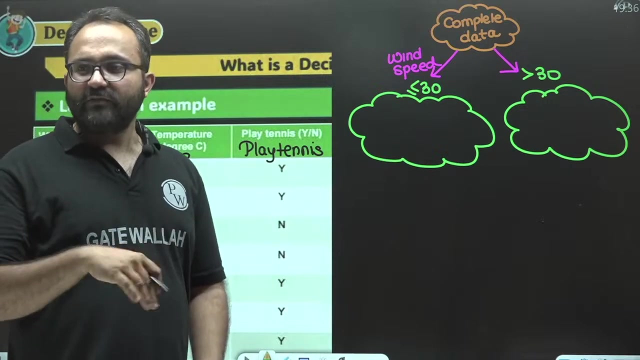 Wind speed Less than equal to 30 Or greater than equal to Or greater than 30. In this way, we will bifurcate it. Why did you take 30?? Now, don't worry, It will give you in the paper. It will be written in the question paper. 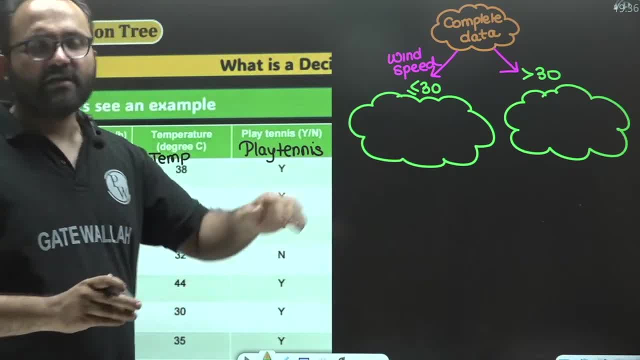 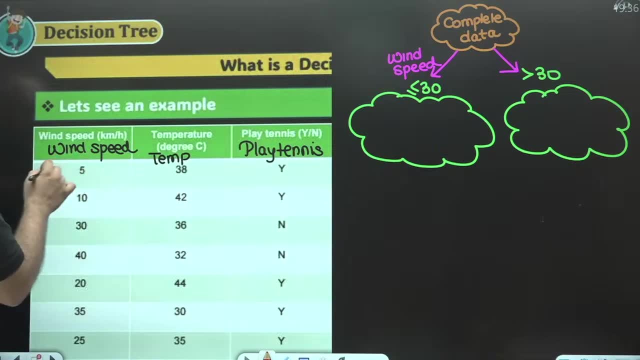 Where we have to bifurcate And then we have to find what is the best bifurcation. I am just taking it randomly: In the case of less than 30, You can see here 0.1, 0.2, 0.3. So in the case of less than equal to 30. 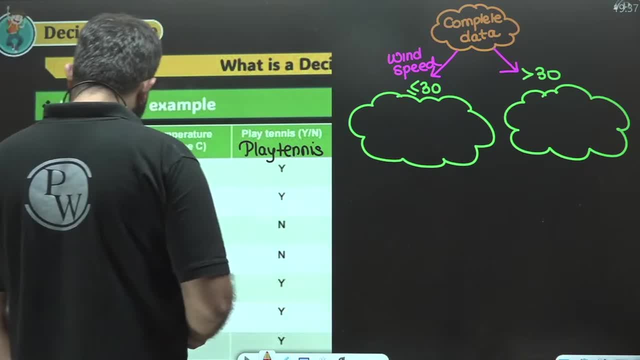 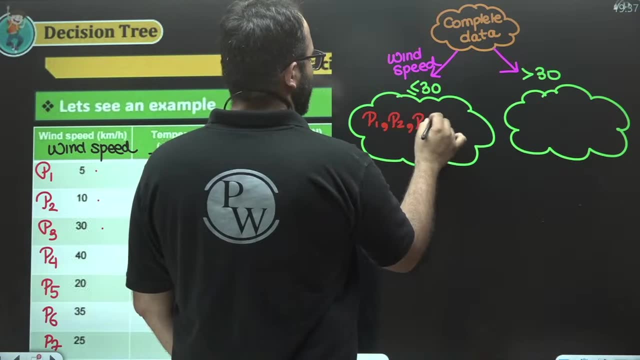 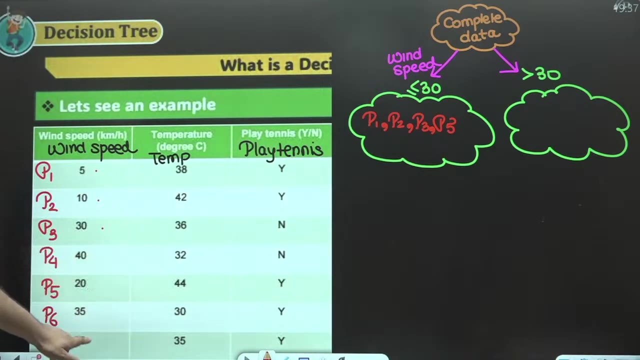 0.1, 2 and 3, 5 will come. Okay, So 0.1, 0.2, 0.3 and 0.5. 0.1,, 2,, 3 and 5- These will come, And 4,, 6 and 7. 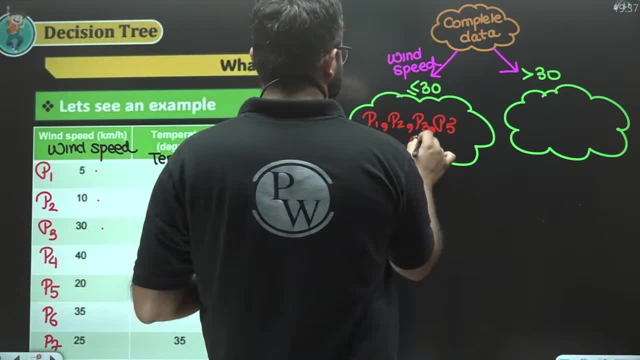 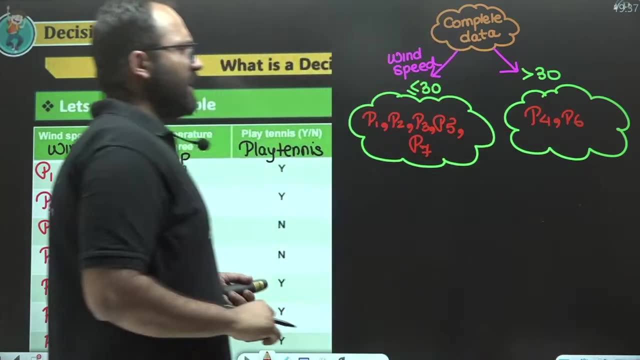 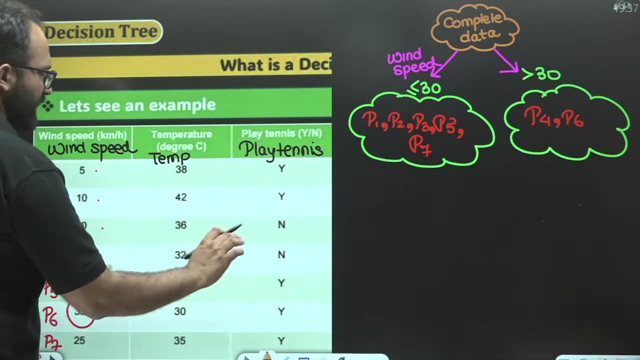 Will go there. No 7 will also come here. So just 0.4 and 0.6 Will go here Now. see 4 and 6. So 4 Still has no, But 6 has yes. So now we will have to bifurcate in that case. 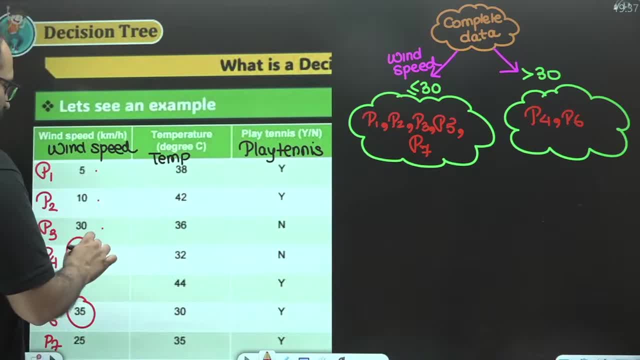 So that we can get homogeneous points. You can see: 4 has no And 6 has yes. So now we have to bifurcate more. Now, where can we bifurcate Wind speed bifurcation? Now we will bifurcate at temperature. So here you can see very easily. 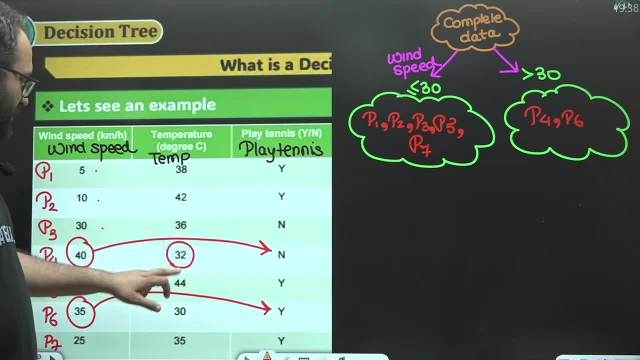 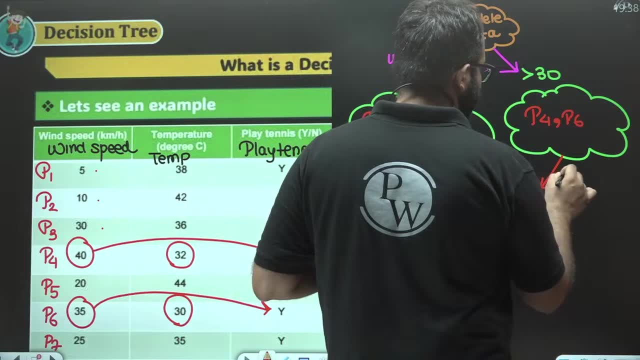 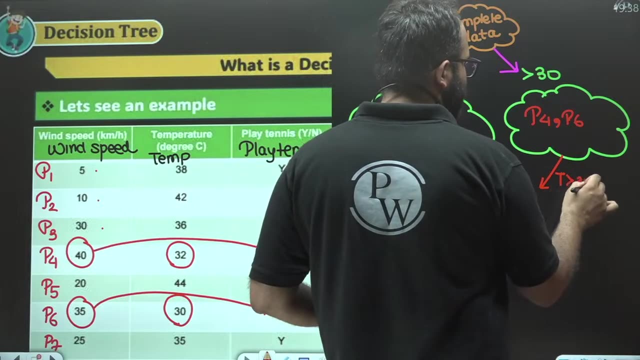 That Here temperature is 32 And here temperature is 30. So how will bifurcation be? Temperature greater than equal to 30. Sorry, Temperature greater than 30 And temperature less than equal to 30 And temperature less than equal to 30. So you will see here. 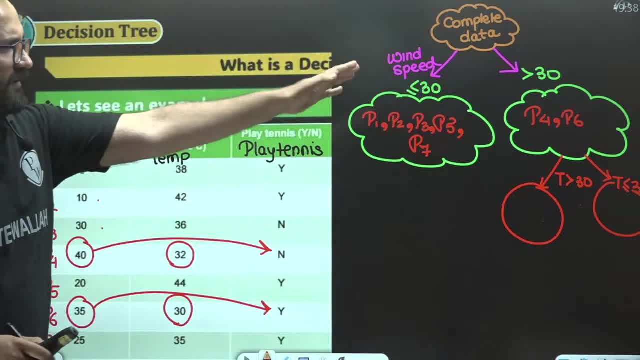 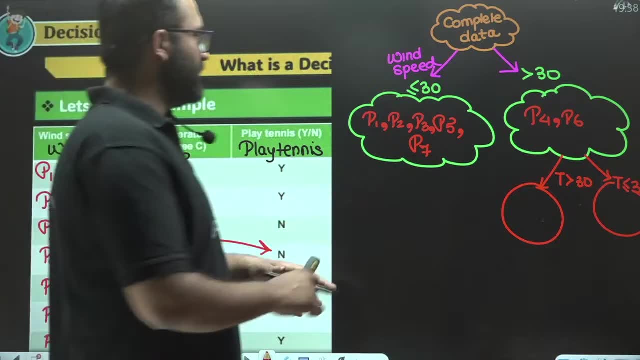 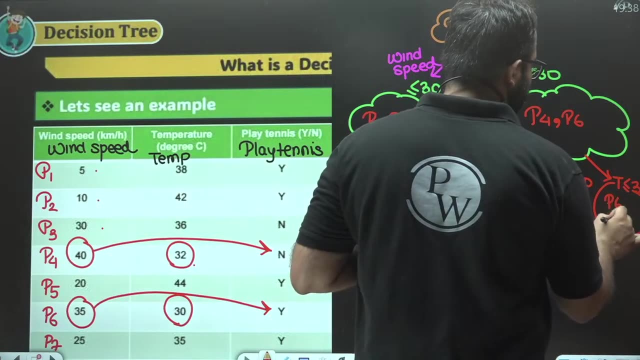 Which points will come here. So if we bifurcate that box Temperature greater than 30, So P4 will be separated, P4 will come here And this category will be No class And P6 will come here. This category will be yes class. Similarly, friends, We can bifurcate here. 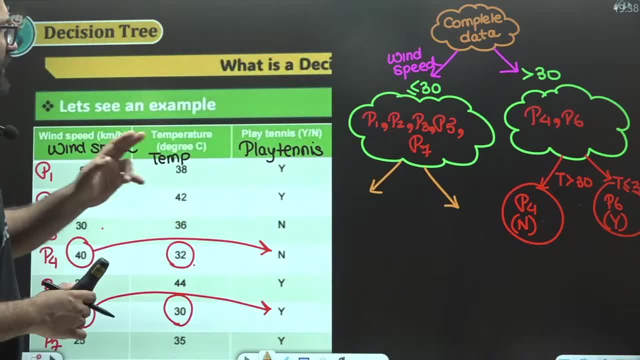 You can see P1,, 2,, 3, 5, 7. P1 Is yes, P2 is yes, P3 is no. This is of different category. P5 is yes, P7 Is yes, Rest all are yes, But P3 is doing some drama. 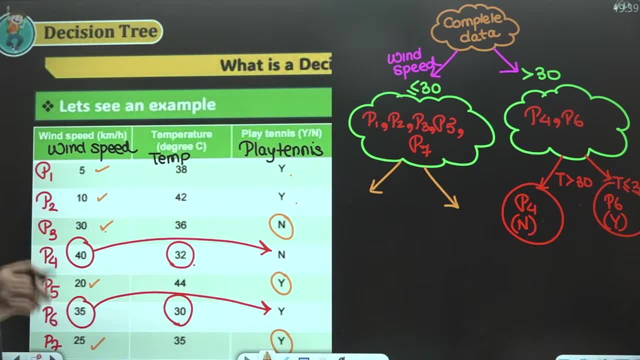 No is coming. Ok, Now what region we will try to create. So you will say, sir, Here temperature is 36, 38,, 42, 44 and 35. Now, here some problem is happening. Means How to bifurcate here, friends, Here bifurcation, if we want. 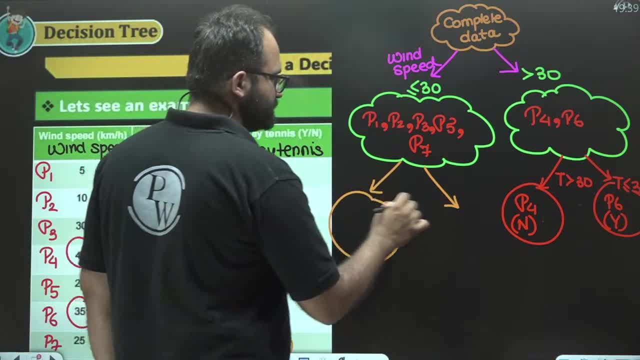 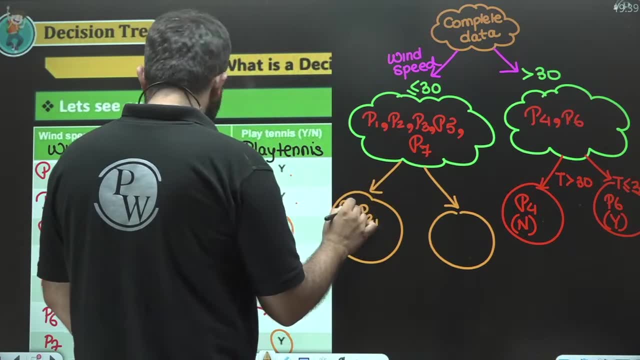 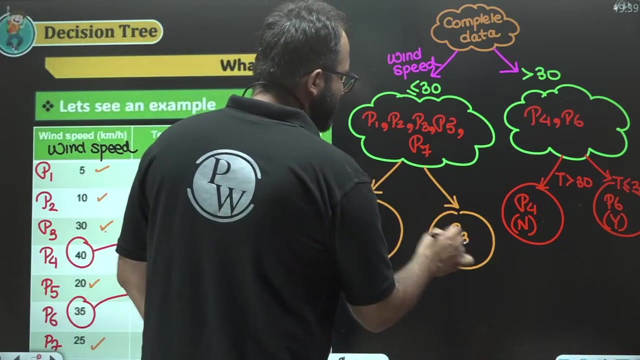 To make homogeneous points, To make homogeneous region. So here you want To come point of P1, Come point of P2, Come point of P3, Come point of P5, Come point of P7. These are all yes, class points, And we want P3 to come here. 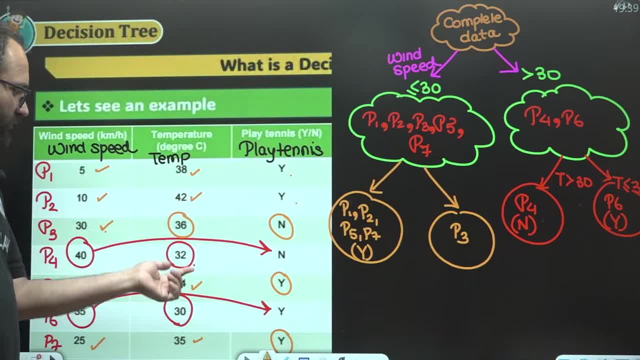 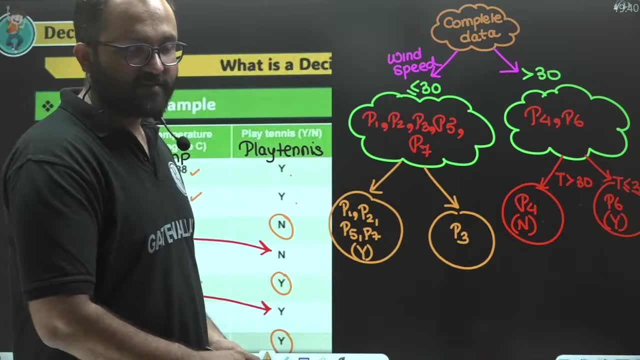 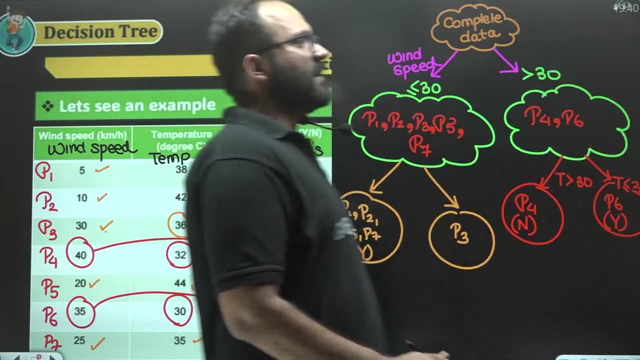 P3 means Temperature 36, But 38,, 42,, 44 and 35- All these temperatures Should come in left side group And 36 temperature should come here. So what do you think? How will bifurcation happen? How will bifurcation happen? 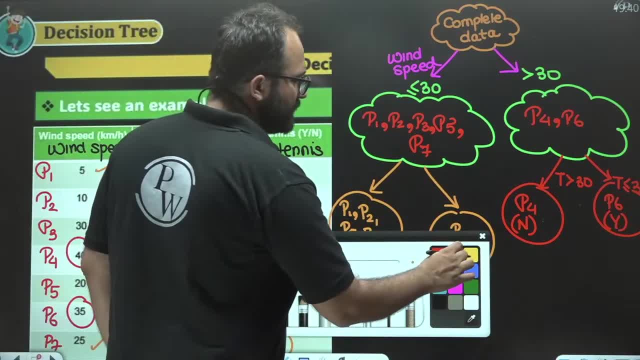 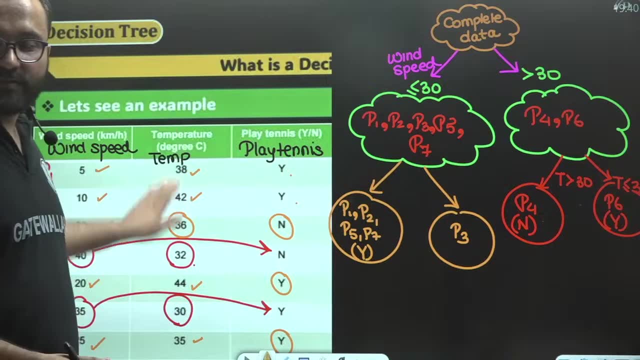 So here we can do bifurcation Anyhow. There are many ways, But you think We are trying to do over fitting. We are trying to learn this data Because now see 38,, 42,, 35 and 44 Is yes and 36 is no. 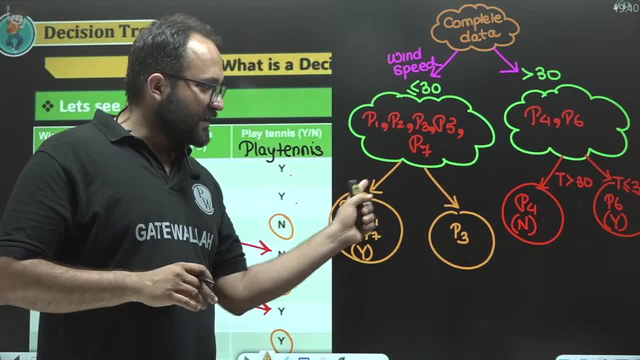 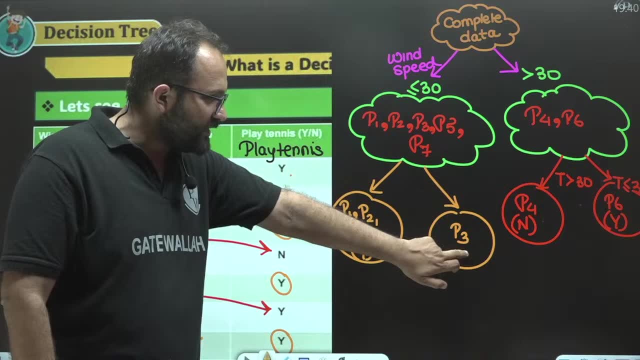 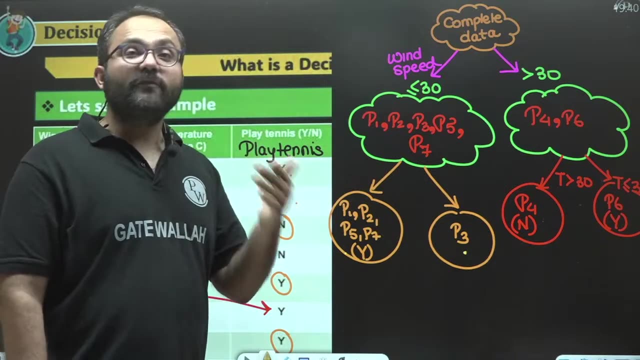 So now we want to take such Decision Or want to create such a boundary, Or want to bifurcate like this, That only 36 point Come here. All these points should come here, And obviously this is actually What do we call it: Over fitting the data. So 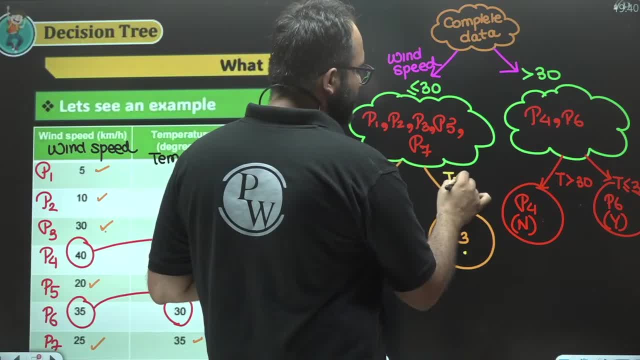 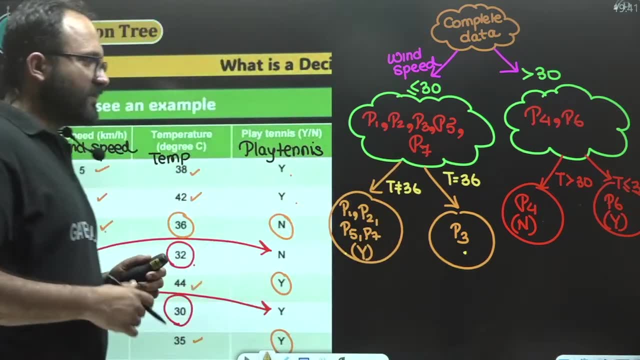 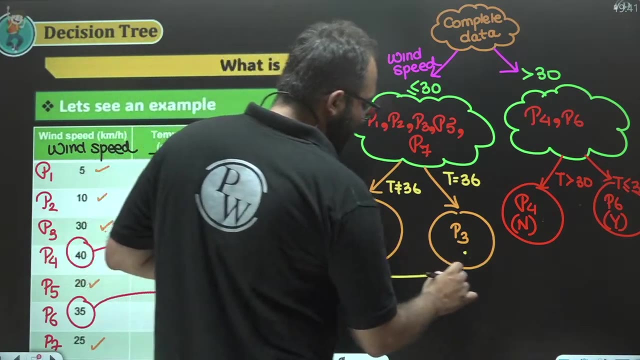 Now we are talking about over fitting. If temperature comes to 36, Then go here, And temperature not equals to 36, Then go here. In this way, we can bifurcate it, But this is a clear case of What do we call it Over fitting. This is a clear case of over fitting. 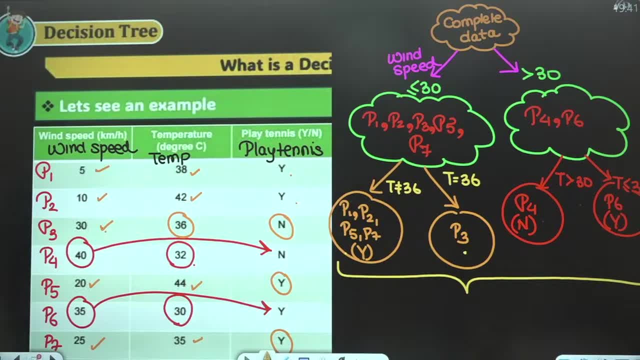 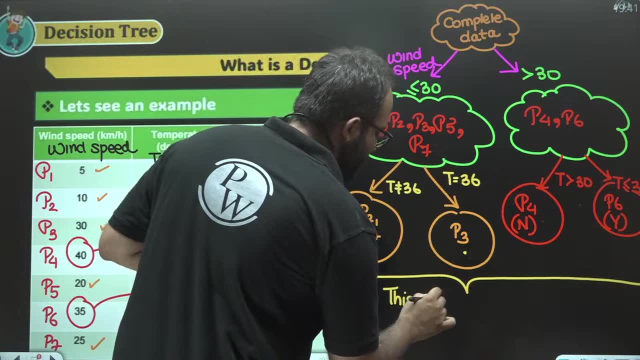 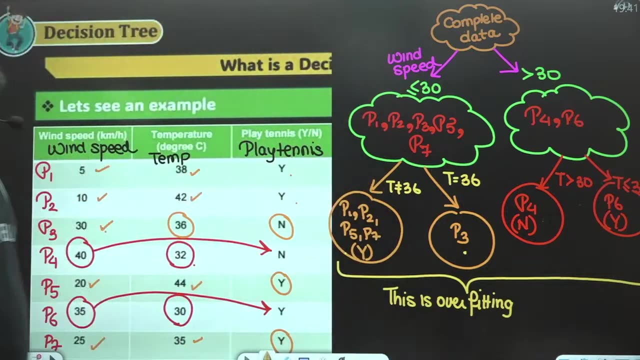 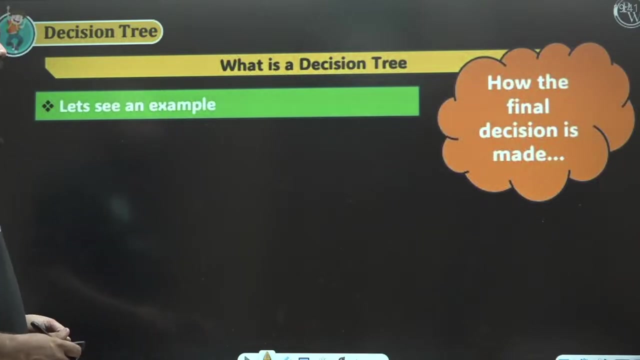 In this way, we have done bifurcation. Ok, So this is over fitting. So, as I told you, If we keep doing bifurcation, Then over fitting will keep happening. The same thing we can see here. Come on, And Now here we will say That our bifurcation is done. 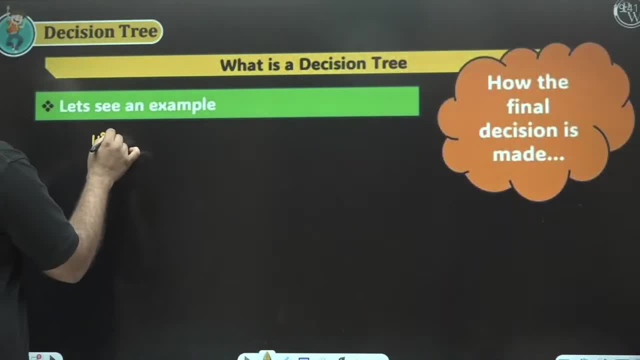 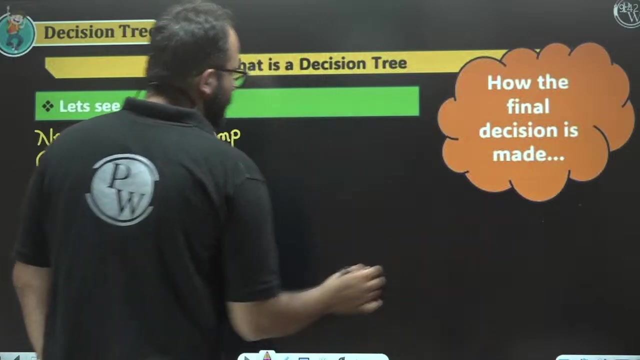 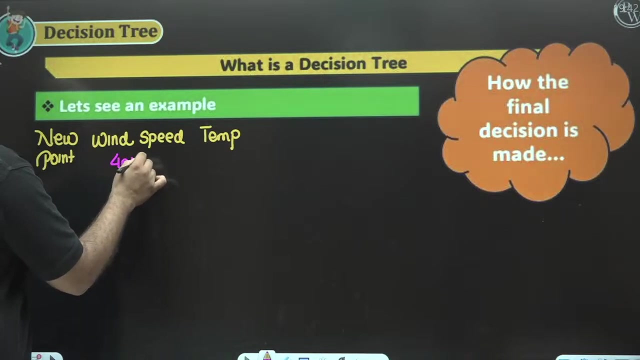 Now, if someone gives us a new point, For example someone says wind speed, This is our new point: Wind speed and temperature. So suppose Our wind speed- Let's say wind speed- is, Let's take anything in km per hour, Let's say 40 km per hour, And